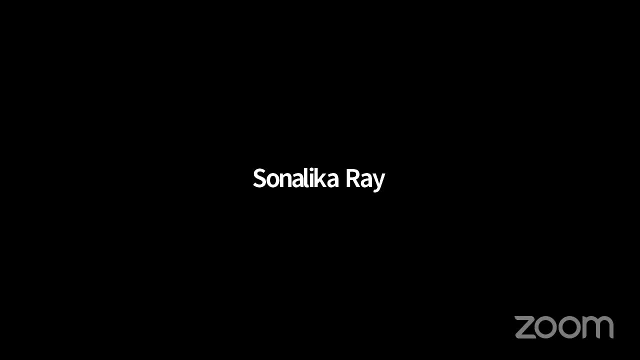 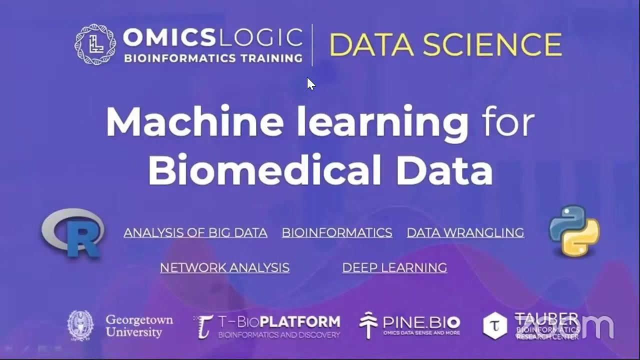 Thank you. If you are live on YouTube, I'll just share the link in the chat box. You can refer the link to see the recording after the session. Thank you, And by the time we begin with the session, it would be really great if you all could tell me what is your educational background. 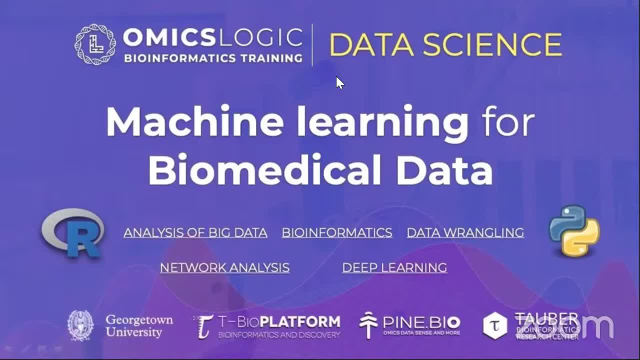 And also, what are your research interests. It would be great to know more about you all and also help us understand what exactly you are looking for, so that we could help you with the best. Hi Hamda So BSc in Biochemistry from which university? 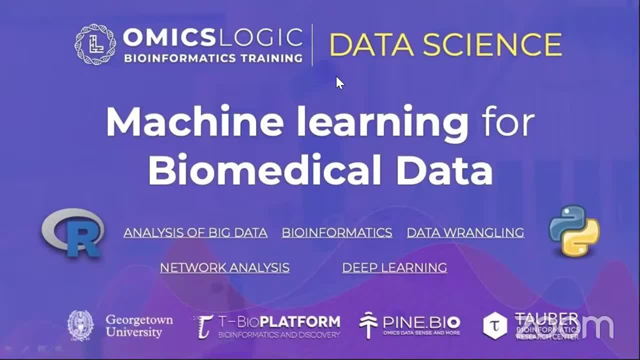 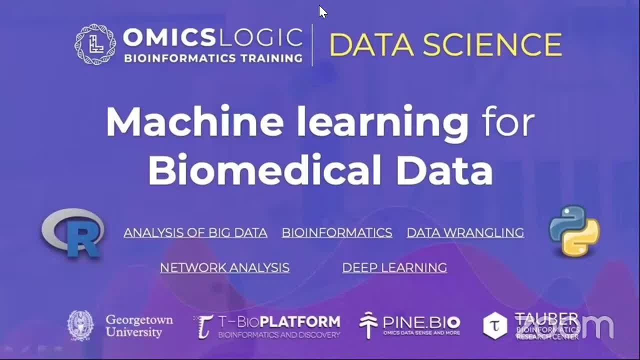 So data science is a desired profession that brings together diverse skills that are needed to handle data And turn it into useful information. Some of the highest paying and interesting jobs are for data scientists at high-tech companies like Apple, Google and Uber, and also the healthcare companies as well. 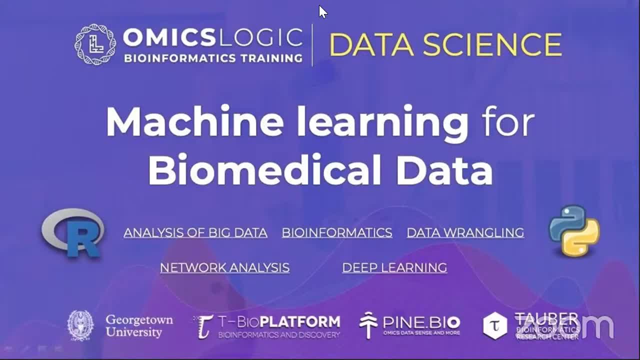 Areas of science where a tremendous amount of complex digital data is being generated are biotechnology and healthcare, And these industries are actually relying on scientific discoveries about biology and translating the basic understanding of biological processes into useful insights for drug discovery, improved treatment efficacy, as well as early detection of risks and even anticipation of disease progression. 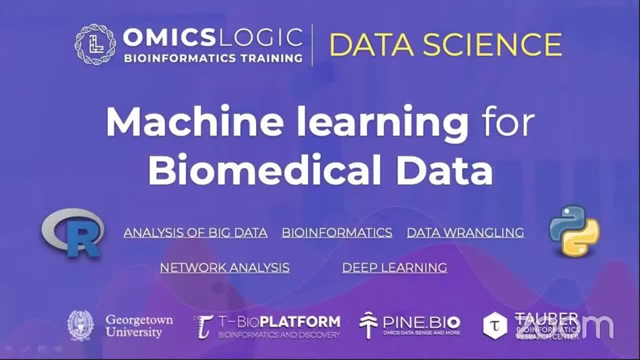 So in this course we will cover practical and conceptual aspects of machine learning in application And in addition to high throughput biomedical data, using various tools and R and Python. Throughout the course the students will get an understanding of opportunities and limitations, as well of machine learning in the context of preclinical and clinical research. 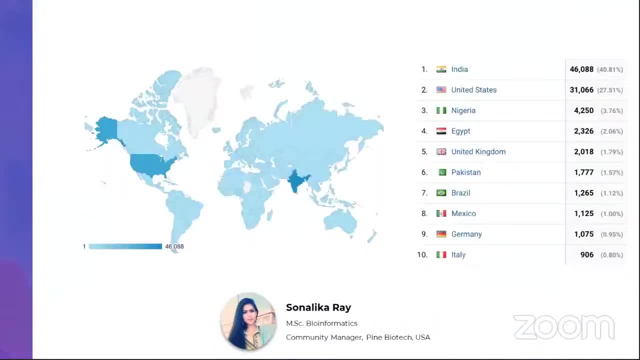 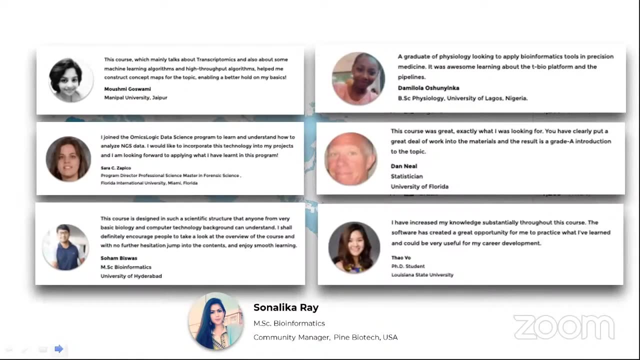 My name is Sunalika Ray and I'm the OmicsLogic community manager. I'm responsible for daily interaction with thousands of users that are a part of our bioinformatics community, which is a very important part of our community, And I'm also responsible for daily interaction with thousands of users that are a part of our bioinformatics community. 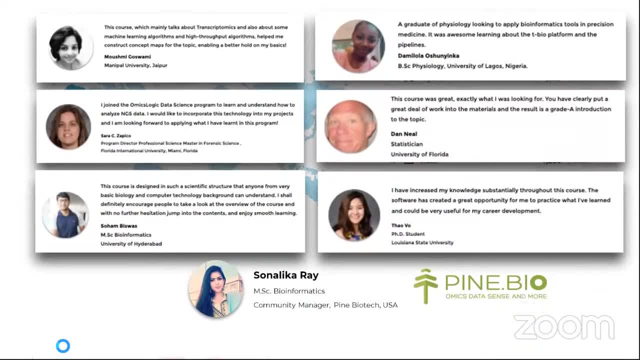 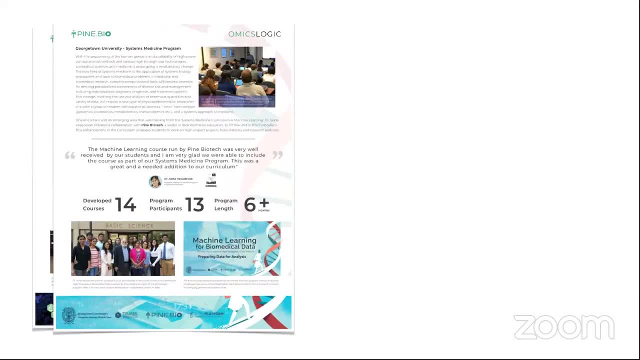 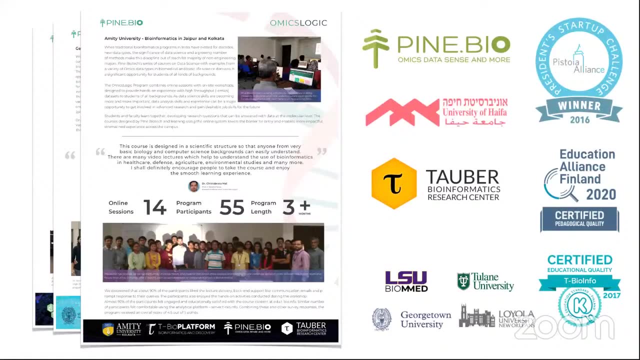 which is managed by PineBiotech. So, before we start with today's talk, I would like to introduce us. We are a US-based bioinformatics company who is working with multiple academic and commercial collaborators to develop easy-to-use analytical tools, And our mission is to make bioinformatics more accessible. 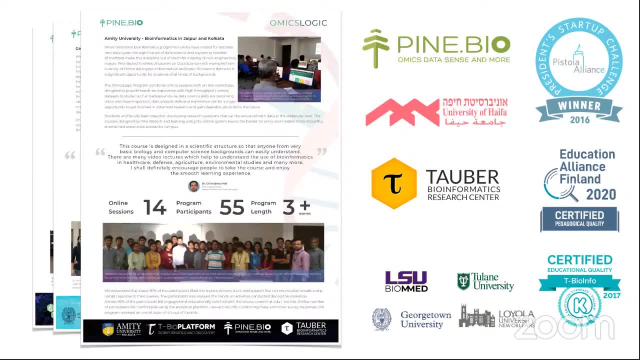 OmicsLogic research-based training programs are a result of close collaboration between PineBiotech and numerous academies, And through this collaboration, we are able to help students achieve high-quality education, which is the goal of our online training program. OmicsLogic is an international program that is running in 5 different regions. 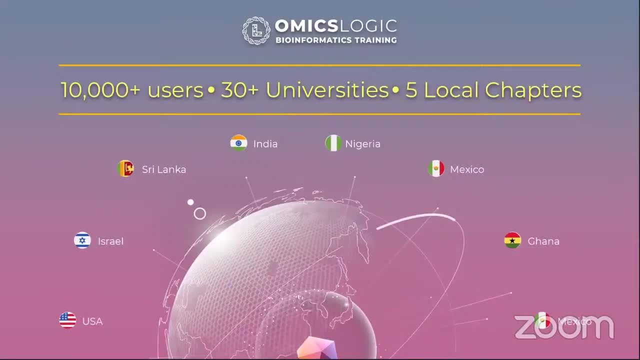 with over 10,000 users across the global hey wore, we will help more than 600 people grow within each industry around the world. Due to this fast growth, our team is working with local and regional coordinators that are helping refine local program logistics and 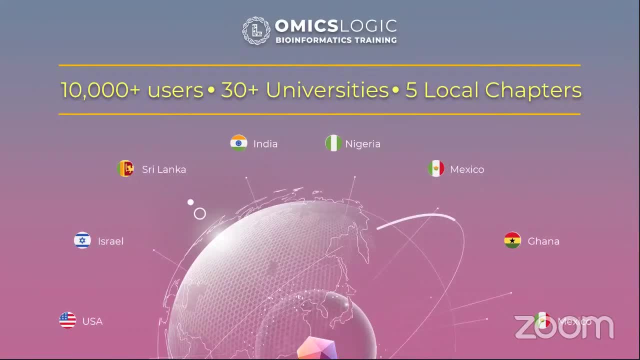 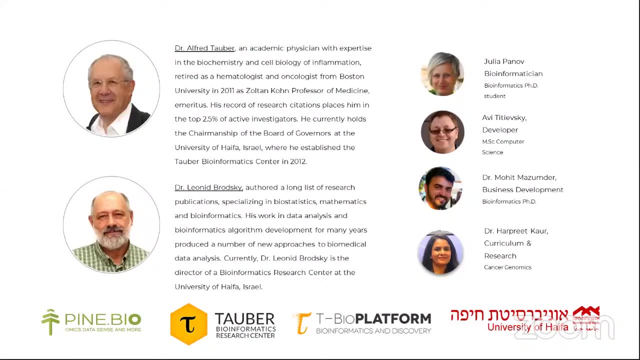 beste refers to discovering solutions to the problem of online training to Uma'S venir con los estudiantes and researchers around the world. I'm honored to have been working with a team that collectively has an amazing experience in this area, including the other co-founders of the company, Dr Alfred. 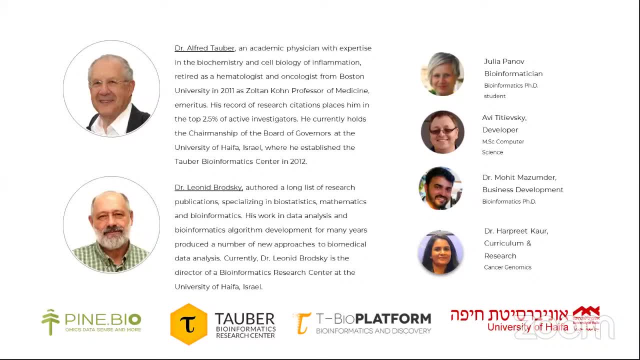 Tauber, who comes from a medical background with an expertise in oncology, immunology and biochemistry of inflammation, And one of his major projects is the establishment of the Tauber Bioinformatics Research Center, which has been at the core of what we do. 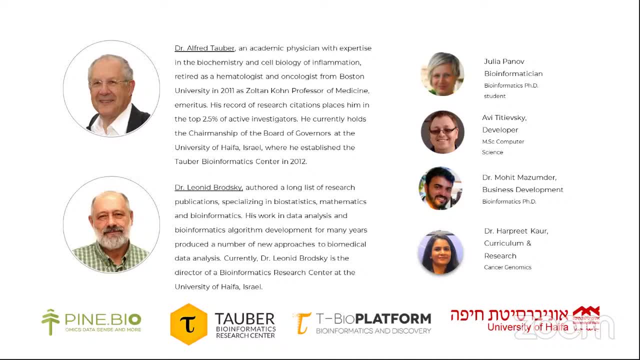 Dr Leonid Drozdsky is the director of Tauber Bioinformatics Research Center and is an expert in bioinformatics and biostatistics. He has numerous publications on bioinformatics and over the course of his career he has developed multiple novel. 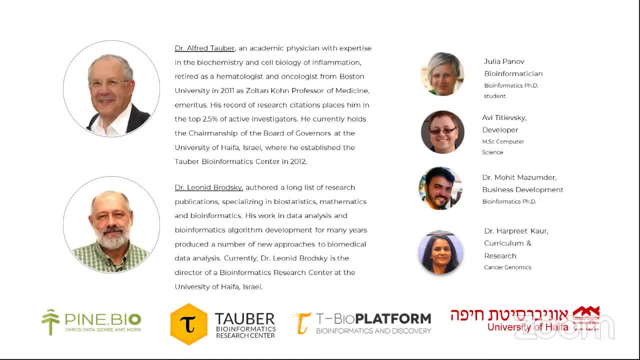 algorithmic approaches to biomedical data analysis. These have been widely used in basic and translational research and have been used in many other fields. Our platform is a result of hard work by some of the people mentioned here on the right: Julia Panov, who is an expert bioinformatician and helped prepare many of the materials that 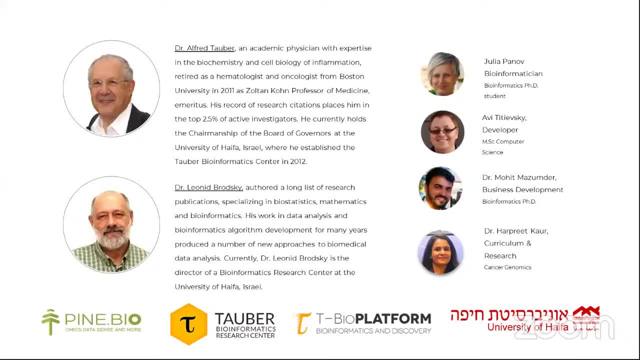 we would use in the course, Avi Titovsky, who is a computer scientist and leads the development of the T-Bioinfo platform that we would be using. Dr Harpreet has an expertise in the application of statistical machine learning techniques on biomedical data and 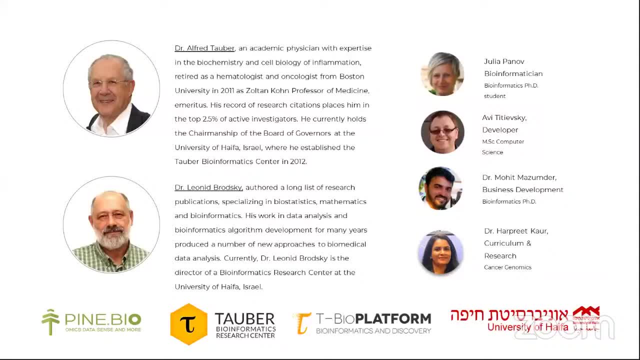 the development of prediction tools and databases as well. Dr Harpreet looks after the curriculum development, bioinformatics and data science course development as well. for the omics logic, Dr Mohit Mazumdar, who is an expert bioinformatician with multiple publications. 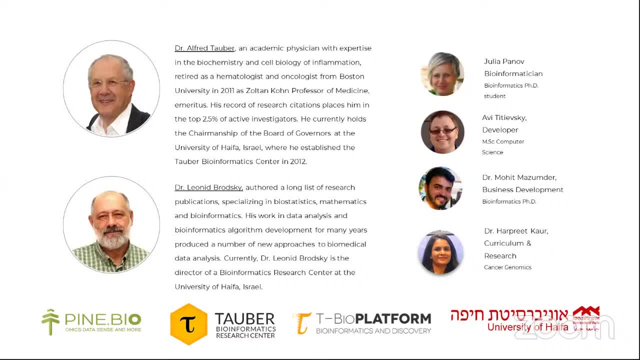 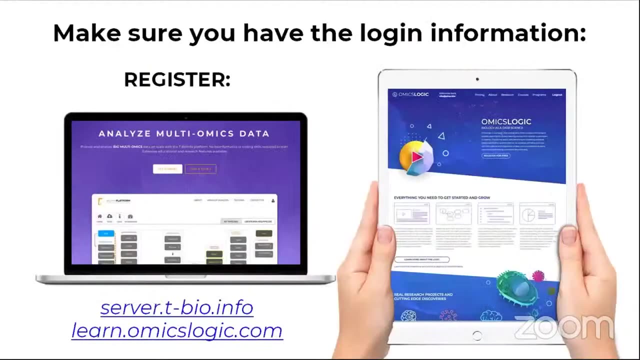 in peer-reviewed journals and collaborations in industry and academia. has been looking after the company's developing collaborations with universities as a mentor and a project lead for omics, logic training and research fellowship. Together with our collaborators, we have been building a growing online community of bioinformaticians. 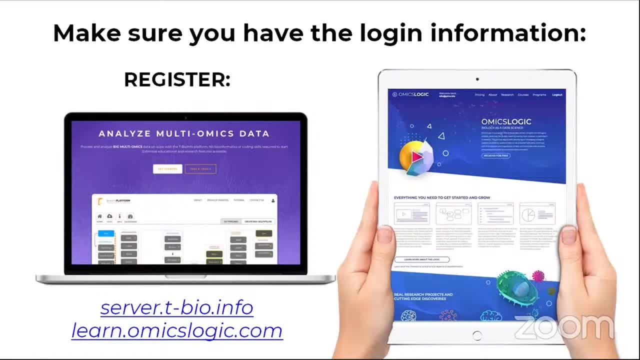 in training, ranging from high school students to faculty and researchers in top universities around the world. Our team offers big data analysis tools and quality learning resources like courses, projects and tutorials. In programs designed around various topics, we discuss bioinformatics approaches for processing, analysis, integration and interpretation of multi-omics. 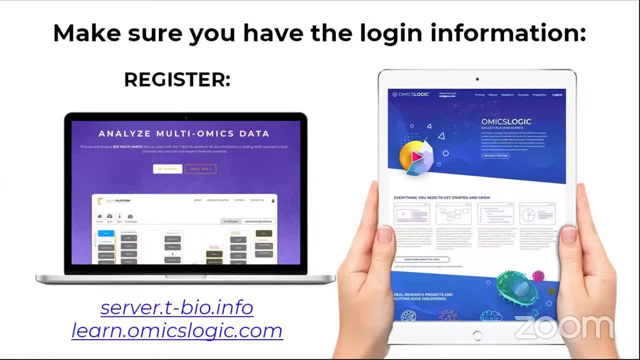 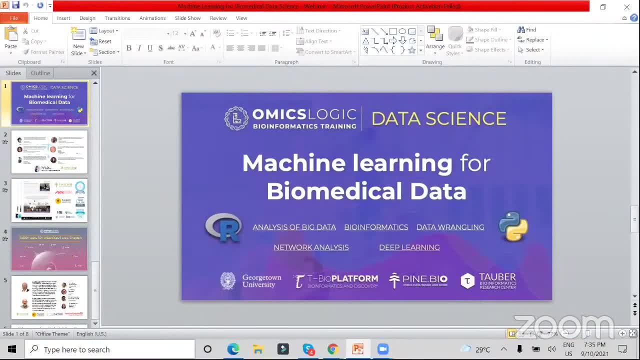 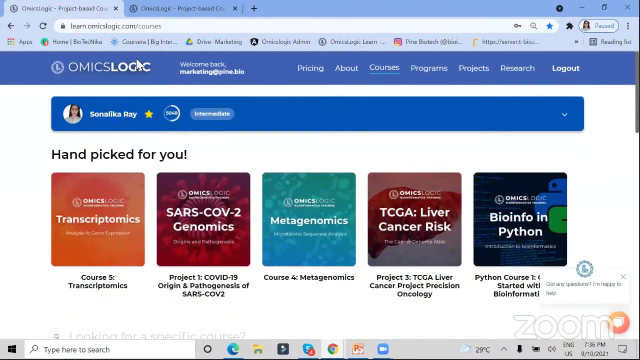 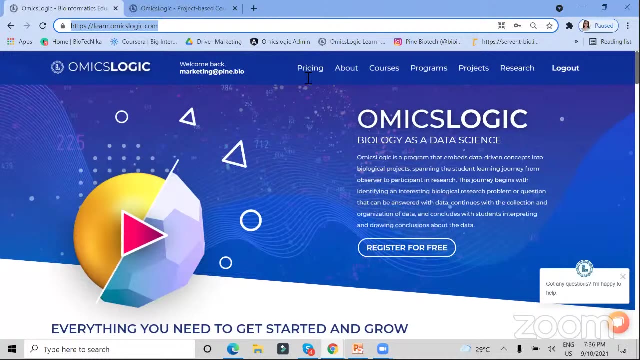 data from oncology, neuroscience, agrobiology and infectious diseases. I encourage you all to sign up now with me for free on our portal, omicslogiclearncom. So let me just post the link to the portal here. It is one of the best ways we can explore the world around us. 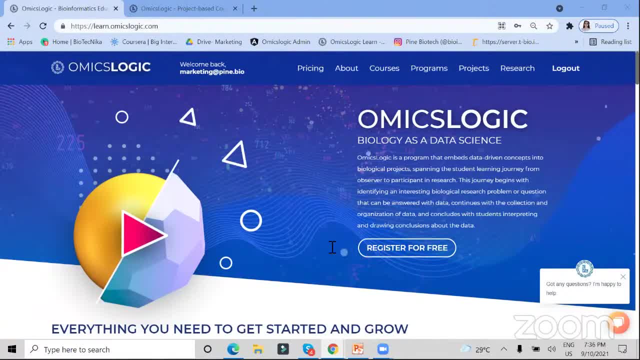 at the molecular level, with zero equipment or lab costs. So please make sure you are on learnomicslogiccom. I request you all to please subscribe to the channel and hit the bell icon to get notified when I post new videos. Please also ensure that you are signed up on the portal, as we are going to get some 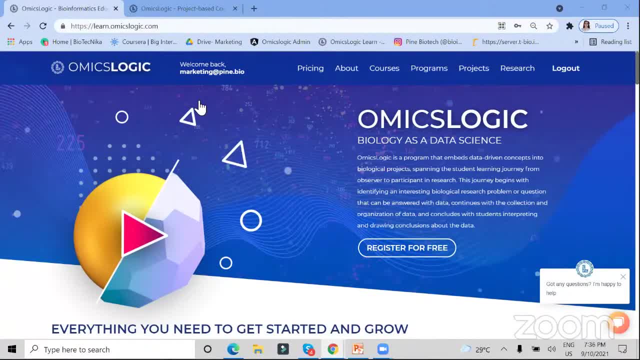 hands-on practice today and also explore the various courses related to data science in the next part of the session. Please type in a 1 or a yes once you are signed up on the portal and all set for the hands-on practice in the later part of the session. 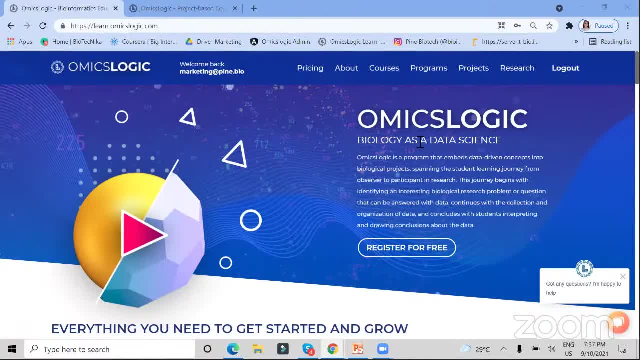 Thank you, Kenny Timmy. Thank you, Kenny Timmy. Thank you, Kenny Timmy. I would be giving in a minute. I would be giving in a minute for everyone to take their time to go to the portal and sign up real quick. 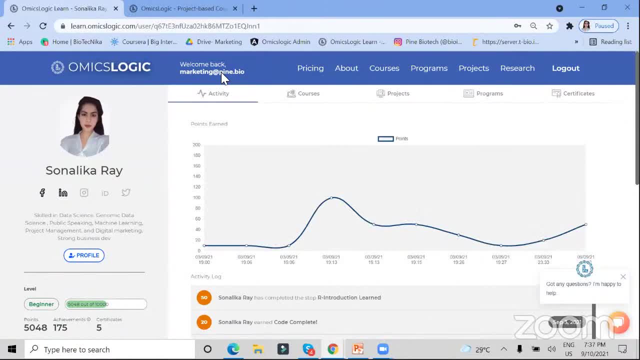 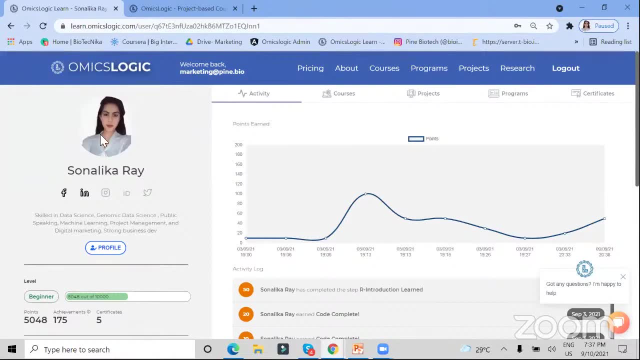 Once you are signed up, please make sure that you have an updated profile Now. when I say updated profile, I mean that you all should have an updated profile picture. Please have your social accounts connected to the profile itself: Facebook, LinkedIn, Instagram and Twitter could be one, and Google Scholar. 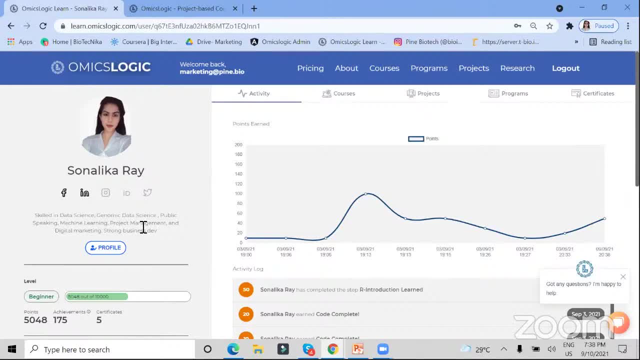 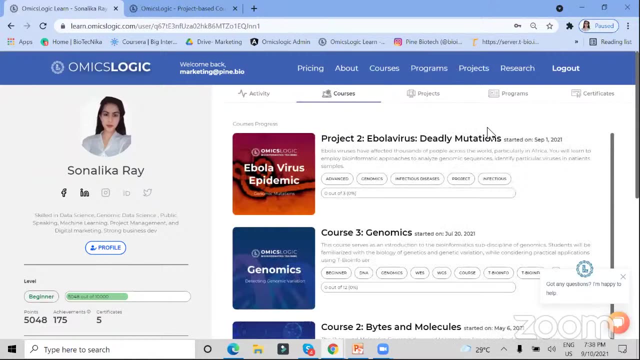 And then please add a brief bio about yourself. We would be monitoring your achievements here from your profile, and you would be able to also look at the courses and the projects or the programs that you are working on right now and get their certificates and download the same from your profile itself. 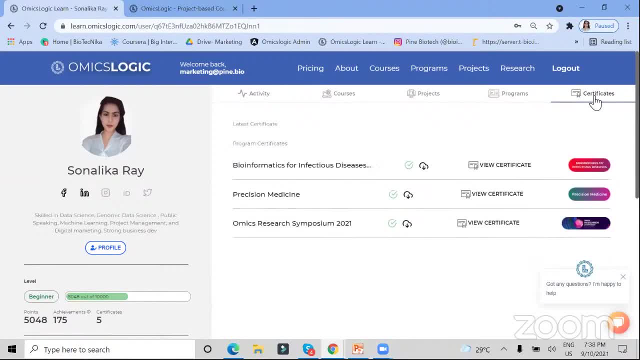 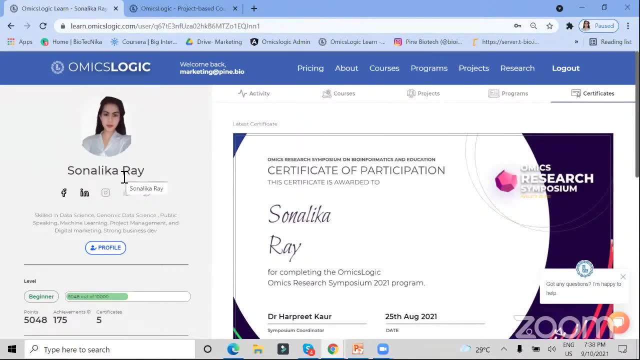 So it's important for you to please have an updated profile and make sure that you have your name in the comments. Also, please make sure that you have the correct title case and not in caps or in small letters, because that's what is going to come on your certificate. 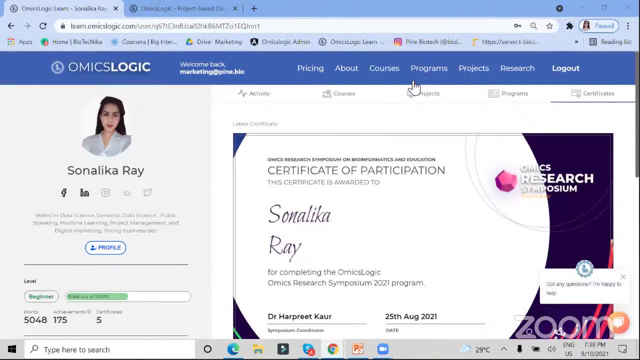 Okay, so before I pass it on to Ilya, a CEO of Pine Biotech, to talk further about the session, I would really like to have a poll, just to understand more about you all. The poll is going to be a little bit long. 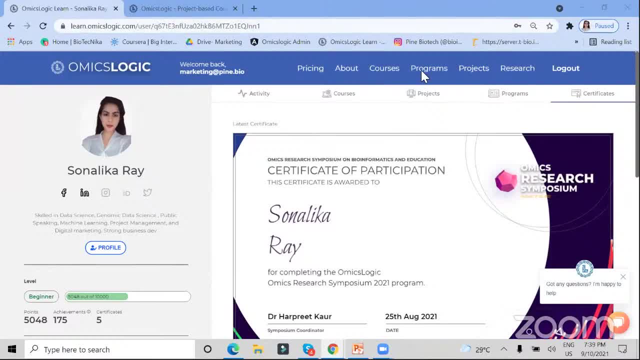 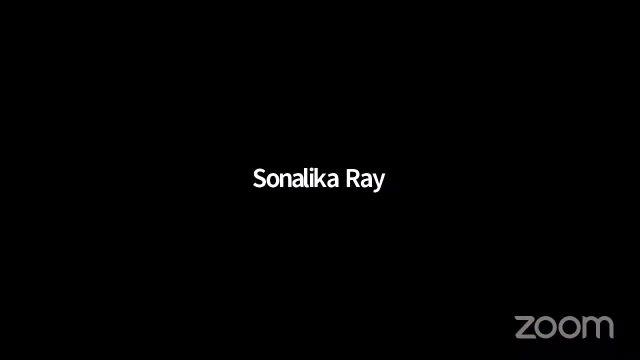 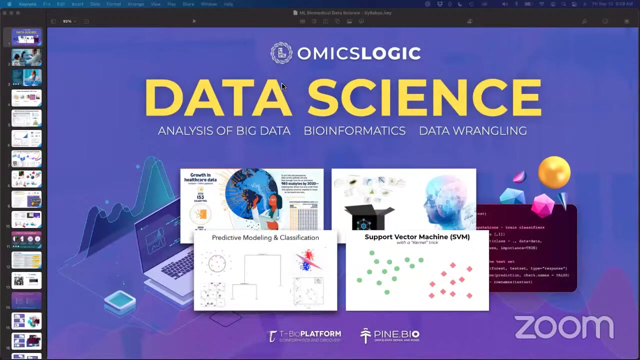 The poll would be on for a minute. Ilya, I would like to pass it on to you. So there's some technical glitch in having the poll on. You can start and after you, maybe I'll just have the poll. Thank you. 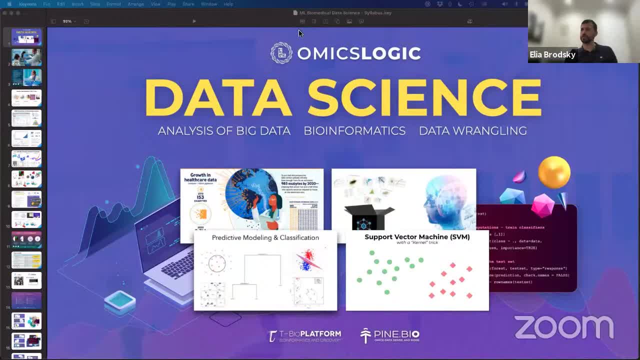 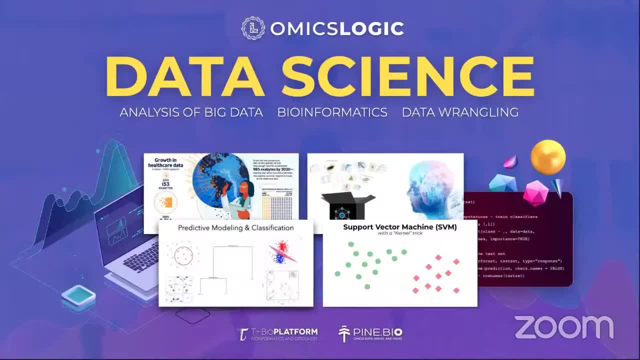 Okay, could you please make me a co-host at the same time? Yes, Ilya, I've made you the co-host, All right, Thank you. Welcome everyone to this webinar. I'm happy to see you all And welcome to Omnivore's Logic. 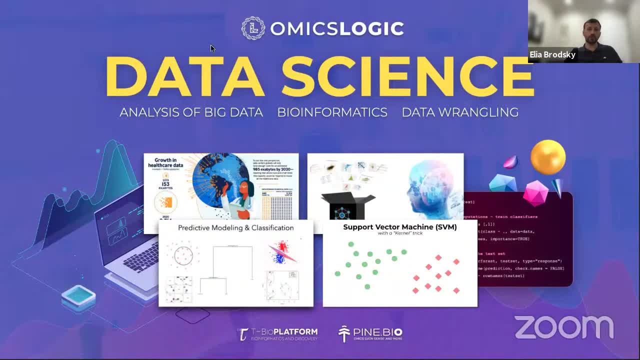 So what we'll do today is we'll kind of briefly talk about this upcoming program and explain how you can use various resources that we've prepared for you to learn about biomedical data and research. So I'm going to start with you, Ilya. 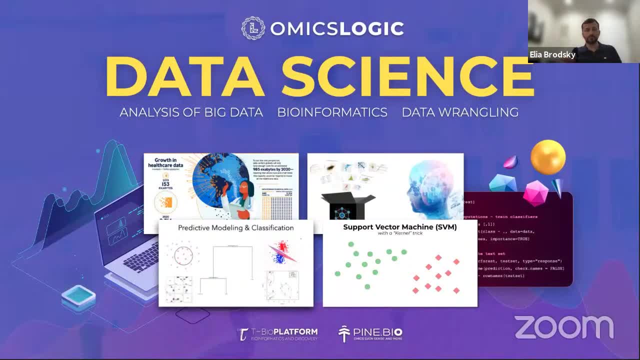 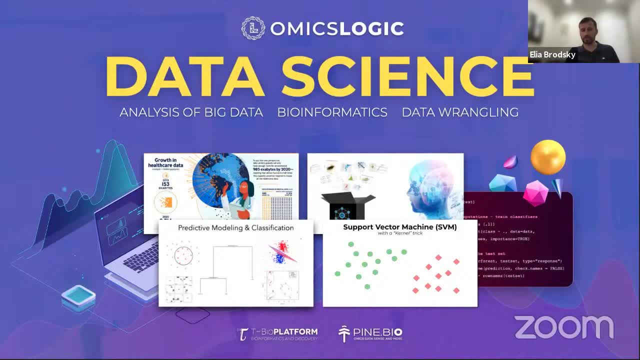 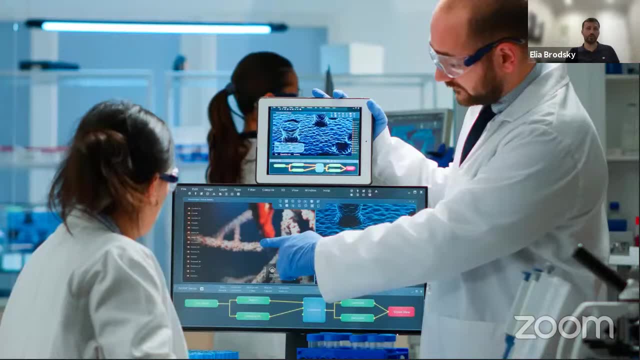 biomedical data analysis, machine learning, as well as some coding in R and Python. So, first of all, why machine learning? Why data science? So, as you probably know, some of the highest paying jobs and interesting tasks are being prepared to tackle data in a variety of ways. 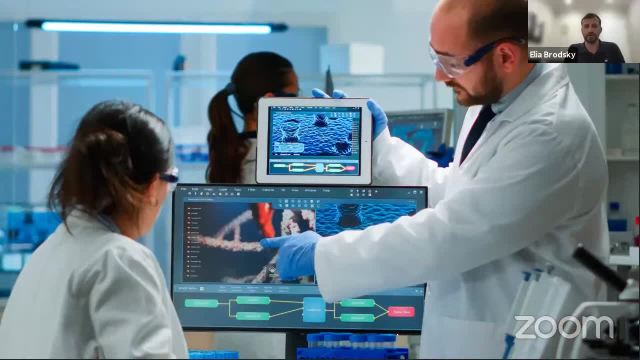 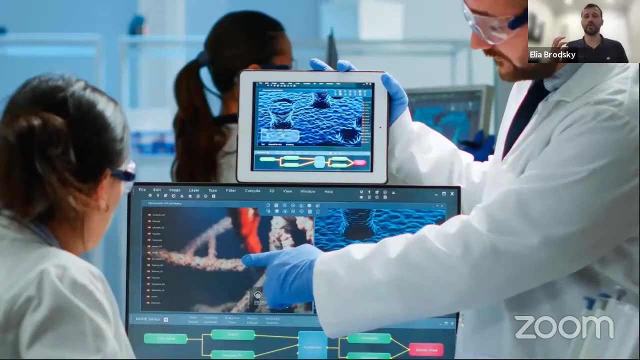 And especially this is happening in the world of biomedical discovery, pharmaceutical research, biotechnology companies, And the major objective for these companies is to take biological insights and translate them into applications And, a lot of times, to look deeper, just like we look in. 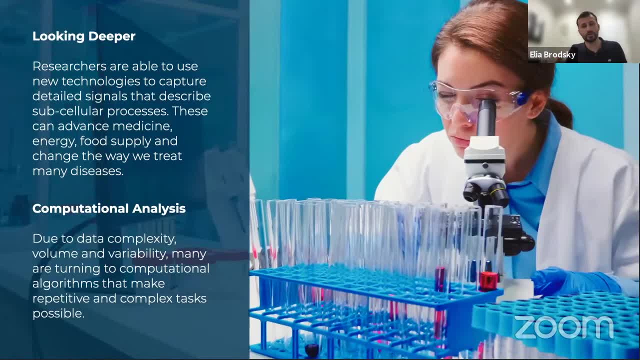 the microscope to understand the details of a biological sample. today we turn to computational analysis because the data is becoming more and more complex, large, variable and, essentially knowing how to use some of these tools can be a major component of your job description. 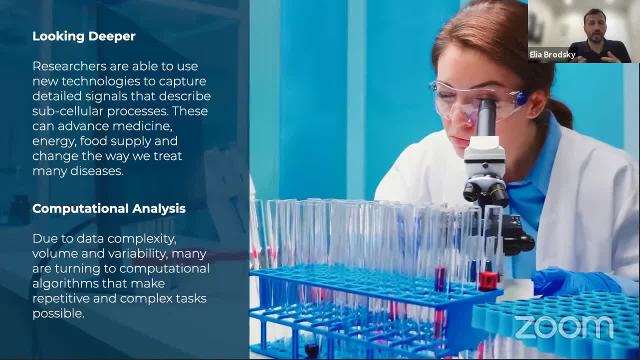 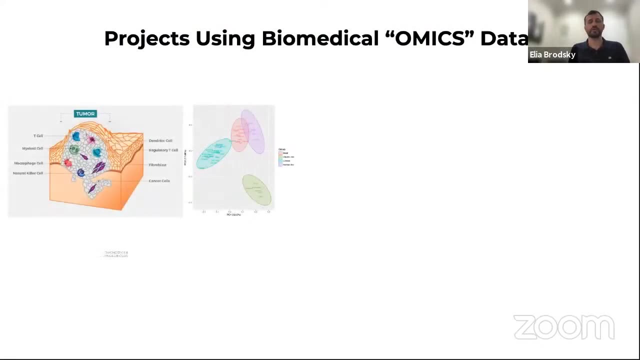 or it could be something that just drives your career and allows you to explore data sets and gain meaningful biological as well as clinical insights. So we'll talk a little bit more about the types of applications in a little bit. So what we want to do in this program is really 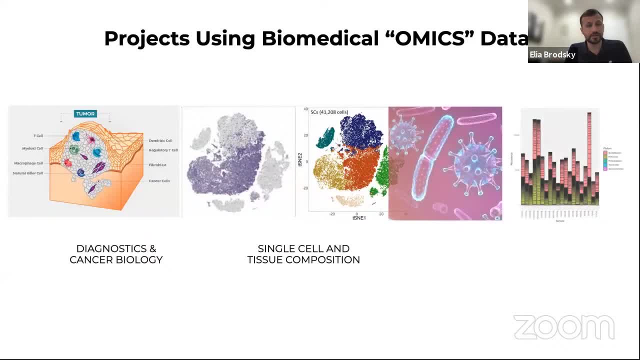 focus on some of the applications of data science, as well as machine learning, to different types of applications, So we're going to talk a little bit more about the different types of data. These data sets could describe challenges in diagnostics. When we talk about clinical applications, they could be discovery of targets that could be applicable to. 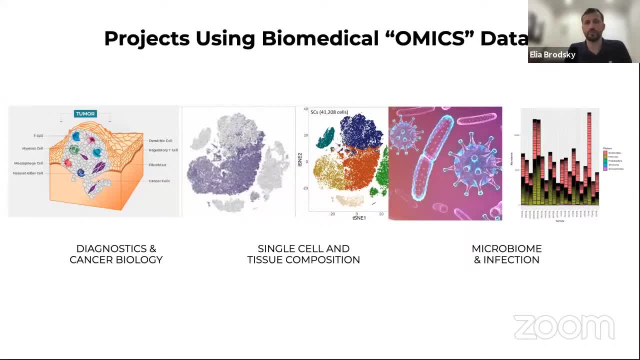 biotechnology or pharmaceutical companies. It could also be for basic research, where we look at environmental samples, clinical samples, animal models of human disease and try to understand what is the data telling us about a particular condition, phenotype or biological process. Now, I think the most exciting thing is that there are huge 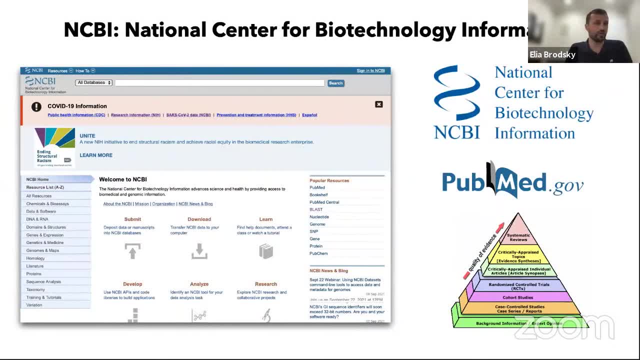 amounts of data available for anyone to learn from and analyze on repositories like the National Center for Biotechnology Information, or NCBI, where you have layers of information from processed information that has already been analyzed and interpreted and put into review articles or publications, but including all the way down to the raw data, And especially for the raw data. 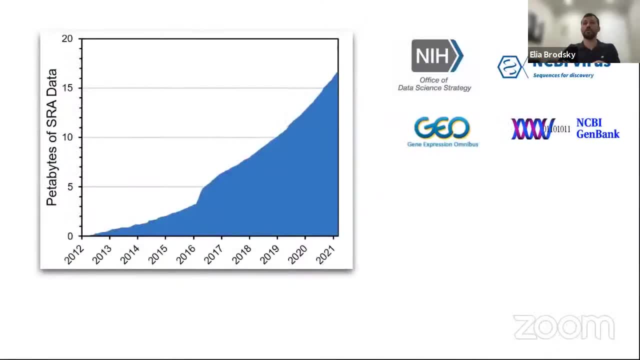 recently, there has been an analysis in 2021 where over 15 petabytes of SRA data, which is raw data, raw sequencing reads that have been deposited on NCBI. So what is 15 petabytes? 15 petabytes is 15,000 terabytes of raw data- raw sequence archives. 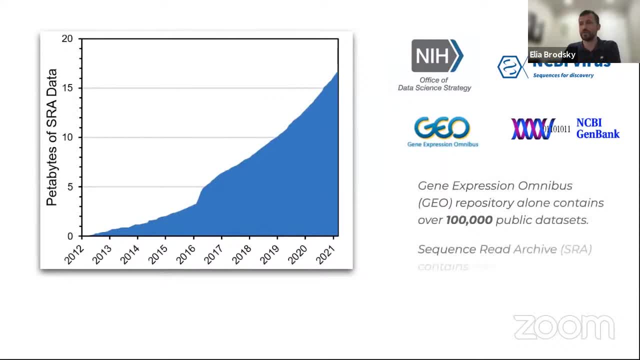 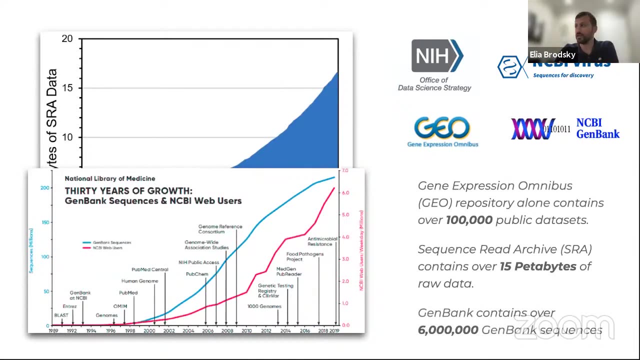 Now that includes some process data as well. There's over 100,000 public data sets for GEO, which is gene expression omnibus transcriptomic data, And there are a lot of over 6 million GenBank sequences, which means over 6 million individual species that have been sequenced, and 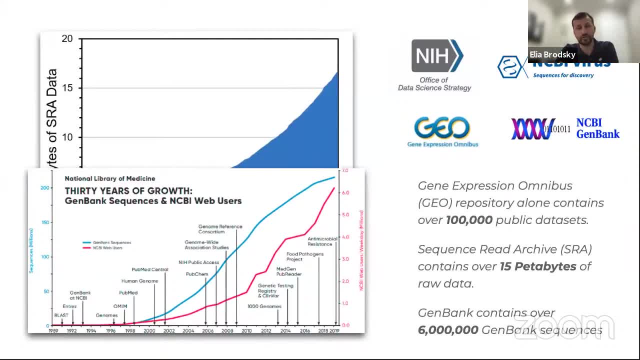 their genomes have been assembled. Now, a lot of this is driven by what's happening right now. What are the hot topics And what's the challenges, What are the challenges And what are the work And what are the challenges And what are the challenges And what are the work. 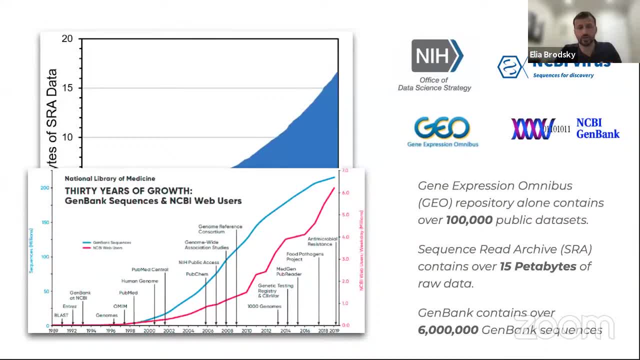 And what are the challenges And what are the work that we need to do to improve our processes in research, including clinical research, including basic research. And one of the major drivers, I think, right now is the pandemic which has brought about almost real-time sequencing. 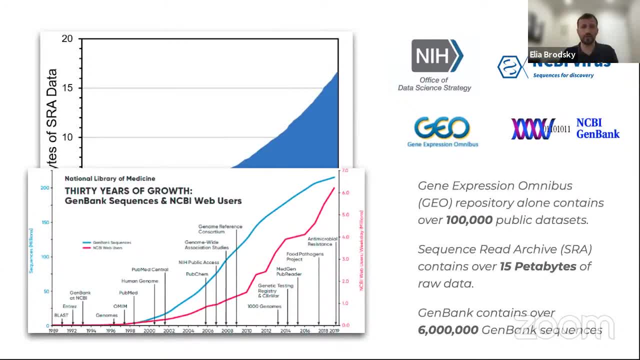 to the forefront, really allowing many of us to not only learn about the impact of the pandemic, but also look at how we can contribute to the understanding of this pandemic. Now, when it comes to such a diverse series of data, we need to understand what are the 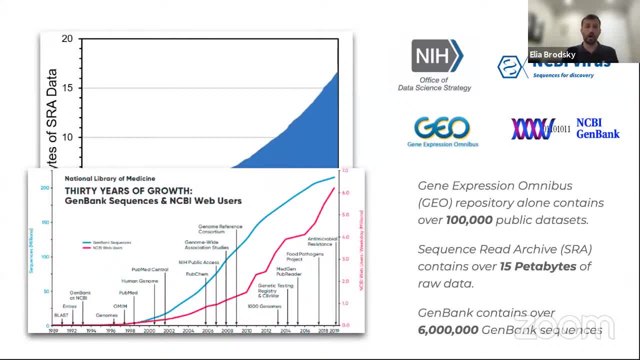 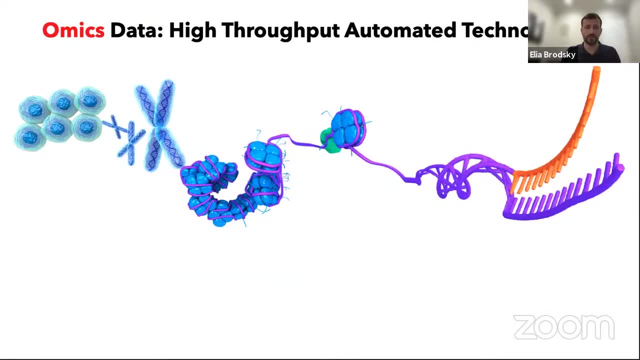 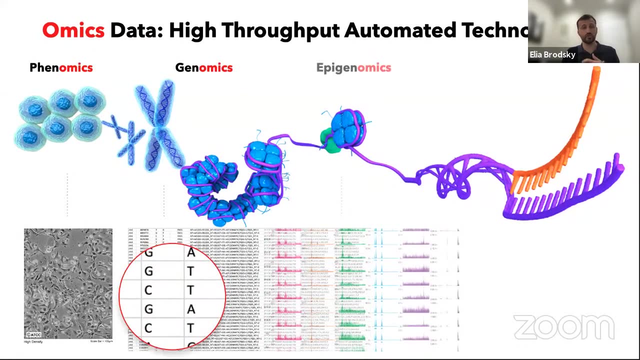 properties and challenges associated with each one. Omics data is a variety of comprehensive views of a particular type of data. Now, a lot of times, this is generated using what's called high-throughput technologies. These technologies include phenomics, genomics, epigenomics. 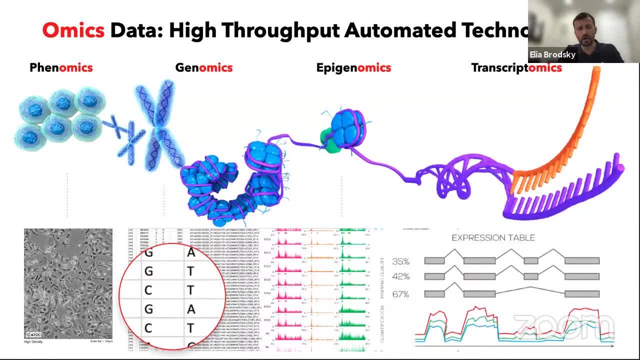 and transcriptomics, And all of these are relying on high-throughput or automated technologies to generate huge collections of data sets. Now, because they are so variable and they speak about different molecular properties, you have to rely on computational technologies to be able to learn from these data sets. 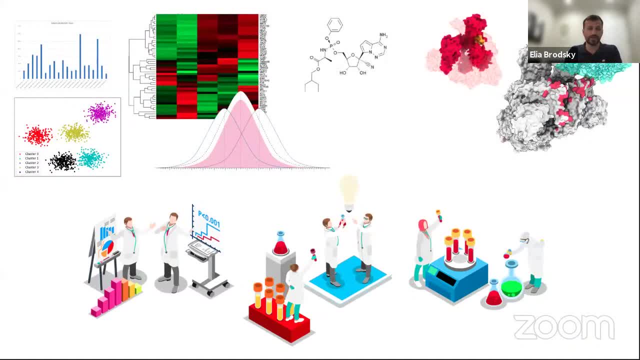 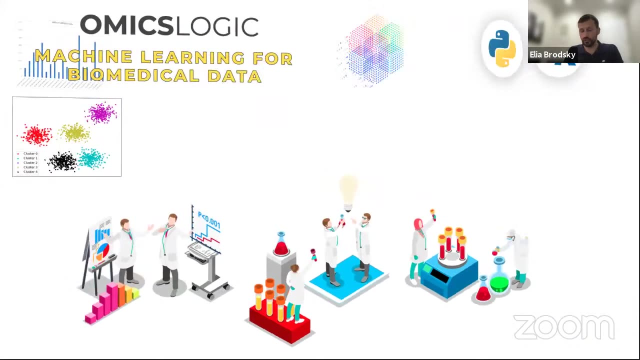 analyze these data sets, explore these data sets and make use of these data sets, And these computational technologies are basically rooted in data science, And so, in this program that we're going to introduce you today to, we're going to focus on some of these data science skills that you 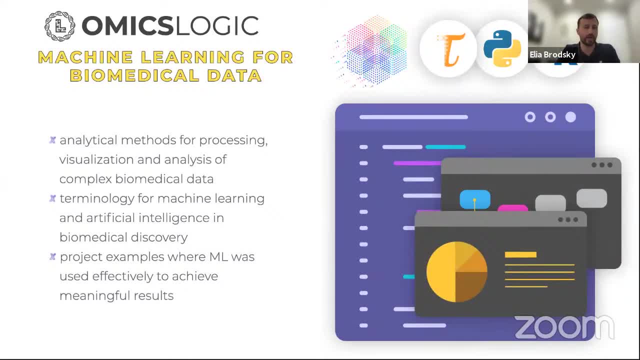 need to have to be able to efficiently process, analyze and visualize such complex biomedical data. So what are some of the things that we're going to cover in this program? First of all, we're going to talk about analytical methods: how to visualize and analyze the data, complexity and 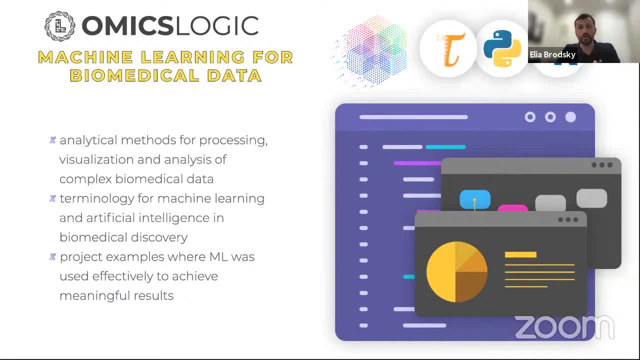 reduce information, How to analyze and analyze the data complexity and reduce information. And and then we're going to cover sort of the cognitive skills that we need to have to be able to analyze and replace the data complexity and reduce information. Now it so that we can extract meaningful insights. We'll introduce you to the terminology for machine. 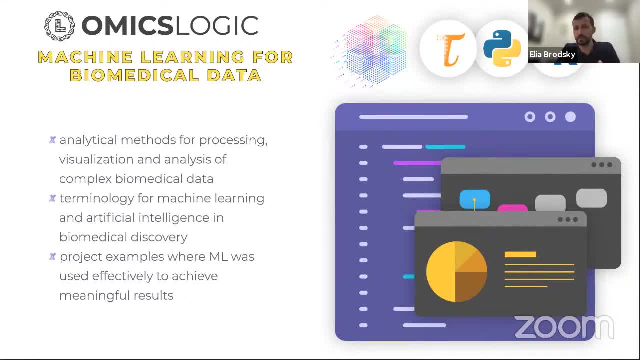 learning and artificial intelligence and biomedical discovery, so that when you read the paper and you hear about a method, you know what it does and you know what it means. We'll also provide you with some project examples so you'll see how other people have used machine learning Now. 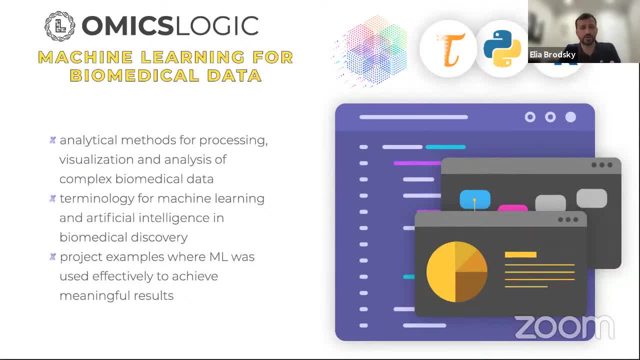 machine learning is used in many different ways, And so you'll see how it's not just clustering or classification. You'll see how different types of machine learning methods are actually used in a variety of tasks related to the whole process, from getting raw data to then making it useful for 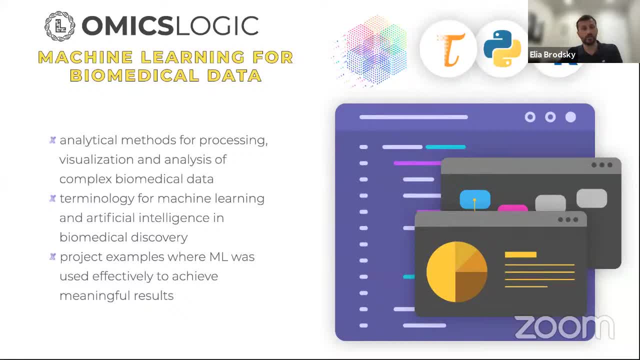 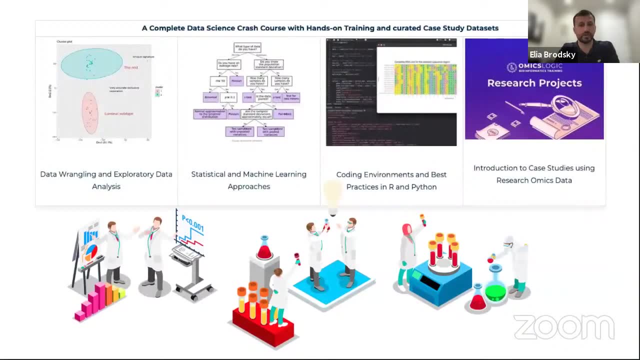 analysis, or structuring it, cleaning it, preparing it for analysis and then finally turning it into a model or learning from it, essentially using the complex patterns in that data. Now, as a result, what we expect the participant to gain out of this program is to really have an understanding of how machine learning algorithms 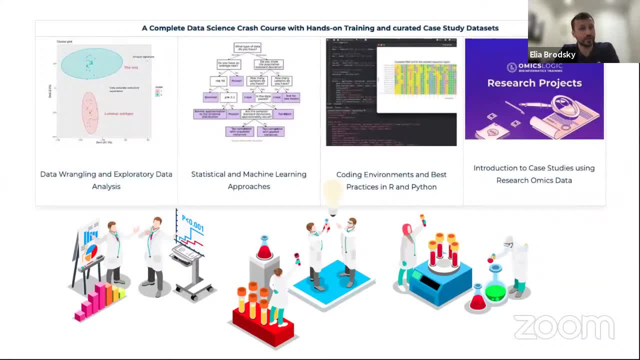 are used in analysis of omics data. You'll understand the differences between different types of machine learning models and different types of problems that they can be applied to. You'll also see practical examples So you'll have a sense of how other experts have used this, and 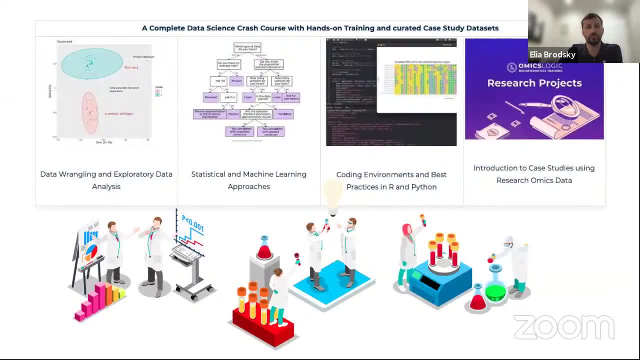 what are the specific challenges that they had to address to make their project work, And we will introduce you to some of the popular and user-friendly Python and R packages so that you gain practical skills. You can actually use these skills to code yourself and you will be able to read other people's code understanding. 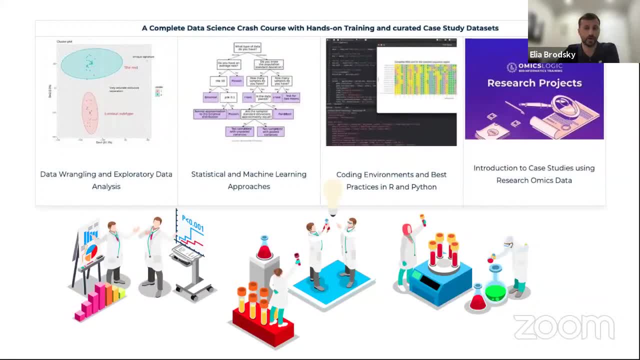 what packages are being used and how to use them yourselves, And so these are going to include some examples that we'll actually do today in this session, so that you get a sense of how can you get all of this done in a short period of time. So the data science program, the omics, logic data- 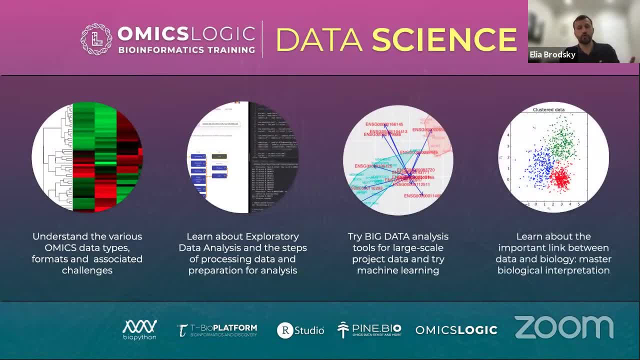 science program is really structured around these four different things: Understanding the various omics, data types, learning to explore them, then to try big data analysis in the context of a project, and then to understand the link between data and biology. How do you actually master biological interpretation? 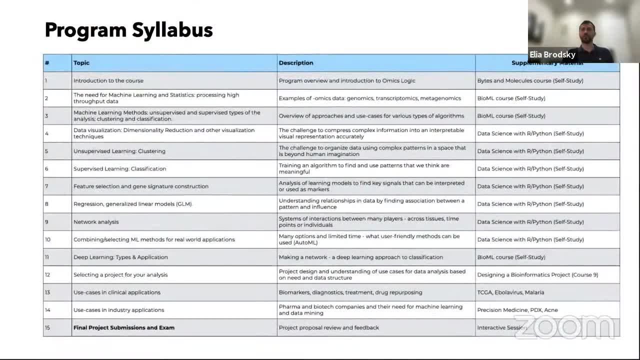 leveraging some of these tools. So let's talk a little bit about the syllabus. So the syllabus of this program is organized into three different parts: Introduction methods, an in-depth review of methods and finally the project section. So all together we'll have three. 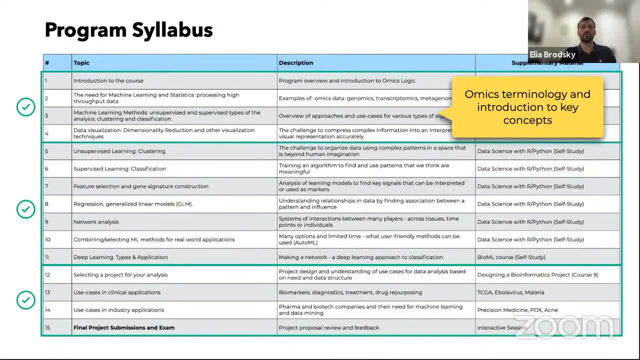 different sections. The first one will introduce you to the relevant terminology and key concepts to refresh your memory and get you started so that you're well-oriented in this whole field of omics and machine learning. The second one will talk about methods that will give you a practical 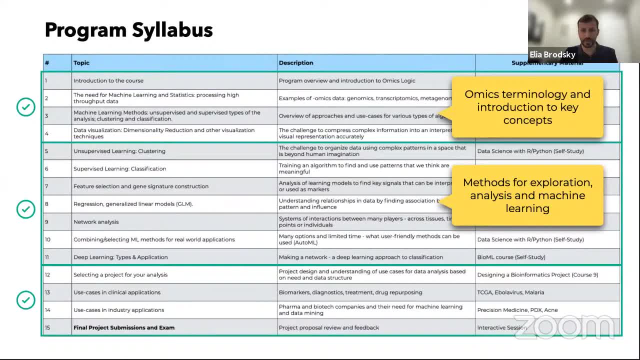 sense of commonly used methods and functions for analysis of omics data, starting from the exploration to statistical testing, to supervising and supervised machine learning, as well as deep learning, And then, finally, some project examples so that you have a sense of applications for such. 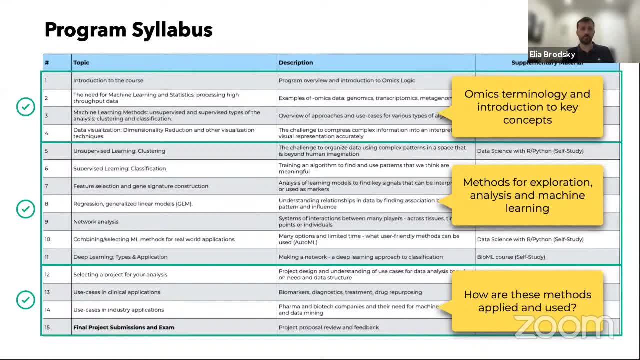 methods, And after you complete the full program, we hope that you will have the confidence to understand and analyze data that you can conduct independently to a data set of your choice, And we'll also introduce you, by the way, to some examples at the end, so you 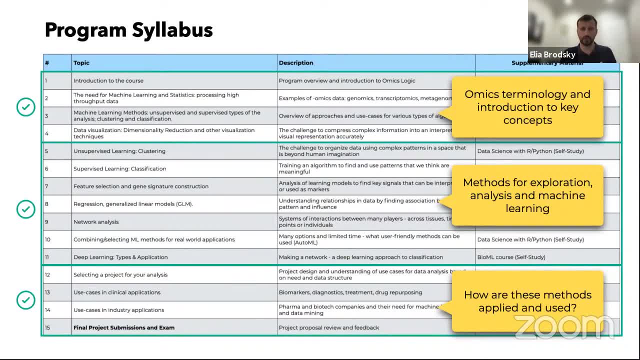 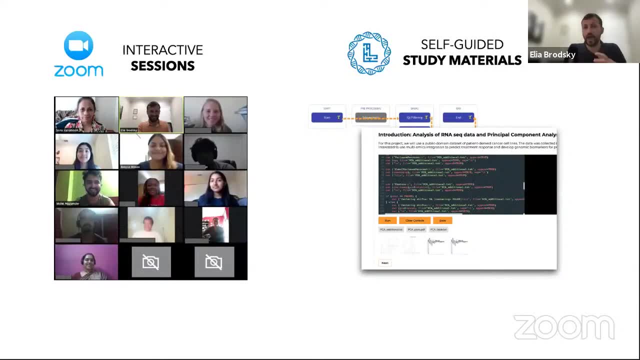 can kind of try it out before you do your own independent work. So the program itself is going to combine interactive sessions, just like we're having today. In each session you will find additional links to asynchronous resources that review and enrich the covered topics. So it's the live sessions plus the self-guided study materials. 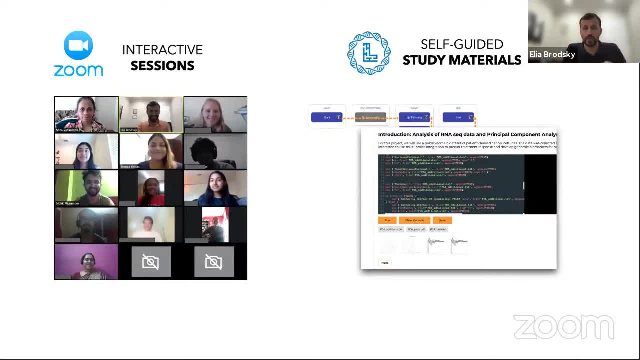 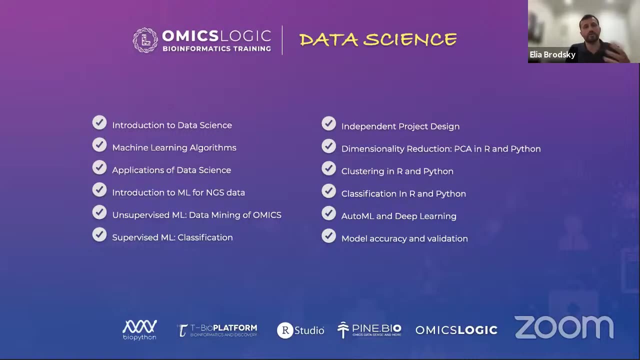 that you can practice and go deeper into If you want to learn more about the technical, the theoretical or the application of the particular topic. And as we kind of talk about a lot of topics in general, I want to kind of give you a high level overview of each one of these topics. So a lot of what we are talking. 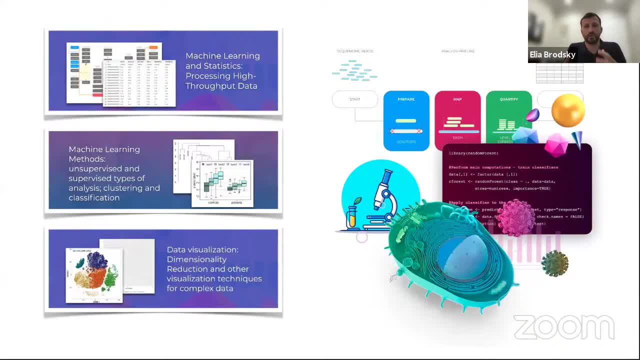 about when we say words like transcriptomics, genomics or metagenomics might be confusing to some of you, And so we will start in the beginning to kind of explain what is the link between the two And what is the link between the two And what is the link between the two. 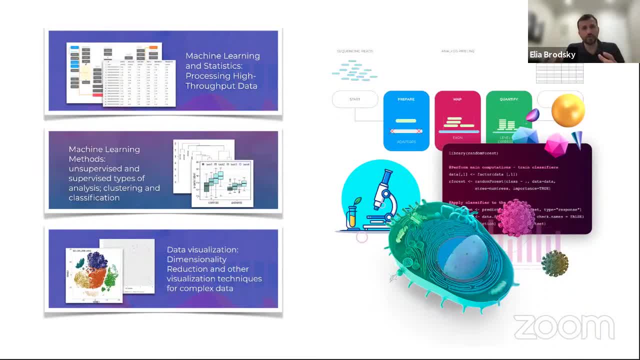 And what is the link between omics data, the biological features, the molecular features that they describe, and how can the data that comes from an automated process like sequencing can be used to essentially prepare it for analysis? So we want to link together the 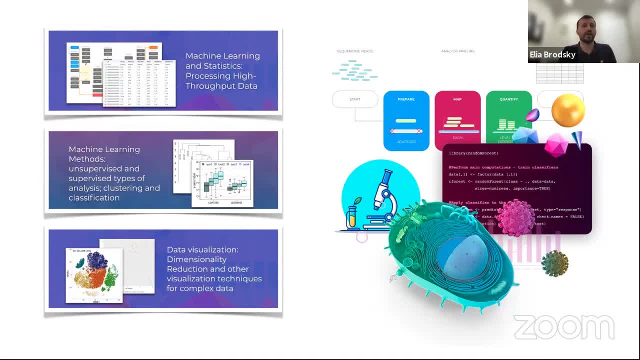 biological, the technical and the data components together, to kind of make sense of the important terminology and give you a practical sense of what does this data look like And how does it work in terms of using it for data analysis. Then, in the second part, 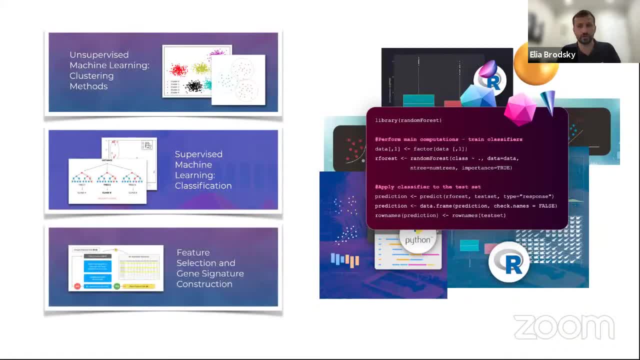 in the second part, we'll talk about the machine learning topics: Unsupervised and supervised learning. How are these methods used for various tasks such as visualization, organization of data, finding, signal in noisy omics data, as well as things like predictive analysis and feature? 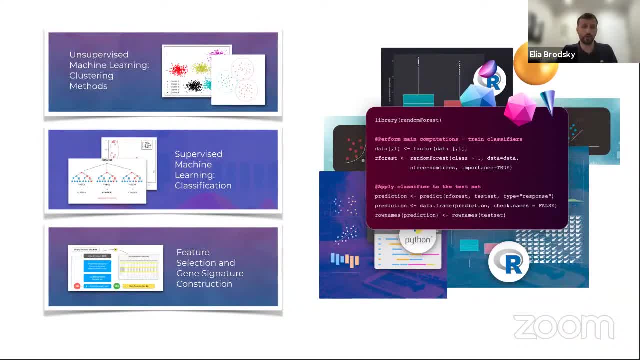 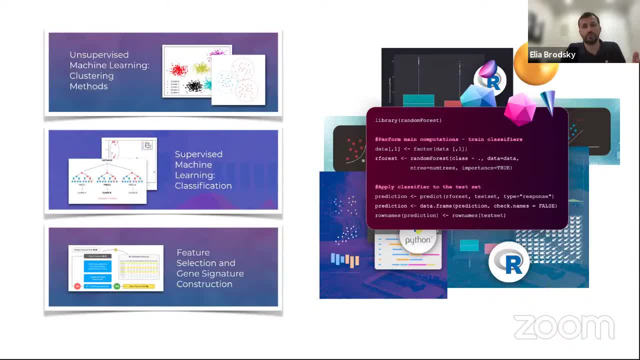 Settings and available packages that combine multiple functions that make the methods that we describe easy to deploy, right, So you can understand the method in detail. but then, as you want to deploy it, you want some user-friendly or some kind of a shortcut to essentially launch and train that model. So that's what you will learn. 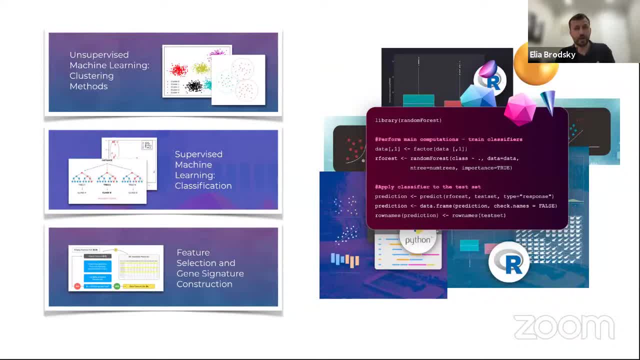 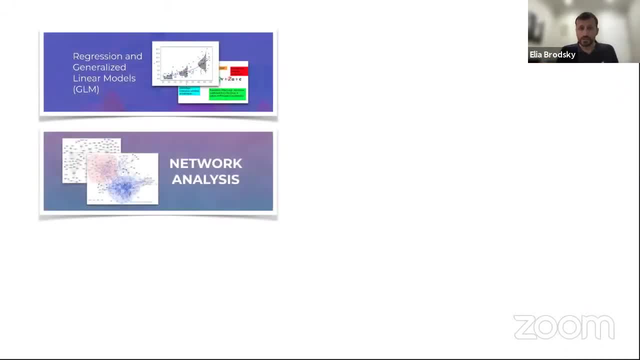 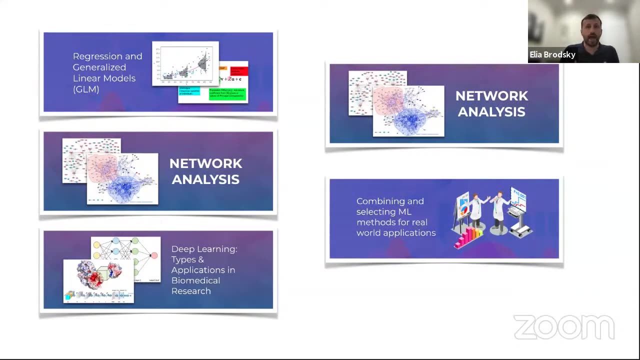 in this second part, You will learn to load data, select a method and run it to get an output that you can interpret for that particular model. Using these principles, we will then review additional methods that are useful for biomedical discovery that include network analysis, such as pathway analysis for biologists, generalized linear models that are used to distinguish between expression profiles of transcripts, for example, and complex transcriptomic data, as well as deep learning models that can be used for specific types of situations to improve accuracy and decrease feature engineering, which is a lot of what conventional machine learning relies on. 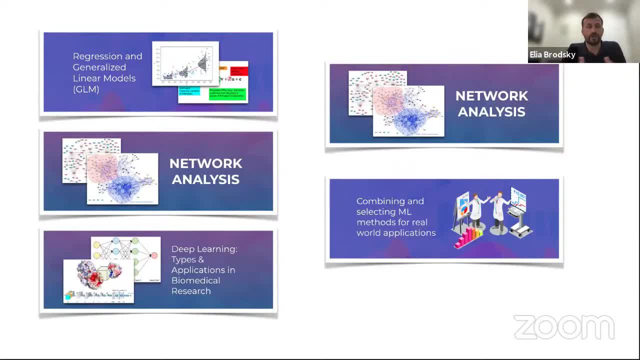 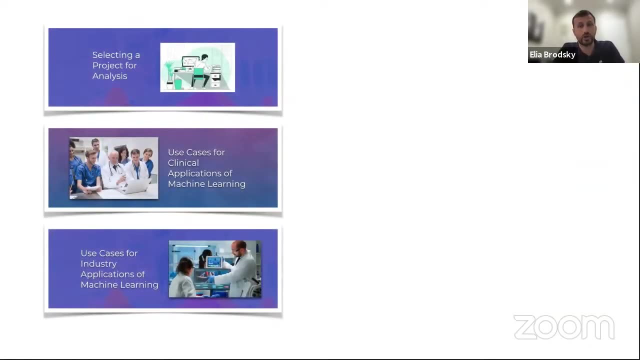 And then we'll also talk about the need to combine various machine learning models into a series of steps to achieve more complex tasks, for example when we talk about single cell data. And finally, we will talk about specific use cases that can show you how the methods we reviewed have been used by researchers to find meaningful insights in complex experiments, biological samples, animal models or patient data. 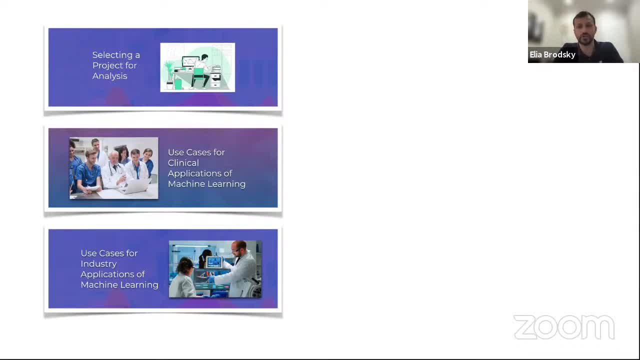 And so, with the few examples we review as case studies, you can also then develop a project of your own, or follow our asynchronous tutorials to reproduce an analysis that you can improve upon turning it into a novel study. So what are some of these projects? 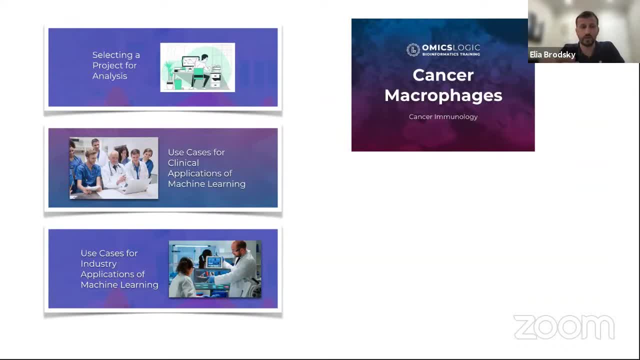 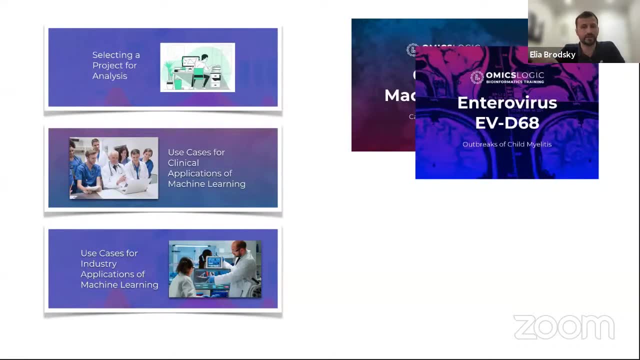 We'll talk about cancer macrophages, which is an important part of the immune system and the immune response to tumor growth. We'll talk about different types of pandemics like enterovirus, malaria or Ebola virus. We'll talk about modeling cancer precision medicine. 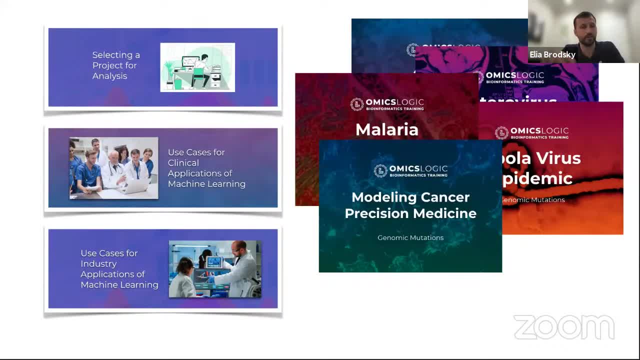 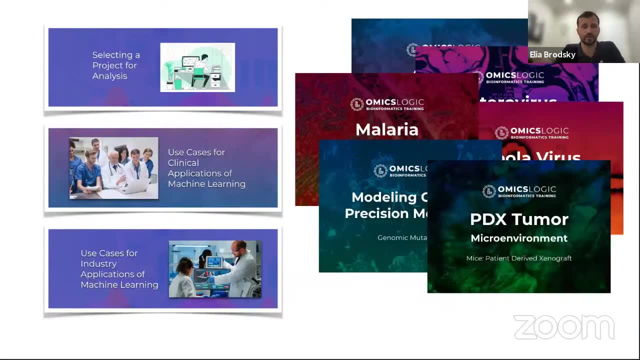 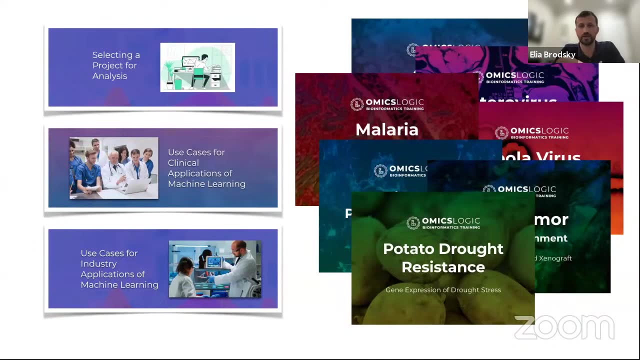 where we can find biomarkers and learn how different patients respond to different treatments. We'll talk about tumor microenvironment, but we'll also introduce projects that are not clinical in essence, things like drought resistance or different stresses that are important for crop production and environmental preservation. 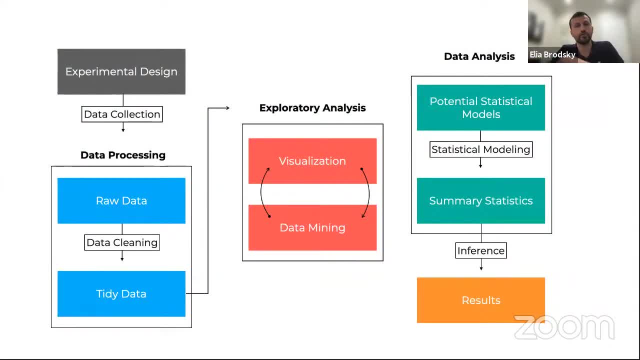 So, as a result, I think that you will really get a full overview of the data science kind of process in biomedical research to understand how different stages of analysis work together to help define the hypothesis as well as prepare the data for meaningful application of machine learning. 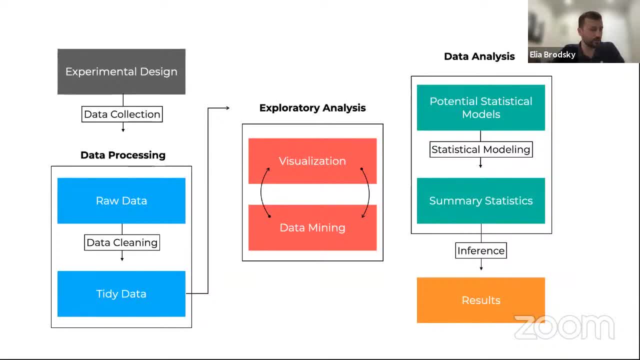 for big data practical challenges. So, as a result, you'll be able to take a dataset, make it useful and then explore it from a biological perspective to understand really what does it mean. As a result of completing all of these different steps, 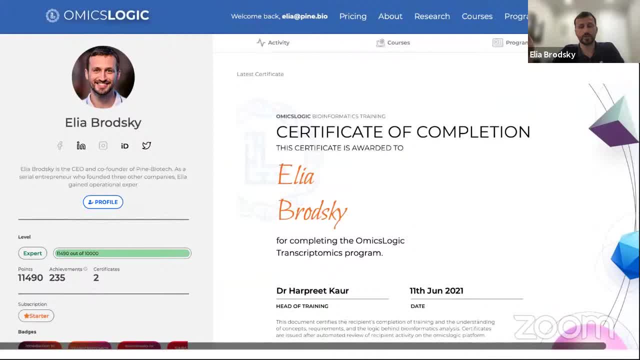 you will also get a certificate. So ask. already mentioned by Sonarica, you will get the certificate after completing all of these different steps on the Omix Learn portal. So now to kind of explain how all of these different resources are linked together and how to use them. I want to give you a practical sense of how this 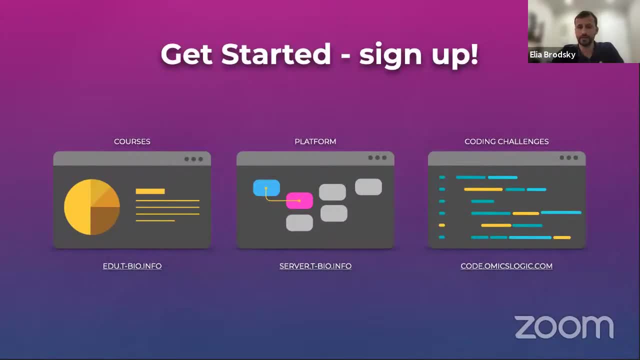 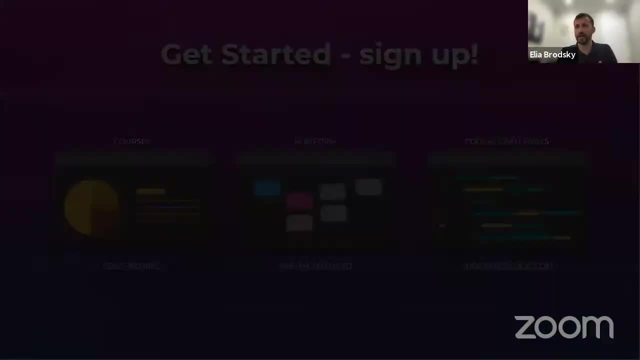 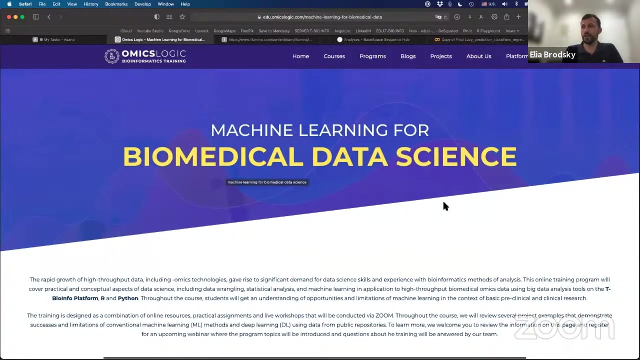 works. So for those of you that have not signed up yet, please go on to learnomixlogiccom and sign up and create an account, And then I will show you a couple of just really simple practical examples to illustrate what we will do. So this is the page where you have registered on the 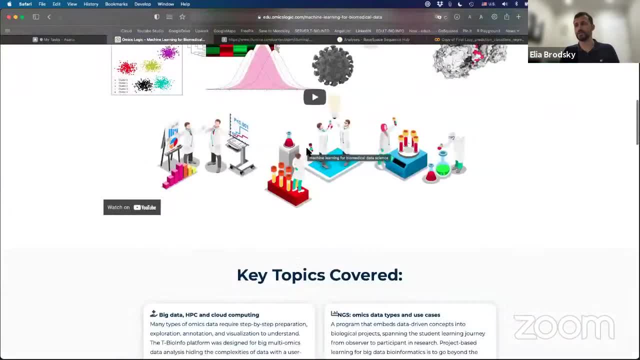 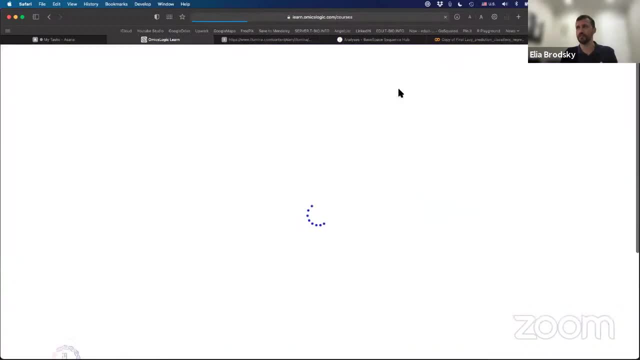 Learn portal for this webinar And, as you can see, it explains everything that I've described today And right here on the top, if you already have an account, we can go to the courses page And what I will do is- I will take one example- 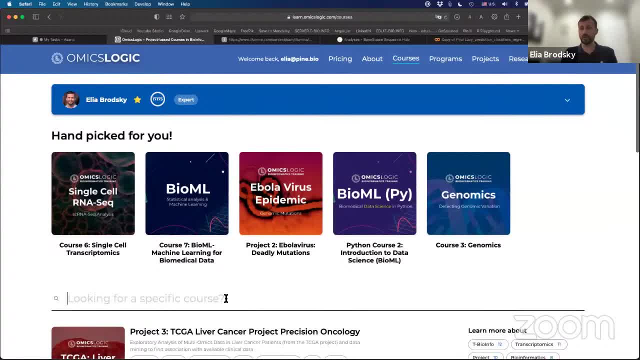 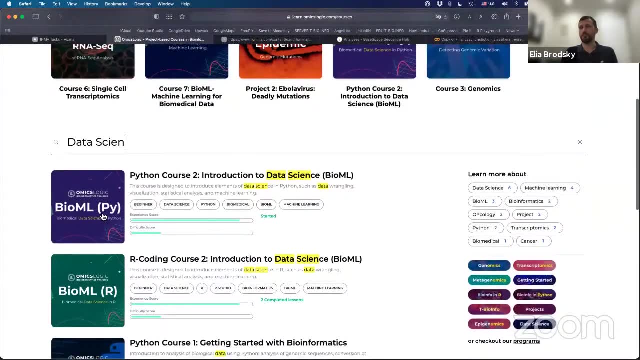 from the asynchronous materials that we will go through to just kind of illustrate what will be going on. So if you go into the search tab right here on the course page, if you go into the search, go to data science And you will see here BioML in Python and BioML in R, as well as some 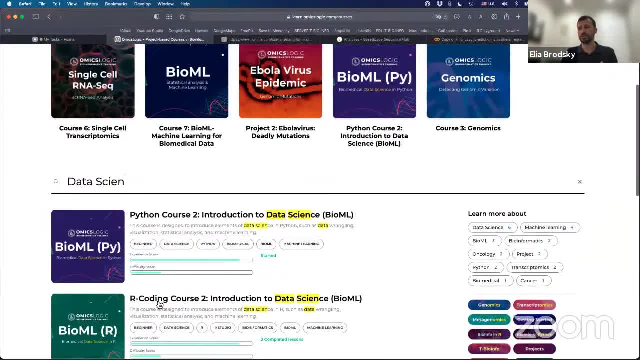 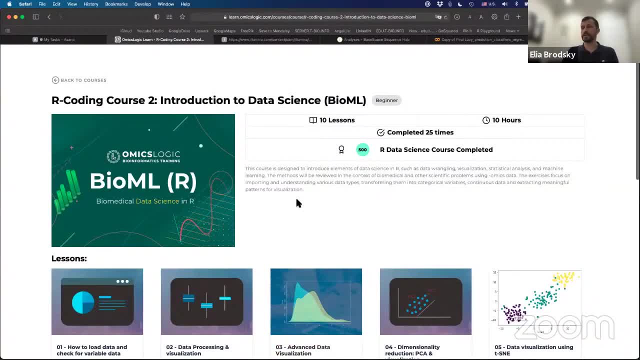 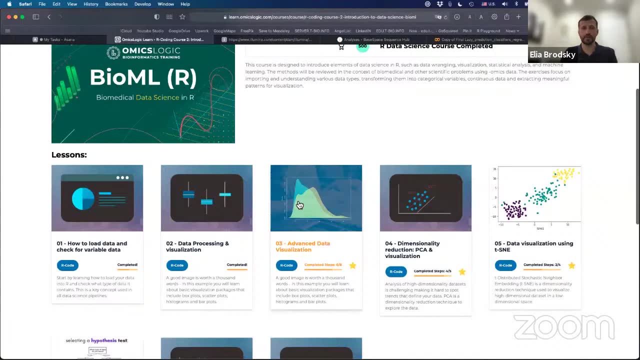 additional resources that you can look at, But right now we'll just take one example from this introduction to data science. We are taking an example from the history: research on how to get started with some of a lot of these basic tasks that we all have to get added to the basicф. 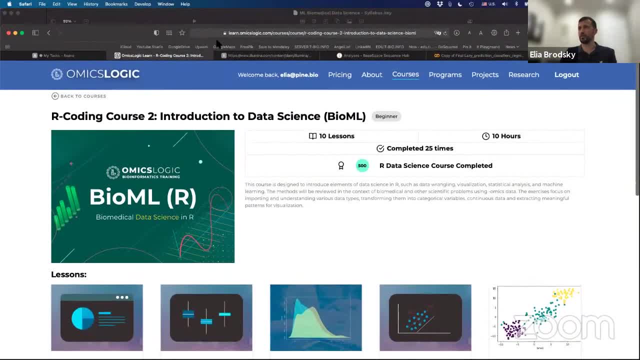 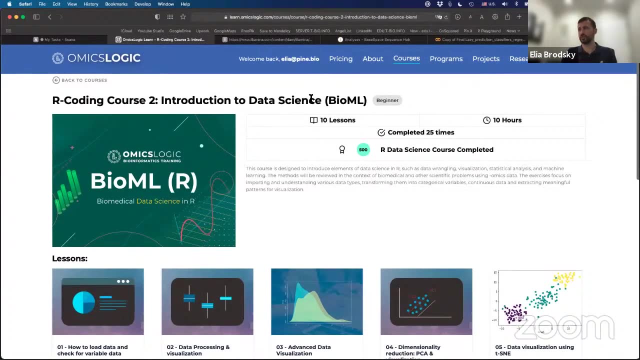 that we are getting into the program. So this is in the course. I'm just going to paste the link again in chatfor those of you that want to follow along. And in this course- This is again, or BioML- you will see all of the different courses that we have. There's about 10 courses. 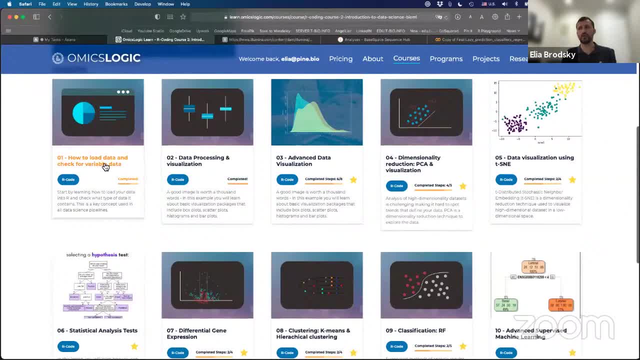 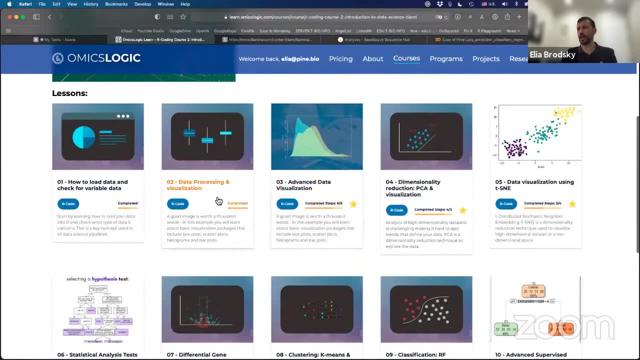 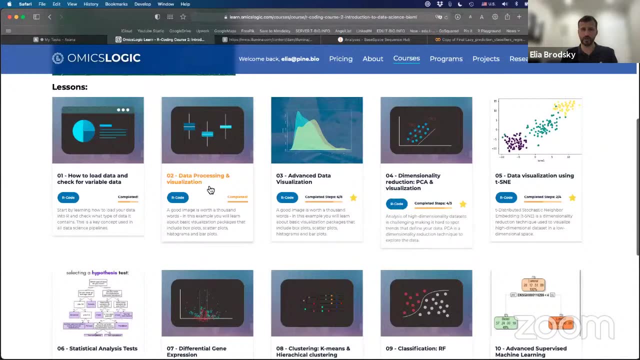 here that go from very, very basic things or how to load data and check for variable data, all the way to advanced supervised machine learning, right. So let's take a look. I'm going to use this course right here, or this lesson right here- Anyone without a paid subscription. 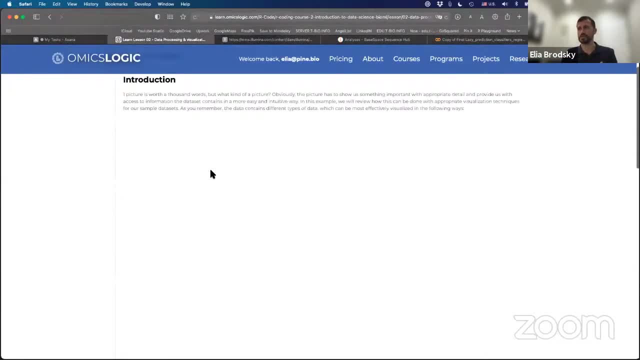 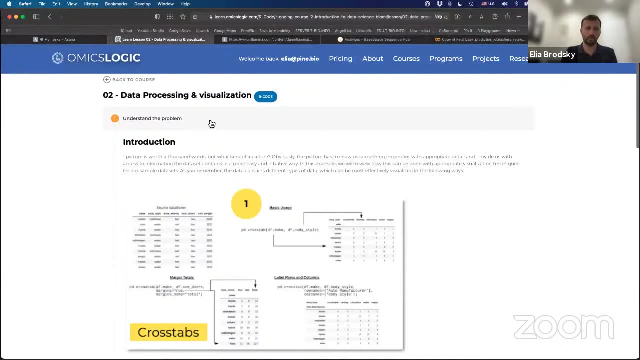 can access this lesson. It's called Data Processing and Visualization And basically what it talks about is once you have a table, once you have a table of gene expression, a table of OTU taxonomy in metagenomic sequencing of the microbiome, or whether you have some kind of frequency of 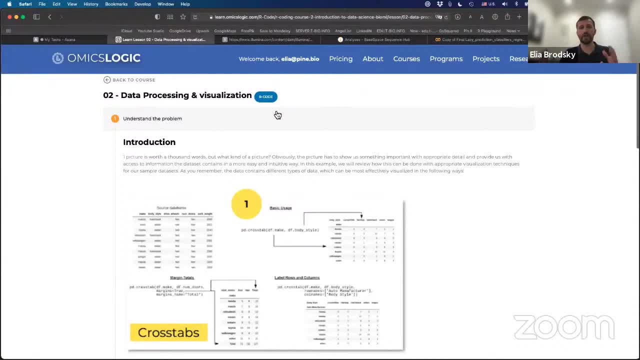 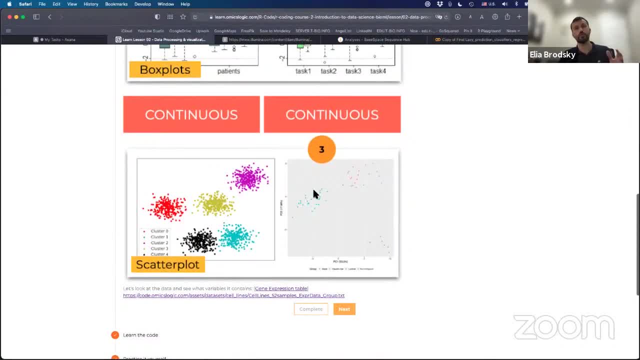 have different types of data. This data can include continuous numeric data such as transcriptomic gene expression. It could have names of samples and names of genes or OTUs, And it can also have categories, So these could be groups of samples that maybe define a particular type of samples. 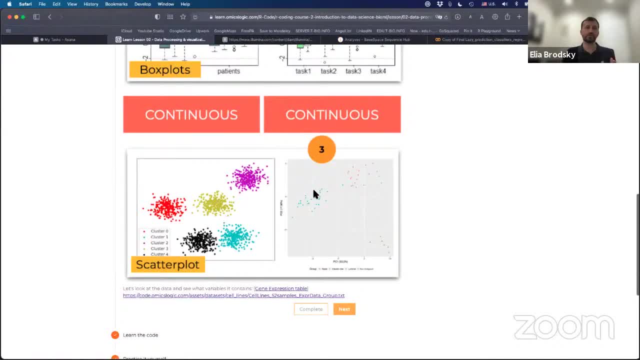 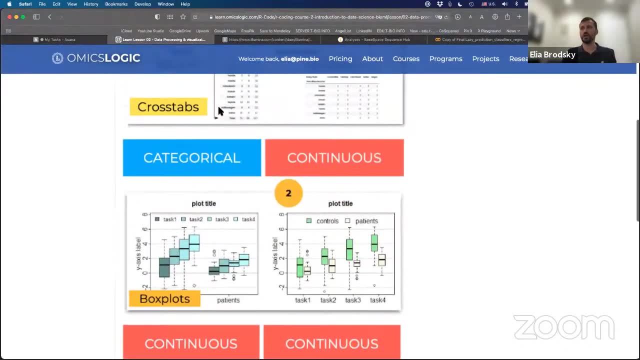 that you have Now to analyze such data. you can explore different methods of visualization that summarize the data in a meaningful way- And that's what we're going to talk about today- And that can include crosstabs or pivot tables. They can include box plots that summarize. 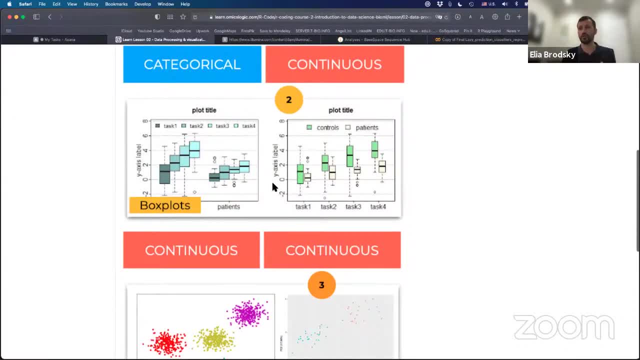 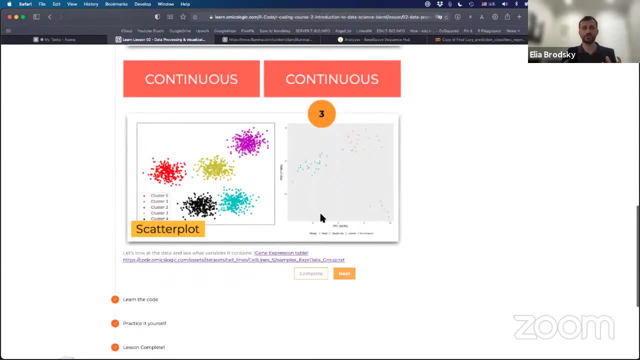 statistical properties of each sample or each group, And they can include continuous data, like scatter plots, that allow us to find relationships and organization of data that could be potentially interesting from a signal standpoint. So as we go through this introduction, you'll kind of learn about some of these methods And then we're going to talk about 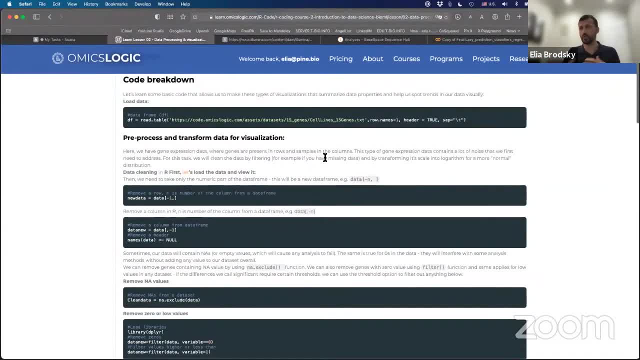 And then we can jump into the breakdown of this code. Now what's important is, first of all, loading the data, And so here you have an example of how you load a data set that is already on GitHub. Well, this particular example is on our portal, but we'll also be introducing you to how. 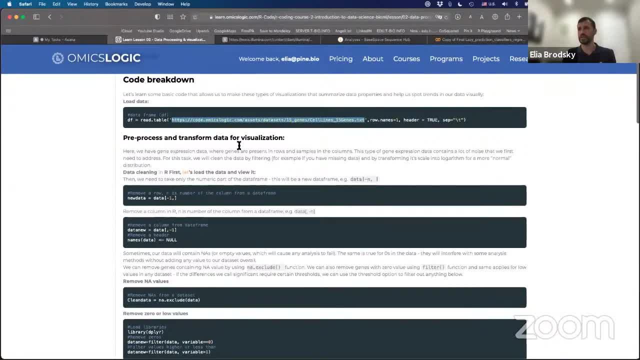 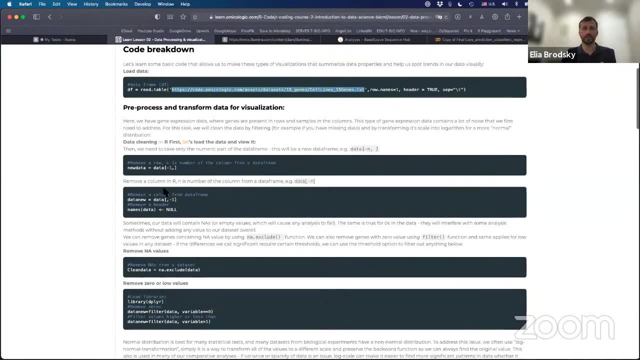 to use GitHub to kind of manage and organize your code as well as data sets. Then you can pre-process and transform your data for analysis. So here you have a data set that is already on GitHub. You can see that we can, for example, prepare the data matrix from the data frame that 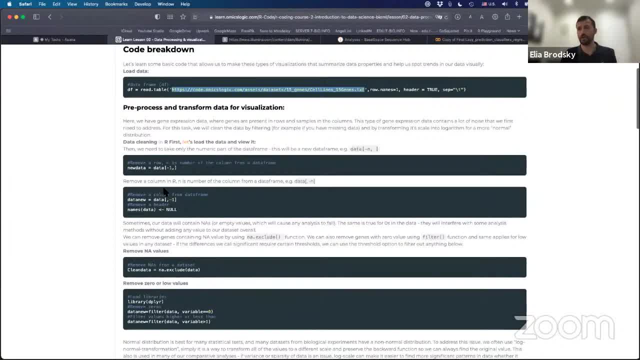 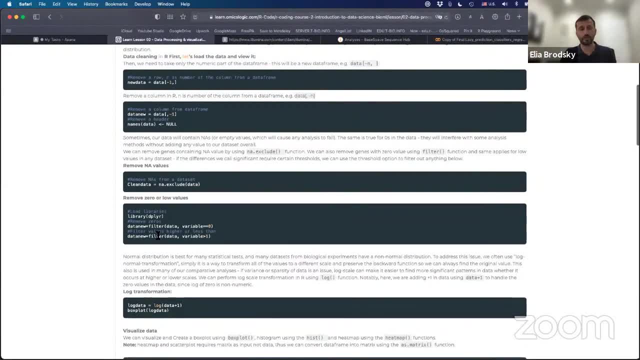 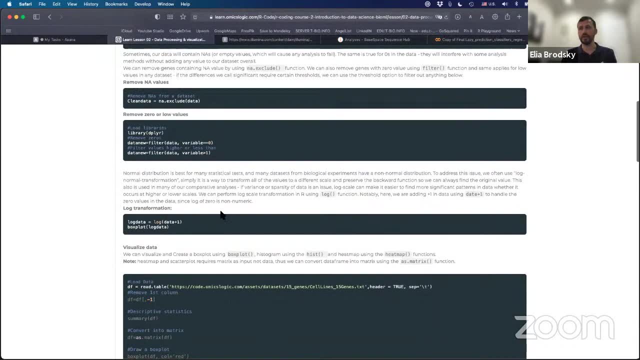 we have to create some numeric data for analysis. Then you can also load a library. A library is just a compilation of different functions that are going to be useful for the analysis and streamline your analysis, And in that data you now have an option to create a visualization like a box plot. 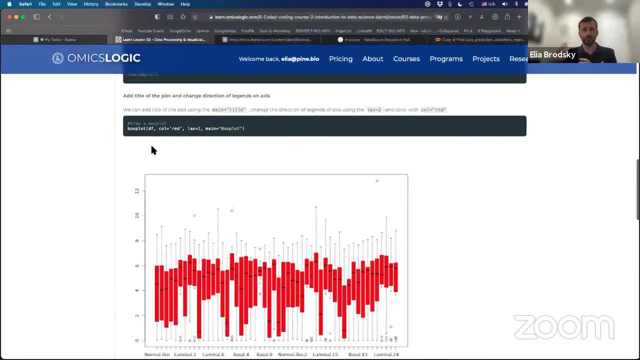 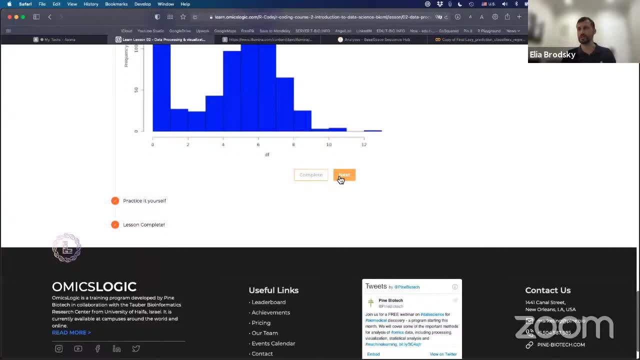 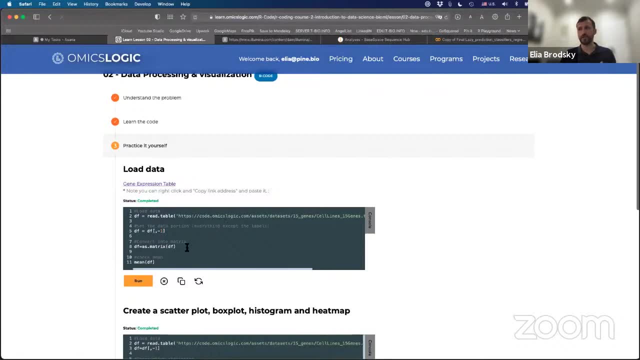 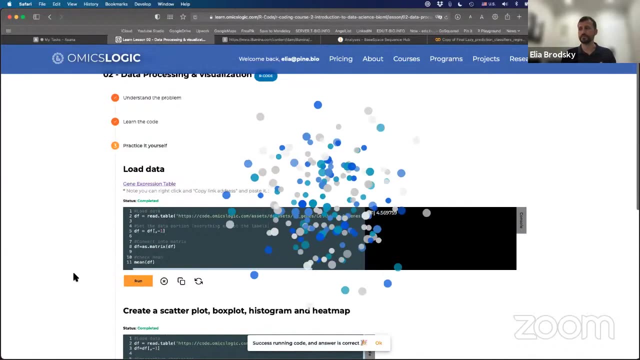 code. We can actually go into practice it yourself right here on the browser. So let's go into practice it yourself And let's try over here to run this analysis. So you see that now you have a console, You click on run And after this step is complete, you have a message: success running. 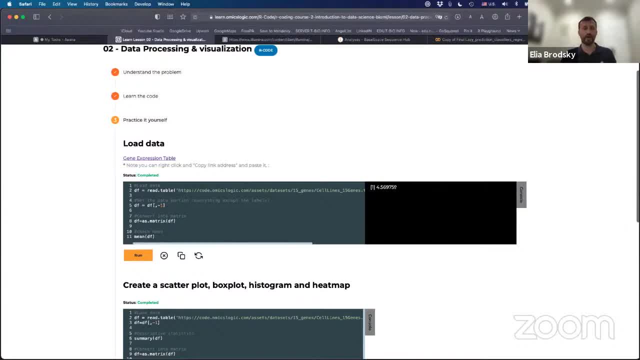 code. You see that basically the code is running, But you don't even have access to the other messages that are in there And essentially you can just stop the analysis from running. you get an output that was predefined for you to make sure that you're following the steps Now. 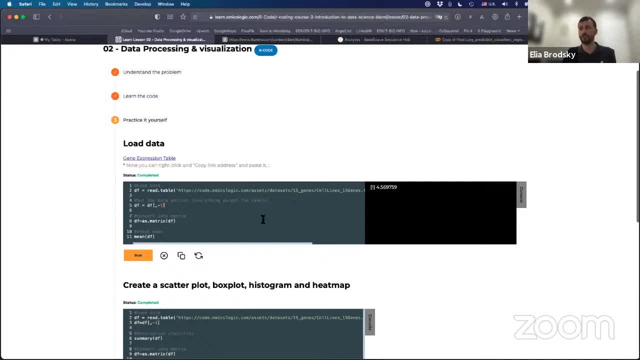 here. nothing really has to change. It's already made for you. What you can do, though, is you can check what's in this data. So let's go in here and we'll edit it, And we will put in head DF, which is the name of our data frame, to understand what is in our data. So, after we 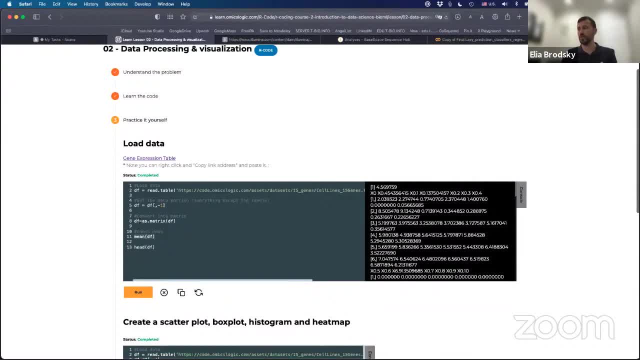 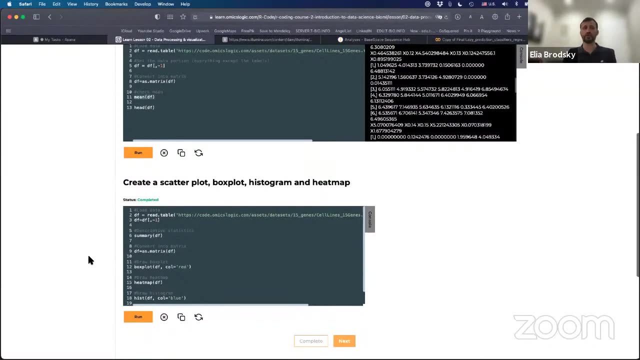 have calculated the mean, which is right. here we now see what is in our data. Now this is a little bit difficult to understand. As you can see, there's a lot of different columns, There's a lot of different numbers. It's not very clear. What do they actually mean? A more useful way to 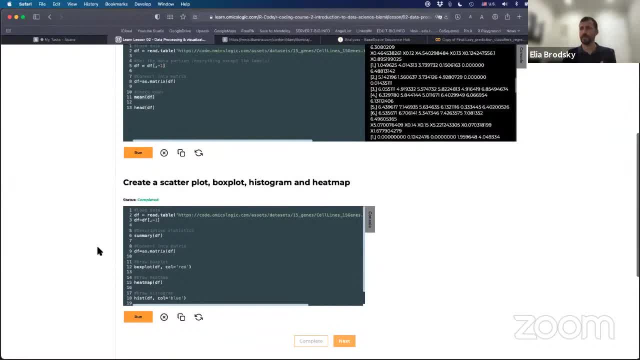 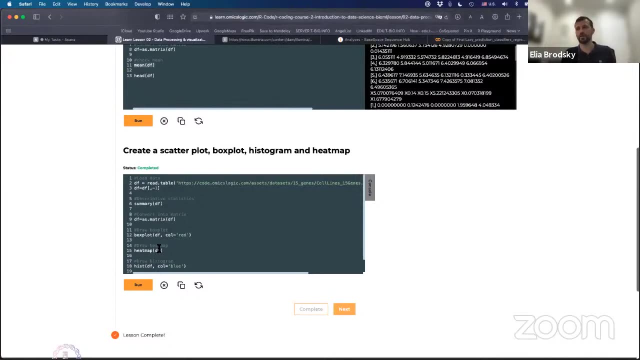 look at this data is to actually visualize it, What's in it, And so here we have a scatterplot, plot, boxplot, histogram and heat map, but all of it is connected into one single piece of code And, as a result, we might be a little bit confused as to what exactly are we. 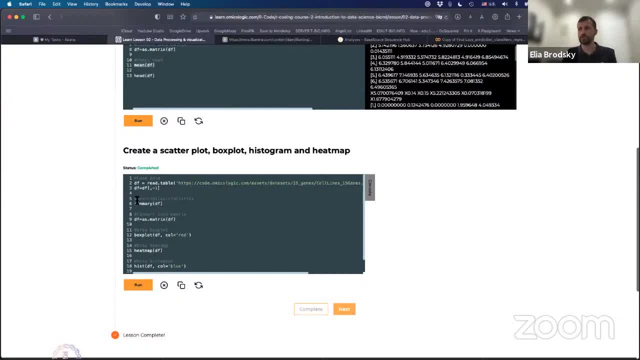 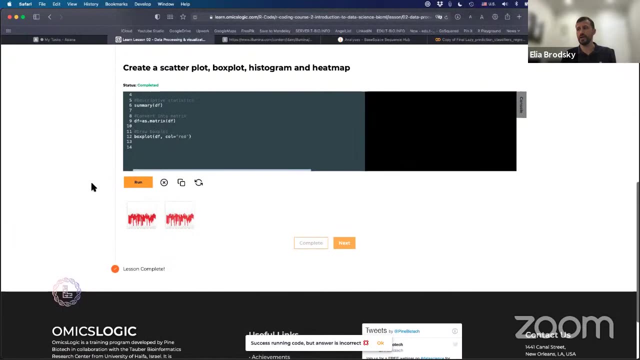 looking at. So let's modify this a little bit. Here we also have descriptive statistics converted into matrix, drawing boxplot, a heat map and a histogram. So let's start with the boxplot. So we'll just remove this, run it And now we have a boxplot. Now, what is a boxplot? A boxplot? 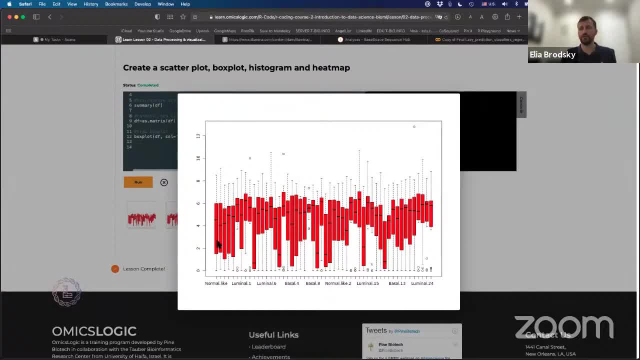 essentially shows us how the data is being processed. So we have a boxplot, a heat map and a histogram, And at the bottom there's the data, for each sample that we have on the x-axis can be summarized using the interquartile range maximum and minimum values outliers, as well as the 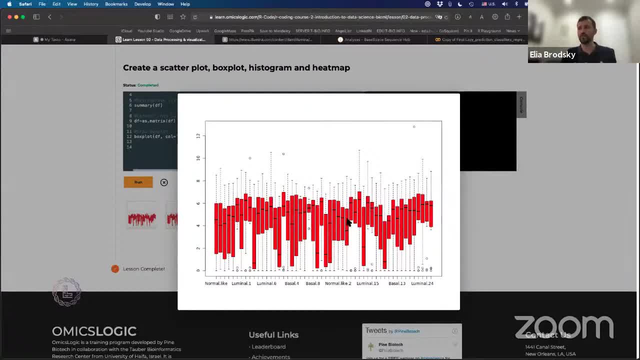 median line for each one. This gives us a sense of what's in the data. that is fairly complex. We have here a bunch of samples And inside each sample we have certain level of variability that we should be using to understand differences between the two. So let's go ahead and run it. 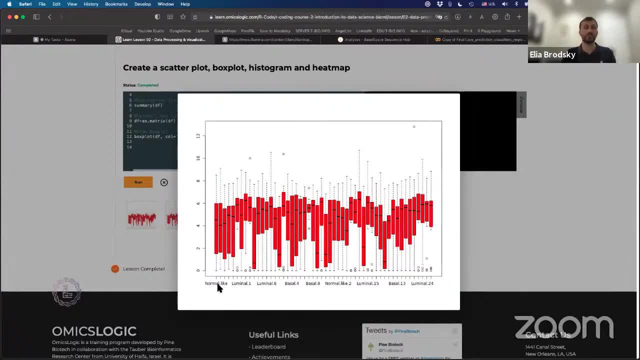 what we see right here, which is the names of groups or conditions that we're trying to interpret. Now, what's important about this visualization is that it should immediately give us a sense of how ready is this data for downstream analysis, right? So, if we want to? 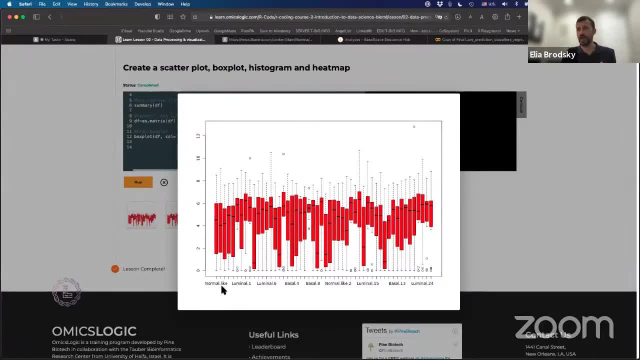 analyze a difference between normal life samples and, let's say, basal or luminal breast cancer subtypes. we want to understand that within each group there's some consistency that we can rely on to make sure that these samples accurately represent the condition that we're studying. 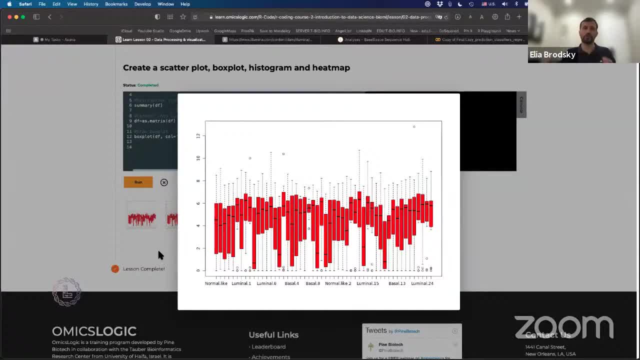 And that is really what this whole course is about. This course is going to go into the detail of the code, but also link it with the biological question that you're trying to ask to really understand what is the process of going from raw data to actual data. 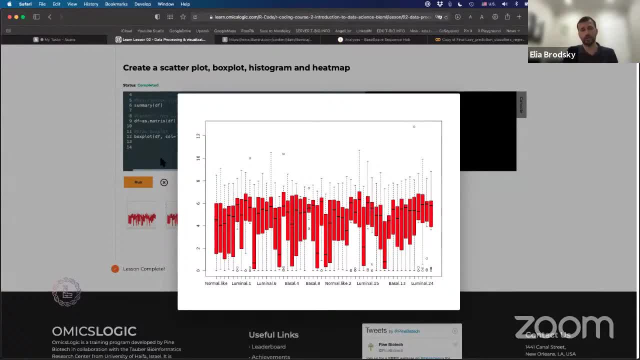 So in answer to a question that is either biological in nature, clinical in nature or has some interpretable insights for somebody working in industry like biotechnology or pharmacy. So with this I want to really make sure that it's clear that in the context of the 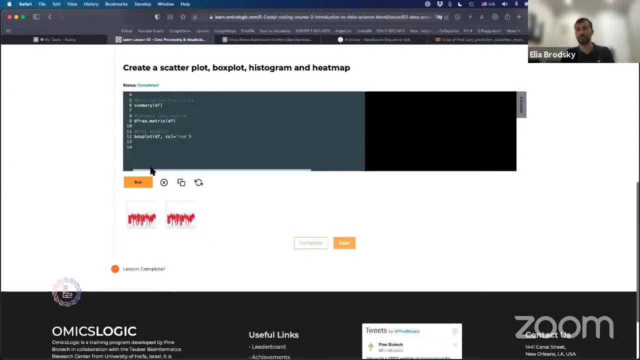 program. we will cover a lot of topics in sessions, like we did today, going through code and running examples. At the end, you will be able to see the results of the program and you will be able to see the results of the program. and you will be able to see the results of the program and you will be able to see the results of the. 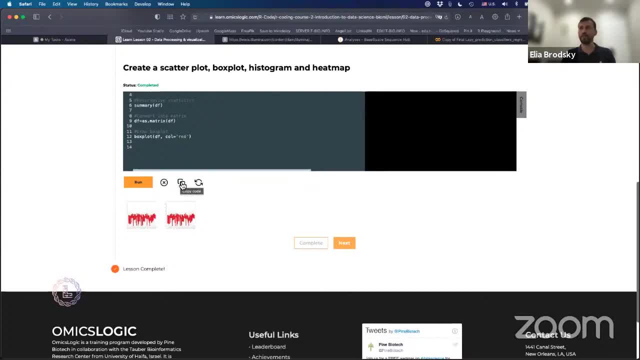 and you will be able to download all of this code. You can copy it, And we will use what's called Google Colab to make sure that all of the code that you work on is not only tested automatically on our platform, but also is reviewed by someone, so that, at the end, you come out with a whole series of 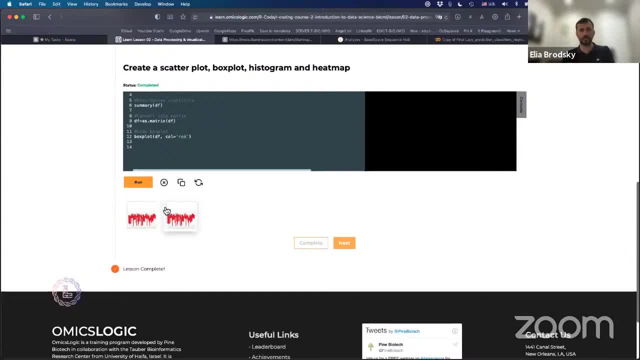 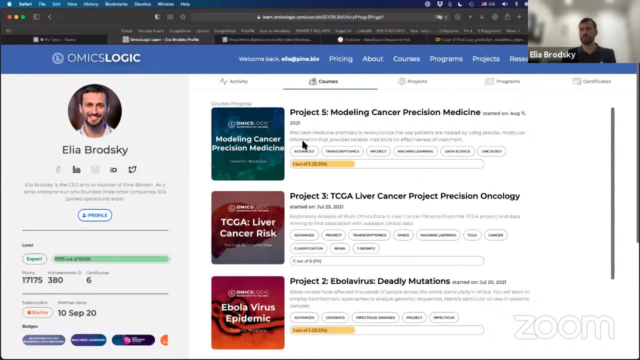 full code from beginning loading, exploration finally, to training and machine learning model and then interpreting your results. And all of that by the end of the year you're going to be able to way is going to be integrated on your own profile. so at the end, when you share your outcome, you will 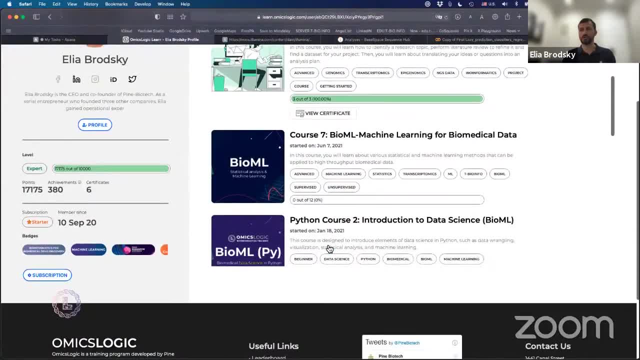 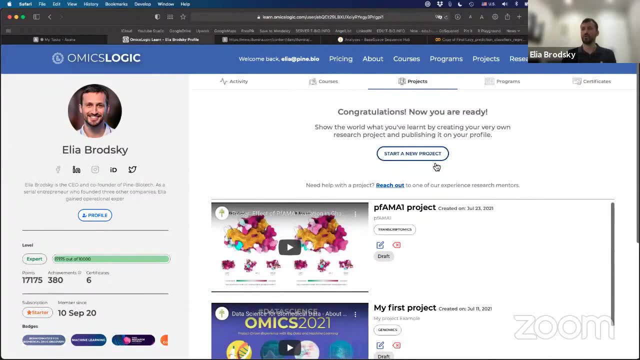 see all of the different projects and all the different courses that you have completed. you will also have the option to develop an independent project. so here, after you have a certain number of points, after you've completed the minimum requirements, you will be able to apply this to a data set of your own, essentially turning it into a mini publication that starts from: 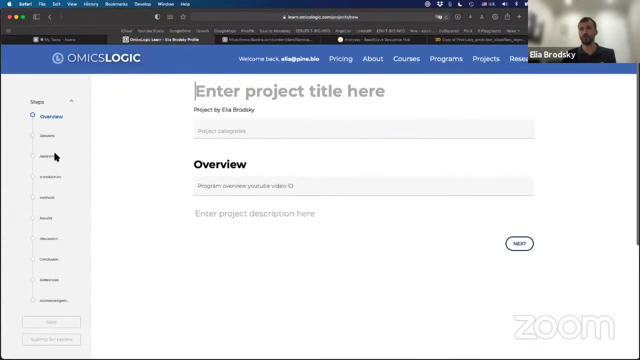 submitting this project right here on this learn portal. that will guide you through all the different steps that you need to take, and then you can actually use this to maybe go for a poster presentation or a full publication if you have a meaningful project. so with that I want to make 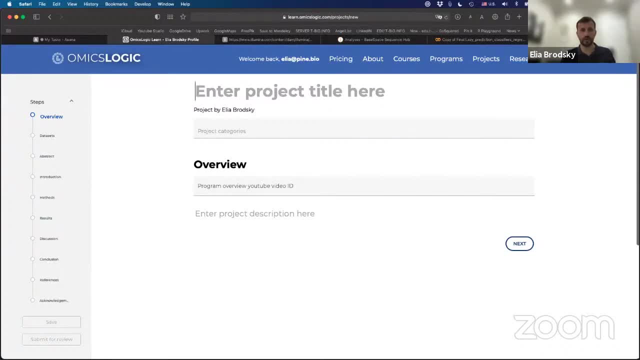 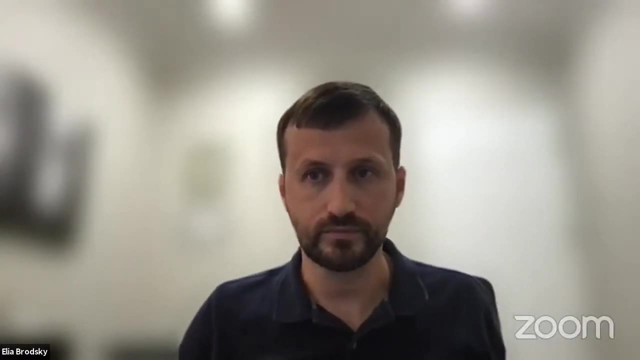 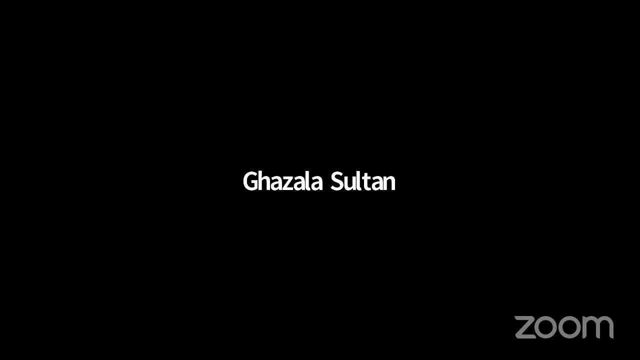 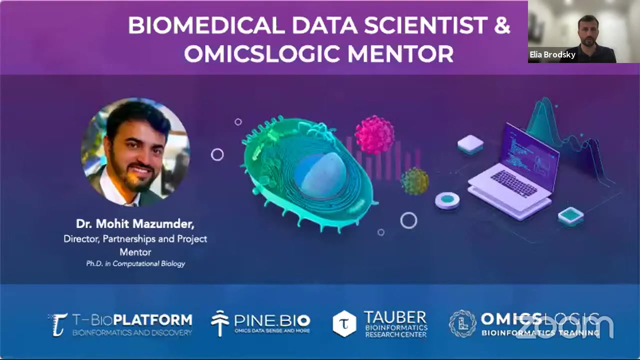 sure that I answer any questions that you might have before I pass it on to Dr Mohit Mazumdar, who will talk about the project, some of the methods that we will discover in this program. are there any questions? okay, so if there are no questions, I will pass it on to Dr Mohit Mazumdar. he's a computational. 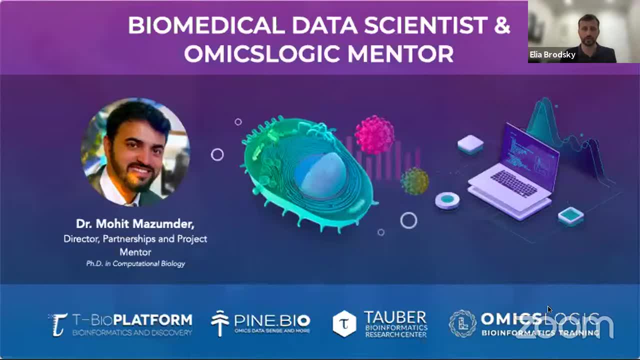 biologist and a project mentor here with omics logic, and he will talk to you a little bit more about the curriculum, how to sign up and where you can find all the information. over to you, Dr Mohit Mazumdar. yeah, am I audible? yes, you're audible, thank you. hello everyone. my name is Mohit Mazumdar and I am a bioinformatician. 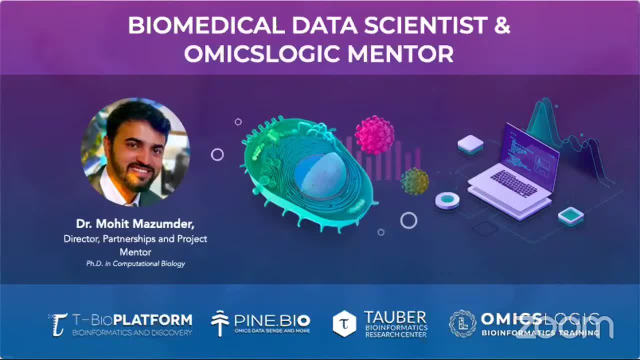 by education, and since last 12 years I have been practicing and applying bioinformatics for research projects, now both for student-driven research projects and academic and industrial collaboration. so during my Phd I learned to apply machine learning algorithms to variety of sequence based data sets and were able to design and complete several research projects that are now published. 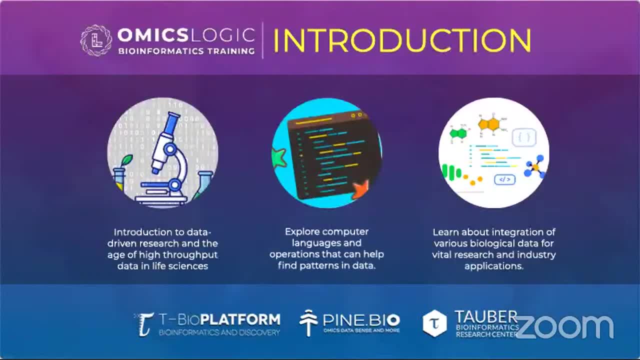 in peer-reviewed journals. so with this incredible growth, I think big data has turned out to be a remarkable career choice for many. today, industries from various disciplines to various fields of the domain offered different positions for big data professionals. that includes biology and healthcare, too, So some of the topics that we are covering in this program are quite 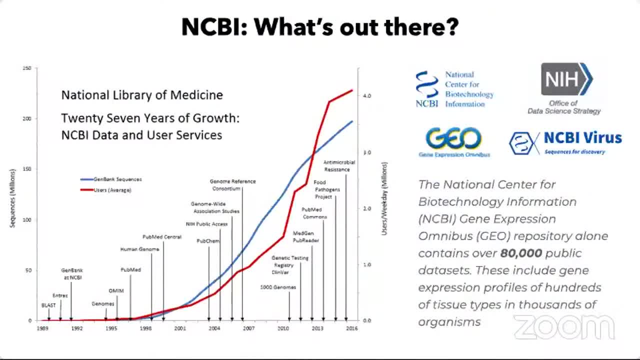 relevant to the industry. So, from a data perspective, I think we have already heard from Ilya a lot about it. So what I think is what makes biology unique from other realms is its sheer size. So I think that, for example, like, for example, if I have to give you an, 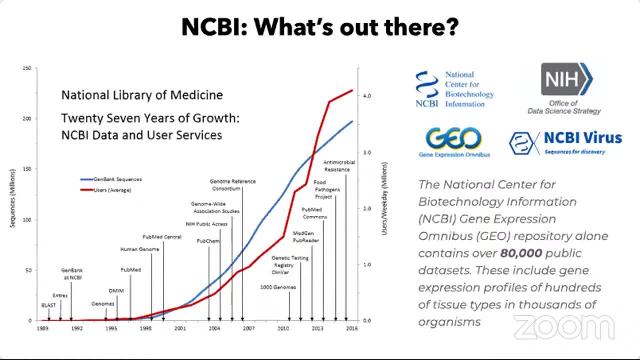 example, a typical genome of a microbe which might have 4000 genes And if we assume that there are like 1000 meaningful distinct variants for each gene, then that's like almost 1 billion samples to test. So I mean, if you, if you consider that sort of volume of data, it's really 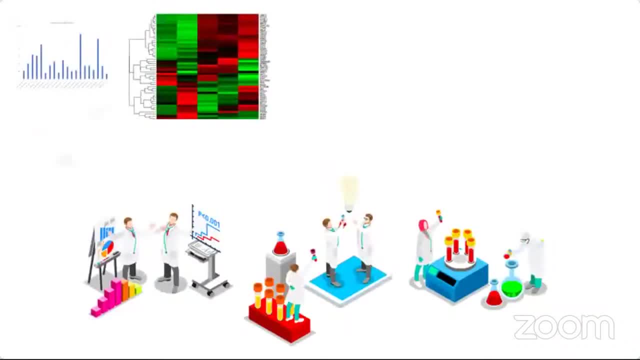 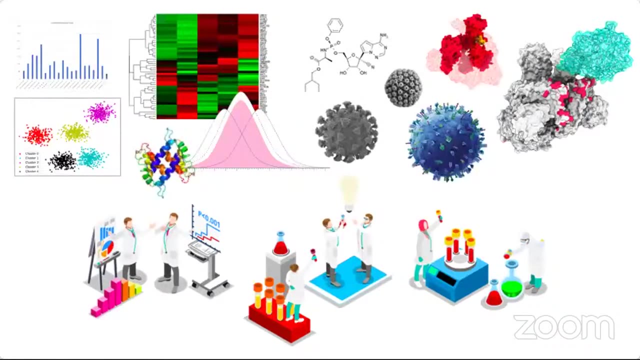 really really very big. So genomic researchers: they utilize bioinformatics to speed up research related to analyzing DNA sequences, ultimately helping inform teams looking to combat a given disease. So COVID vaccines and cancer research are two areas of genomics that is greatly helped by bioinformatics. Similarly, in the case of drugs as vaccines and future cancer. 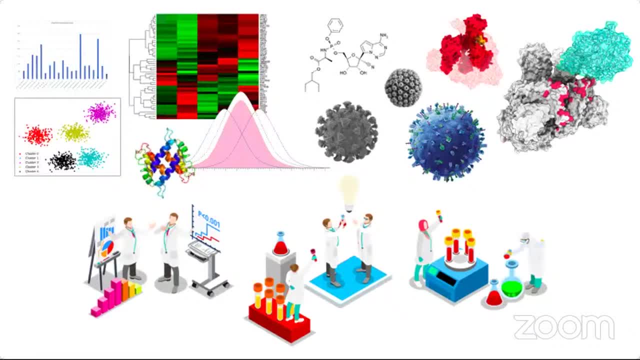 treatments. current pharmaceuticals can also become more efficient, and they are, you know they are moving in the right direction, with almost instant analyzation capability afforded by bioinformatics right And machine learning. machine learning helps to make databases more searchable and trackable by biologists whose human understanding and instincts are paired. 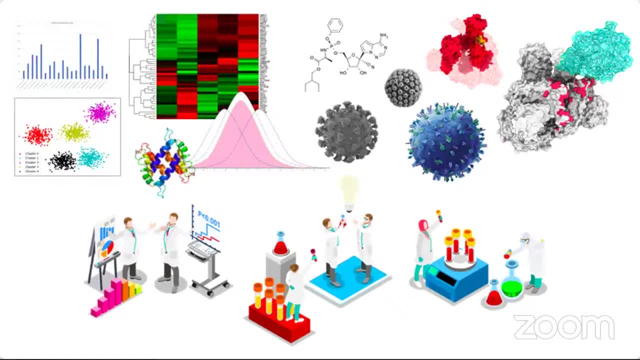 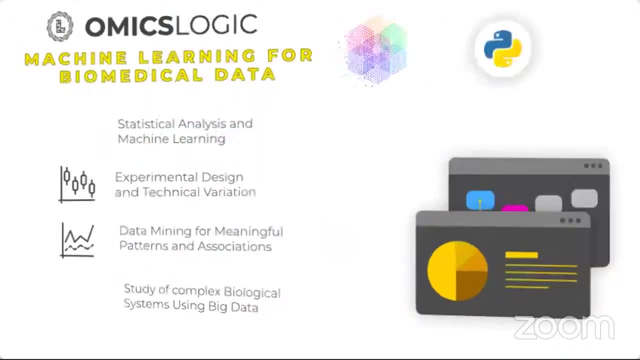 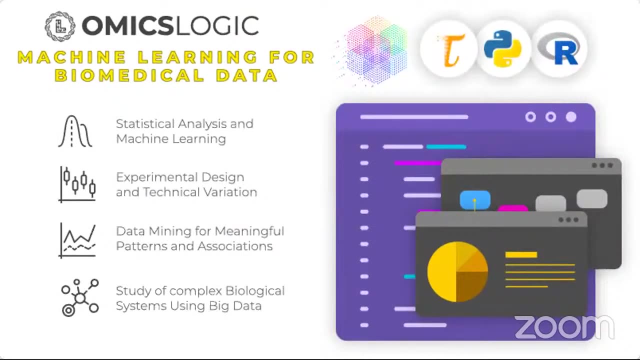 with power of AI and that power of AI can create a kind of an investigative ecosystem. So that's something that we all are looking forward to About this program. I think our team and industry within our team and with our industry and academy collaborators contributing and developing this unique program that takes 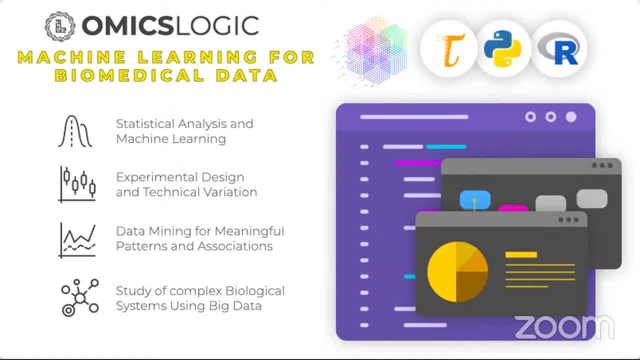 you through the omics logic learning experience and provide hands on training through the powerful HibaInfo platform. So let me tell you about the intended outcomes and some of the learning objectives of the program. So some of the things that we will be doing is that we will be learning about the terminologies. 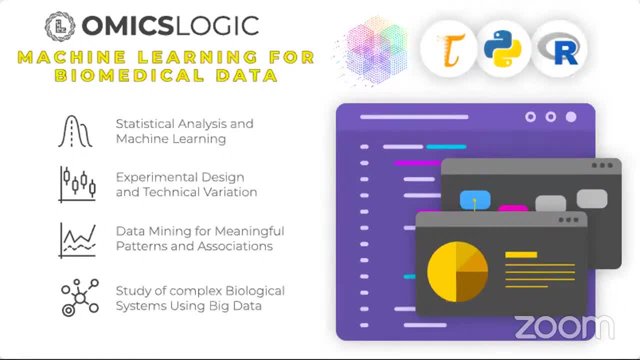 for machine learning and artificial intelligence in biomedical discovery. we will be understanding the analytical methods for processing, visualizing and analysis of complex biomedical data. We will be understanding the machine learning taxonomy and also the commonly used machine learning algorithms which are used to analyze different kinds of biomedical data. 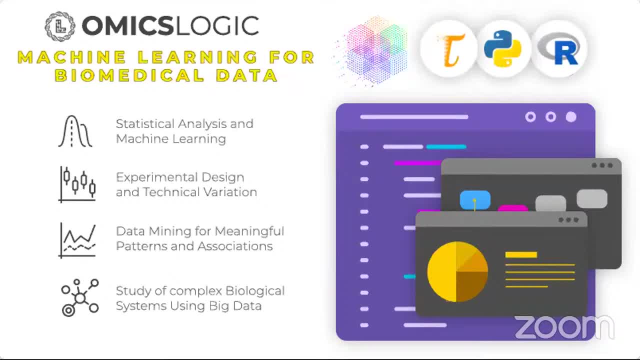 We will have hands on practice in application of standard unsupervised and supervised machine learning methods to various types of data, such as genomics, transcriptomic metagenomics, imaging data and clinical data. You will be becoming familiar with project examples where machine learning was used effectively. 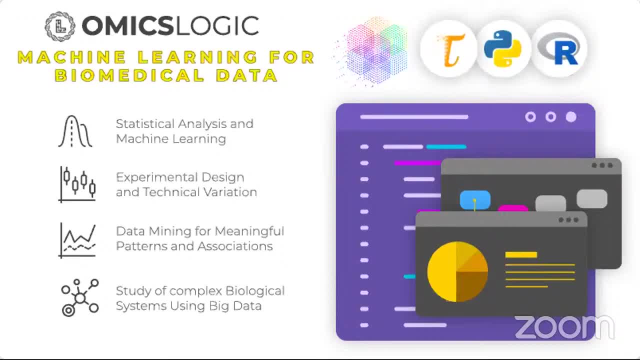 to achieve meaningful results, And then you'll be able to understand differences between machine learning categories, I mean categories of algorithms in different machine learning algorithms on different category, which would be like what kind of data sets they are good for, what kind of problems they are good for and they are applied to, and then we will understand about. 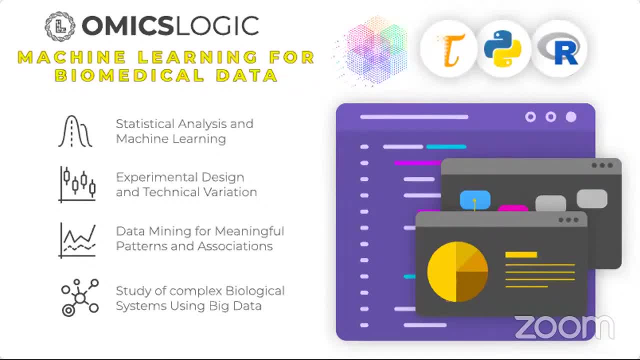 different applications of machine learning in the aspects of project design, uh objectives, and then we will learn about python packages for data visualization and analysis of uh and and using analysis using machine learning methods by python and then apply machine learning techniques to analyze public domain data or in your own data set. so those are some of the things that are. 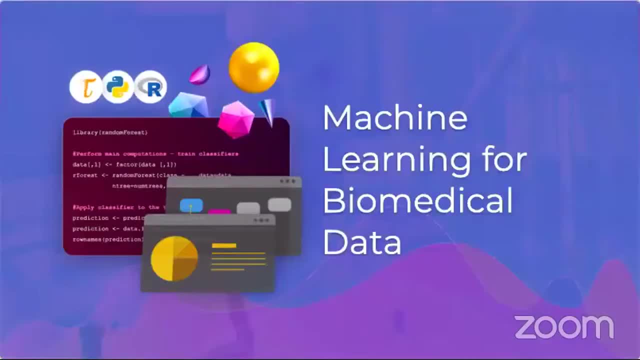 intended to come out of this program. so this course and this program is designed as a combination of online resources. then there will be practical assignments and there will be live sessions, live workshops that will be conducted through zoom and throughout this program we will review several project examples that demonstrate the success or the limitations of conventional 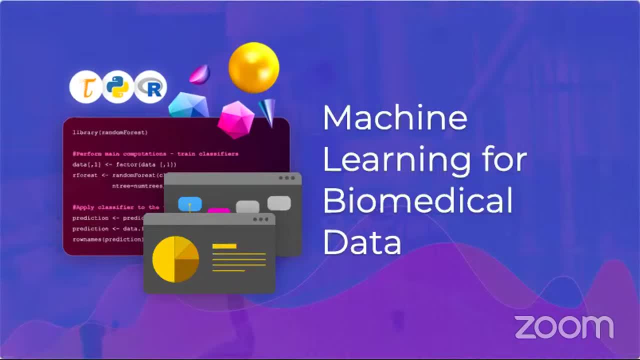 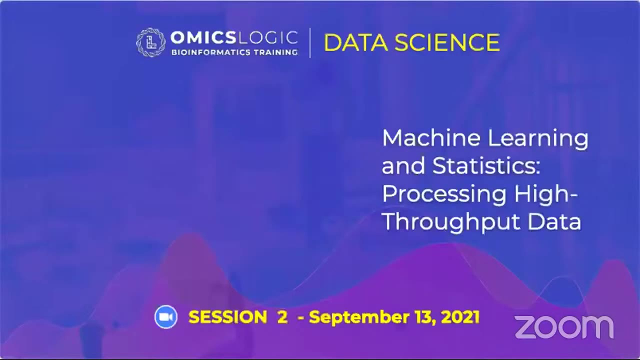 machine learning methods and also deep learning methods using data from public repositories. okay, so now let's uh go to the sessions. that what sessions will be the next? so i would wanted to give you an overview of what is coming next. so, in the next session. uh, that will be the second. 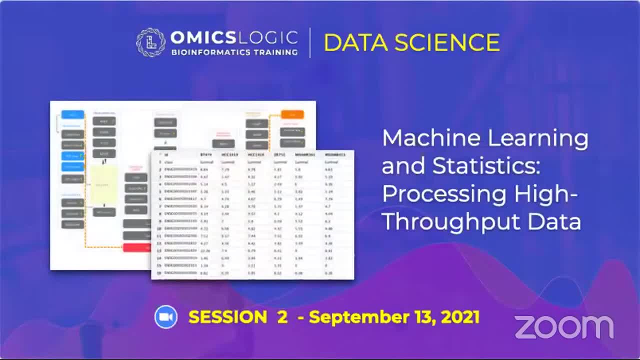 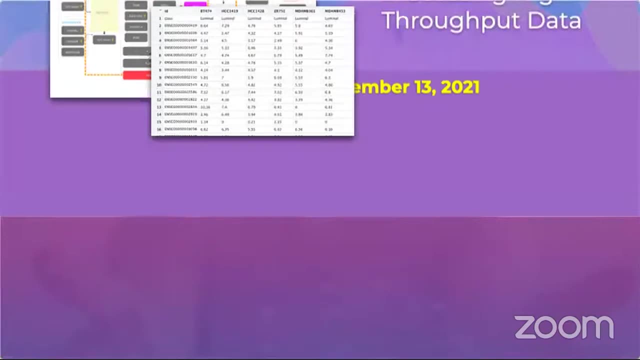 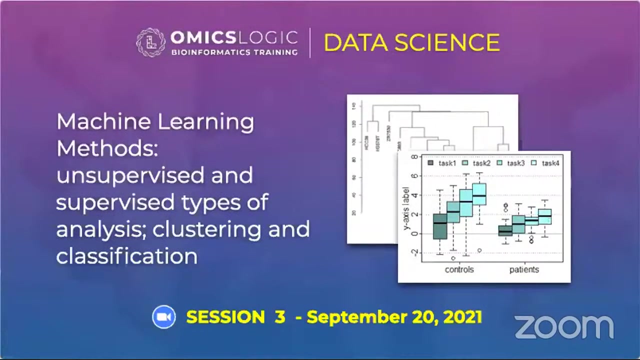 session uh, we in this session we will learn about various omics- data that are generated through high throughput technology and contains detailed information, for example genomics, transcriptomics- and then we will learn about the overview of approaches and we will learn from used use cases for various types of machine learning algorithms for clustering and classification. 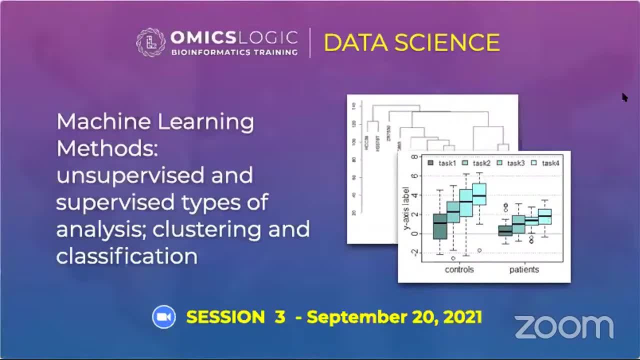 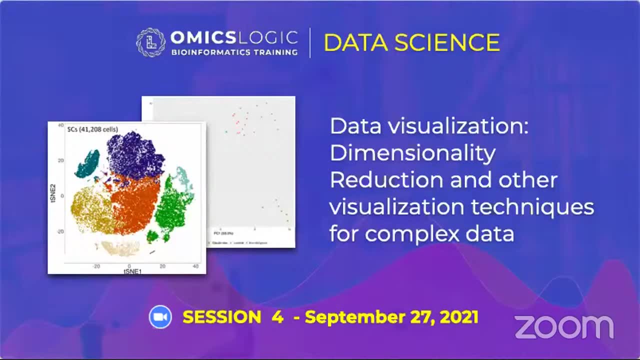 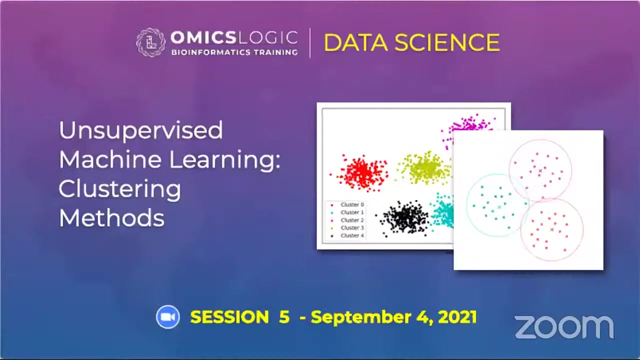 to visualize and interpret multi-dimensional data. the fourth session in this session we will overcome some of the challenges to compress complex information into an interpretable representation- visual representation- accurately. and in the fifth session in this session we will learn about the very critical challenge to organize data using complex patterns in a space that is beyond human imagination, and we will be in 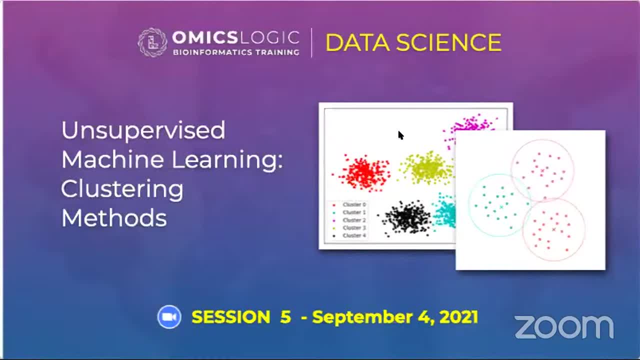 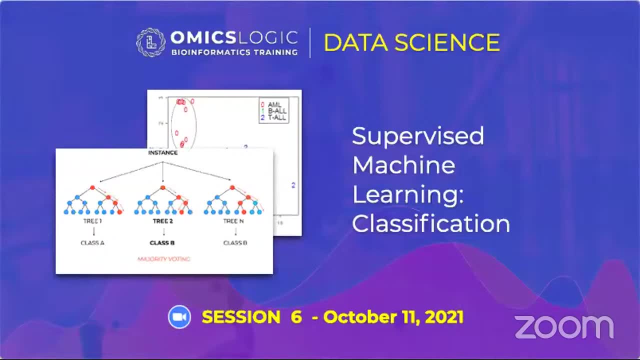 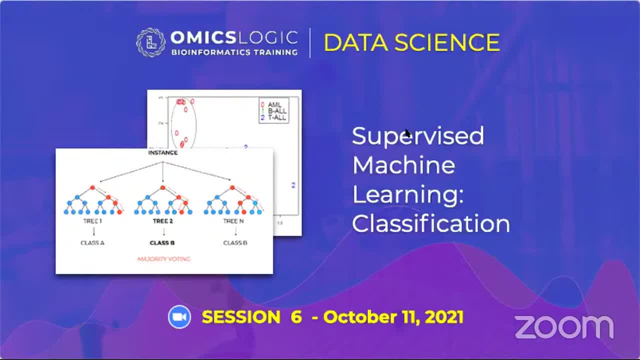 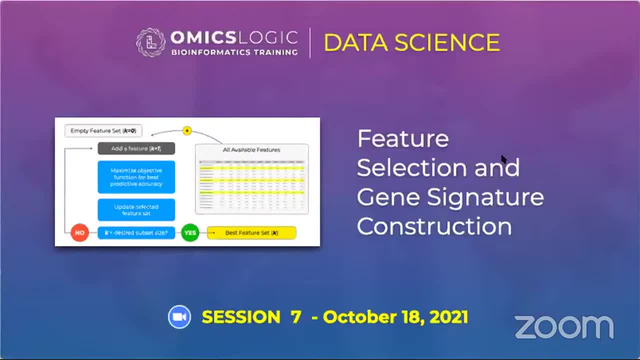 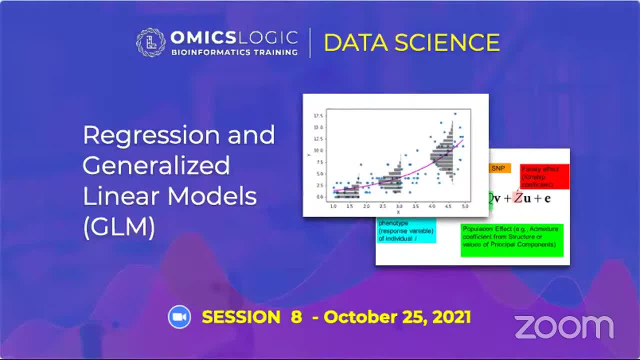 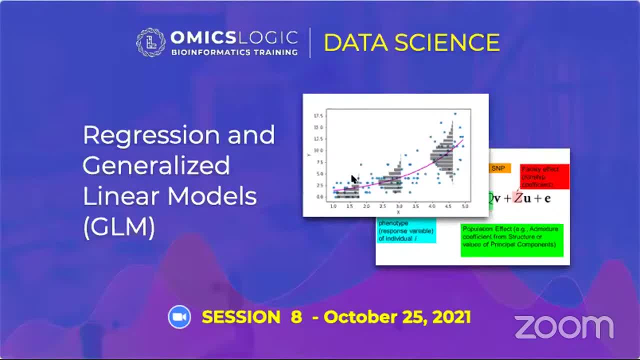 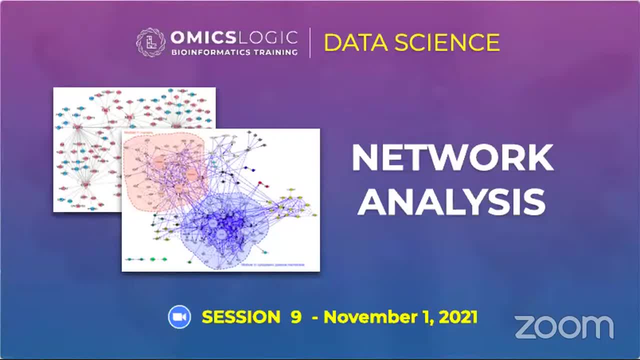 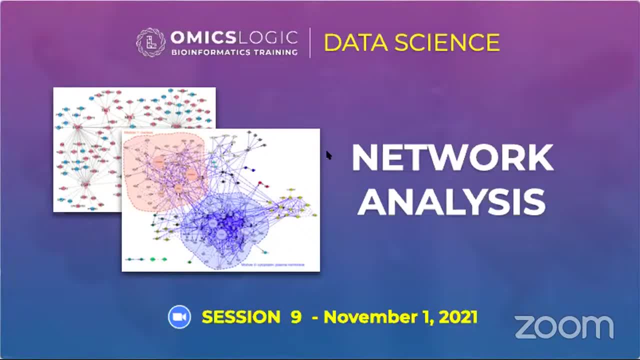 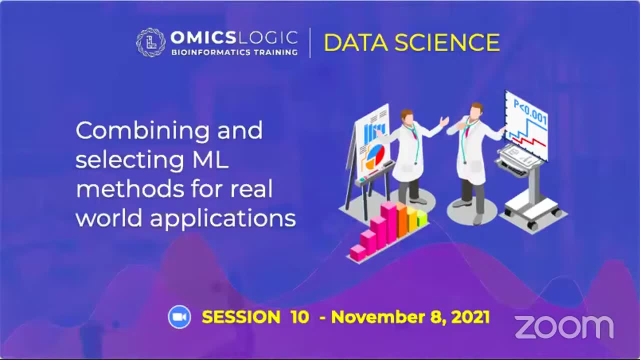 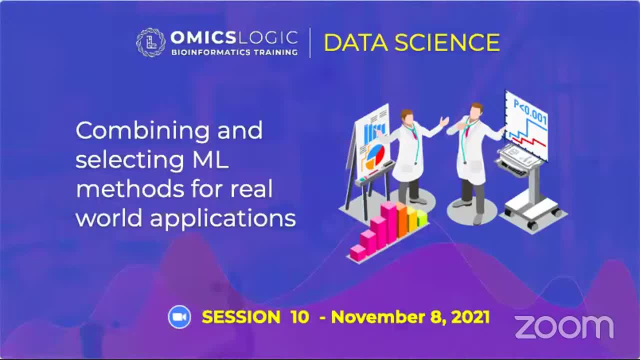 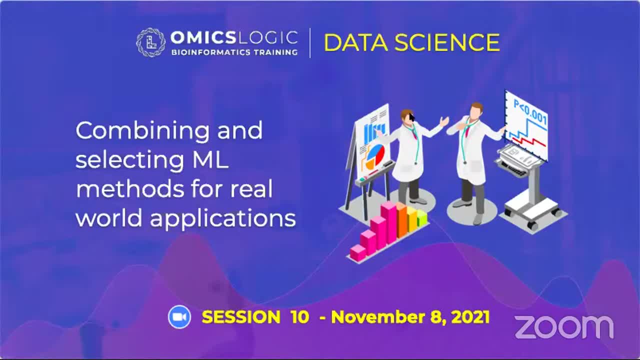 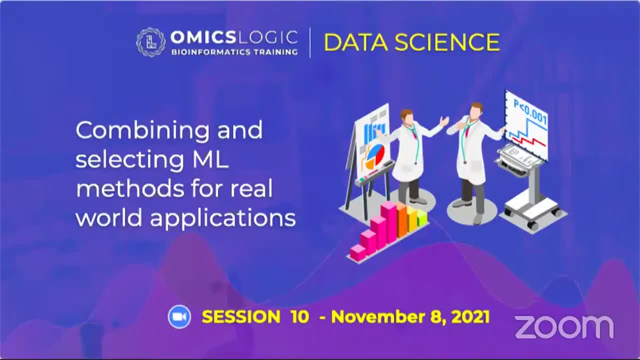 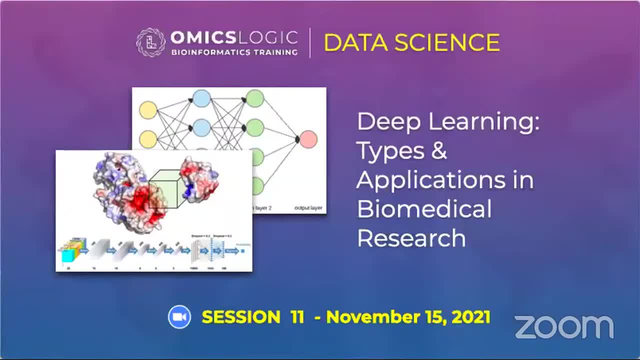 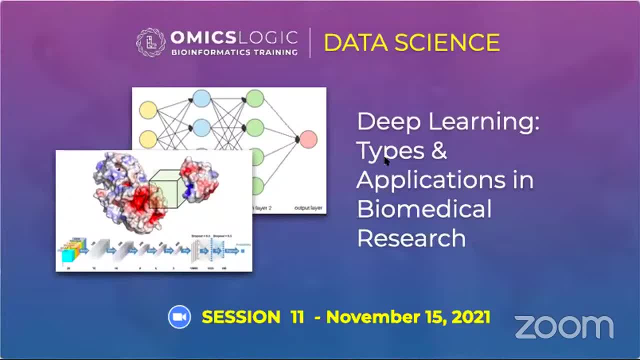 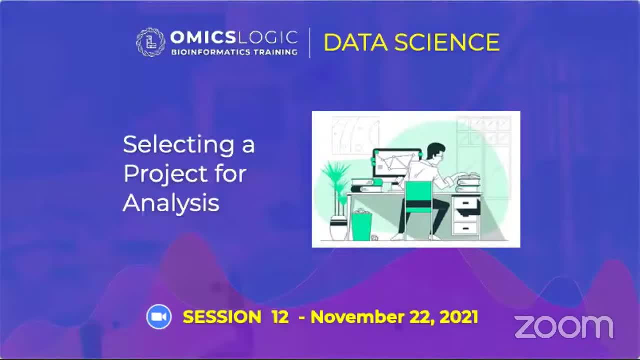 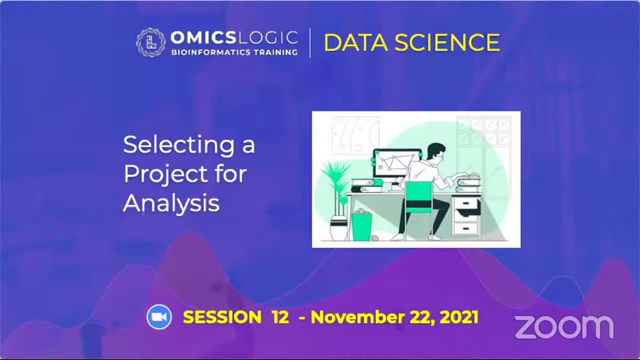 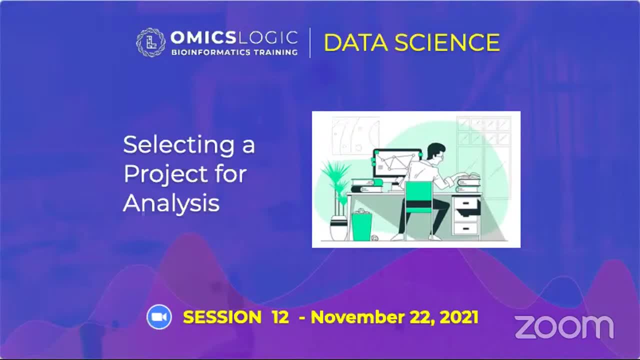 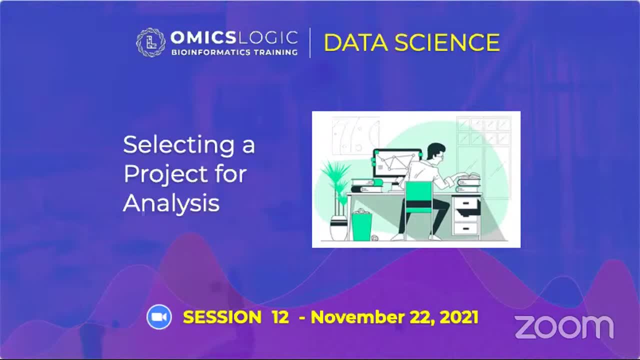 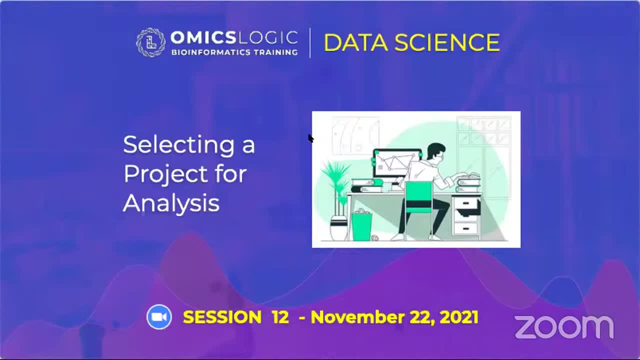 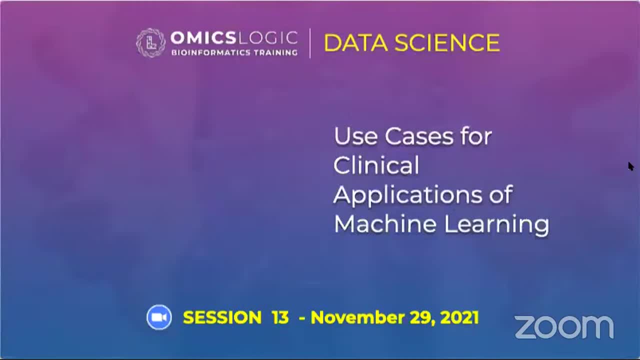 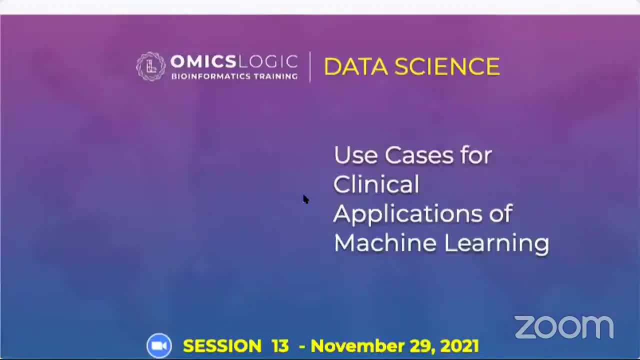 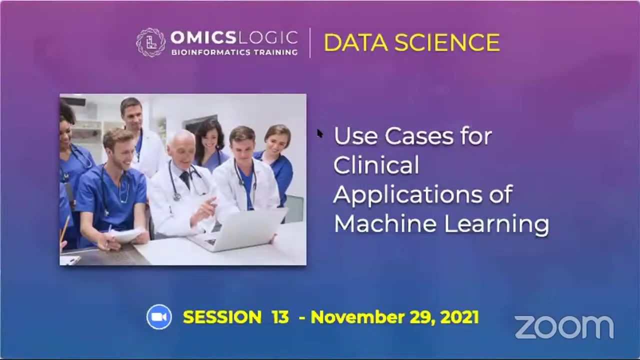 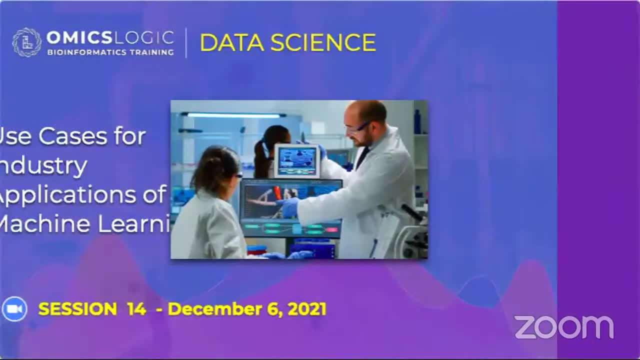 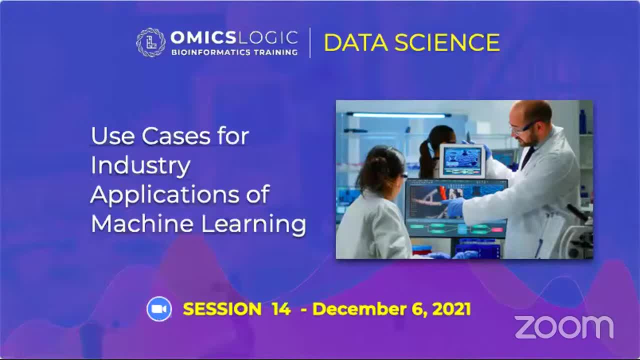 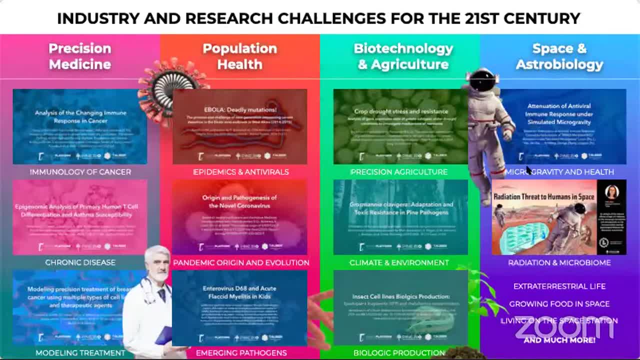 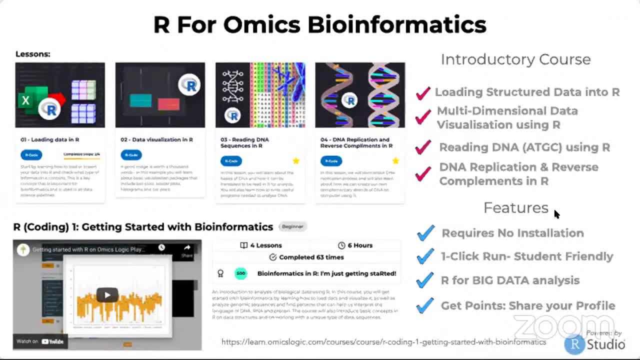 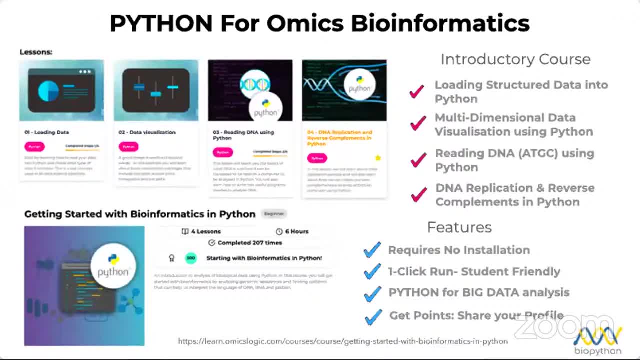 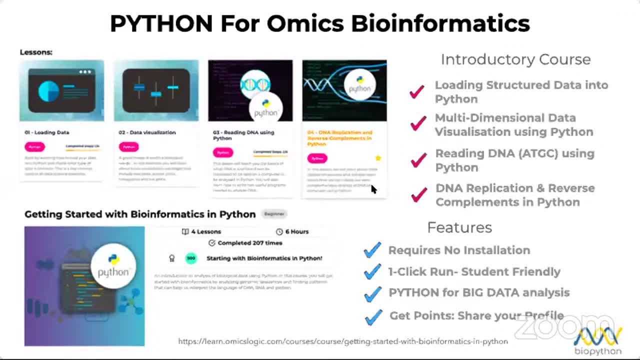 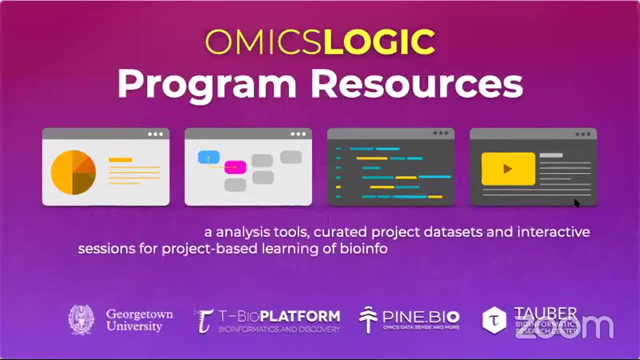 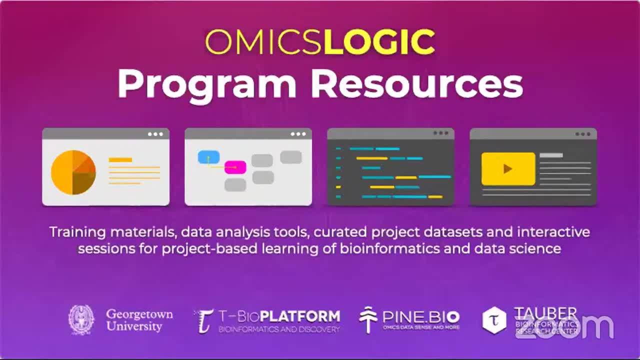 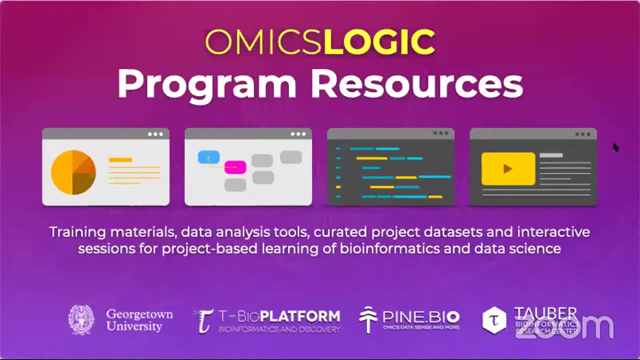 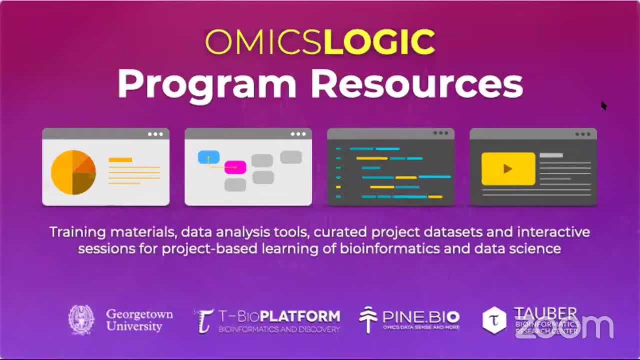 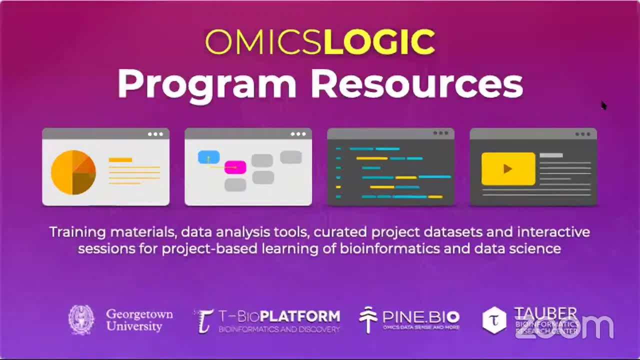 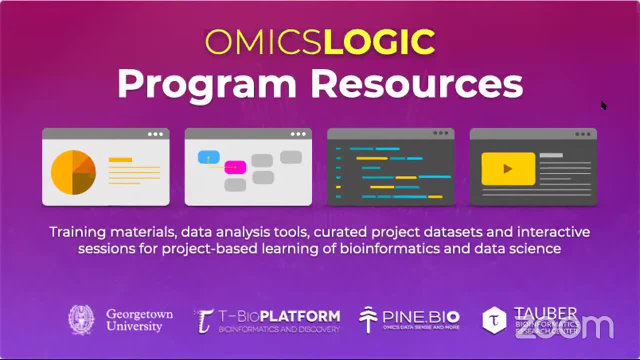 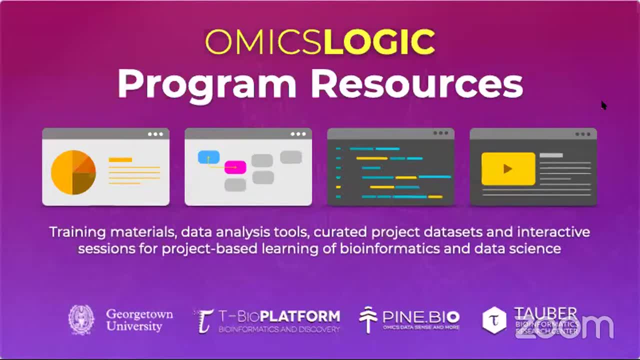 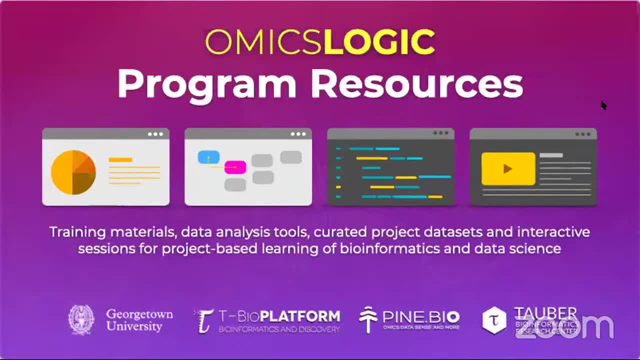 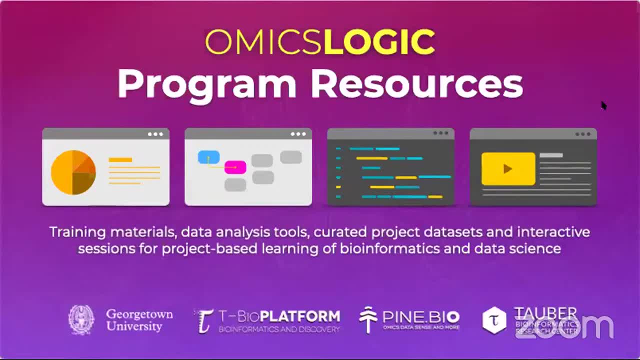 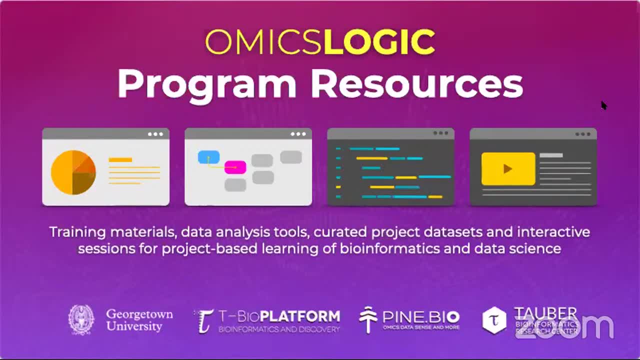 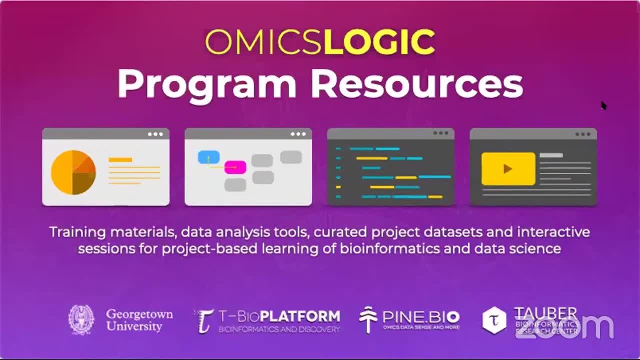 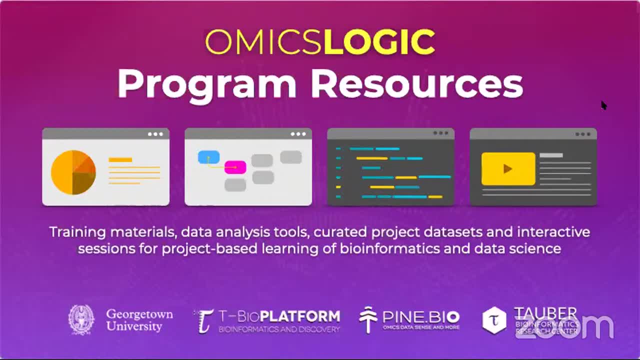 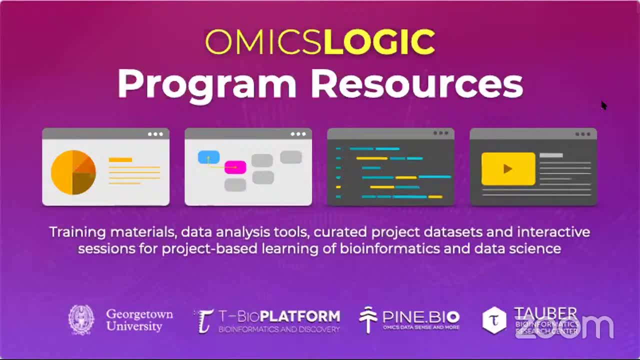 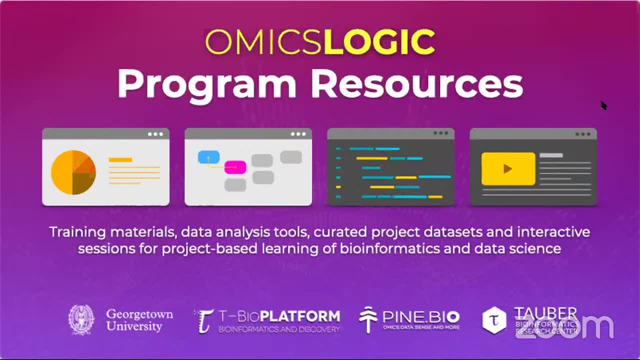 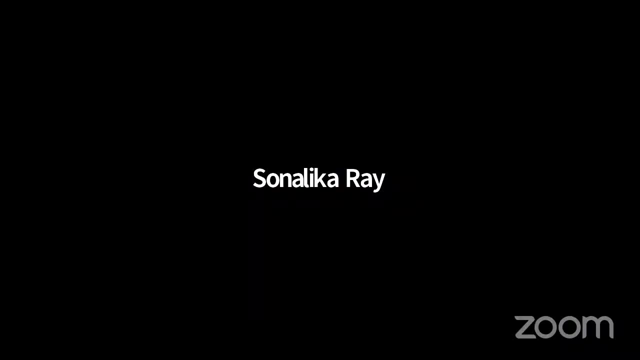 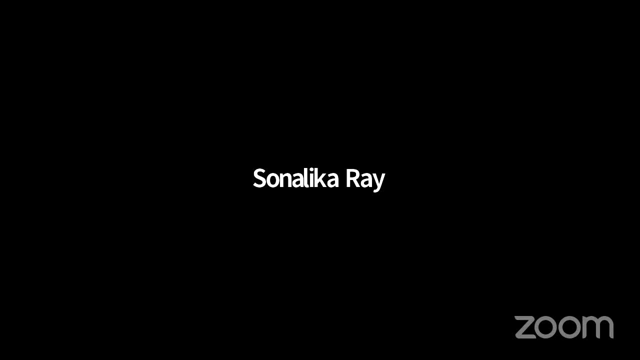 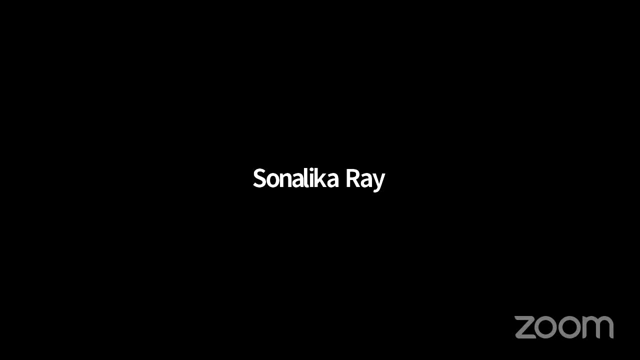 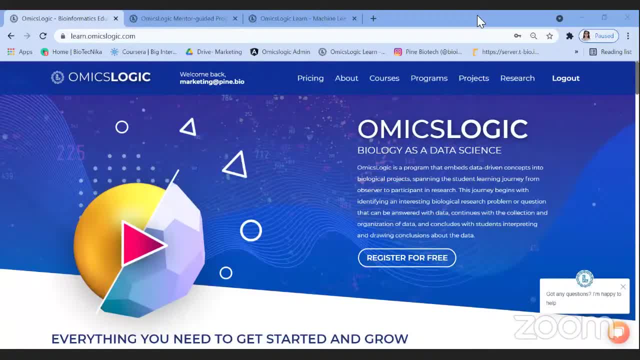 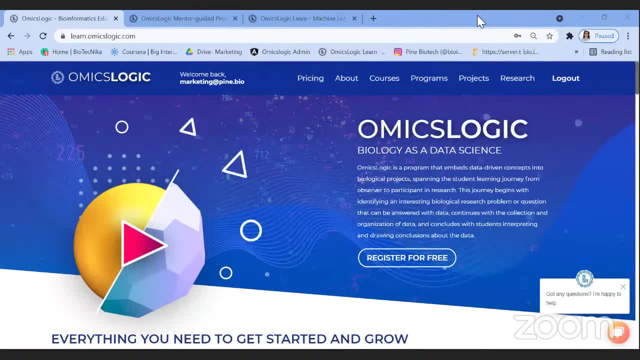 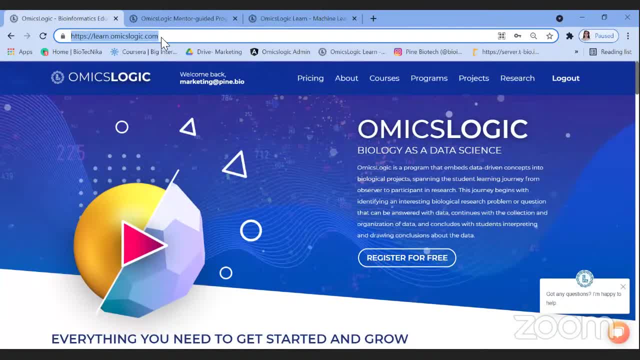 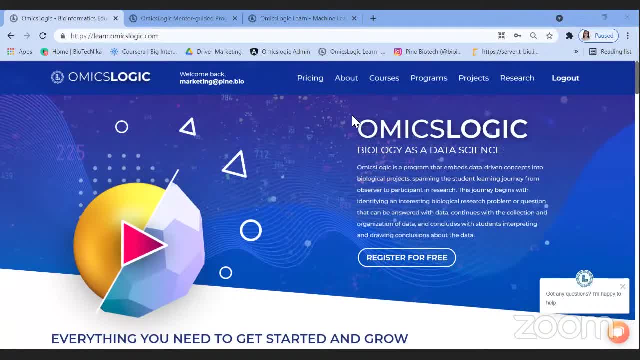 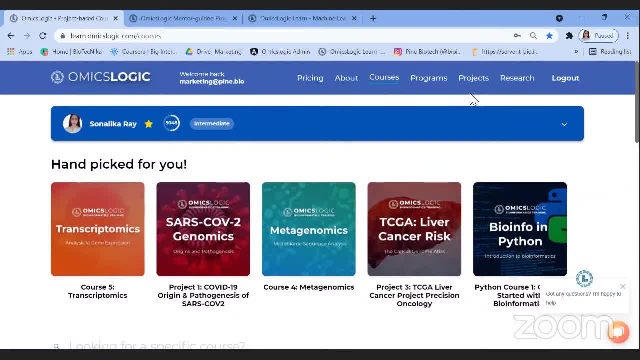 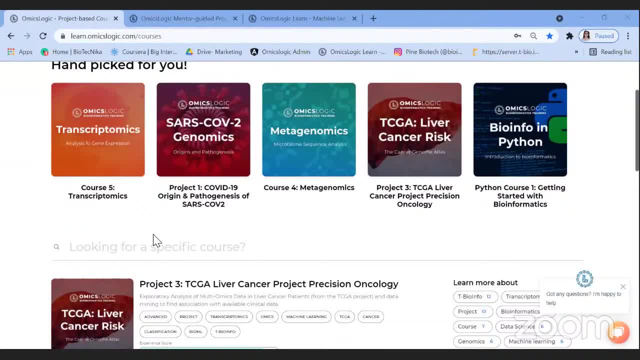 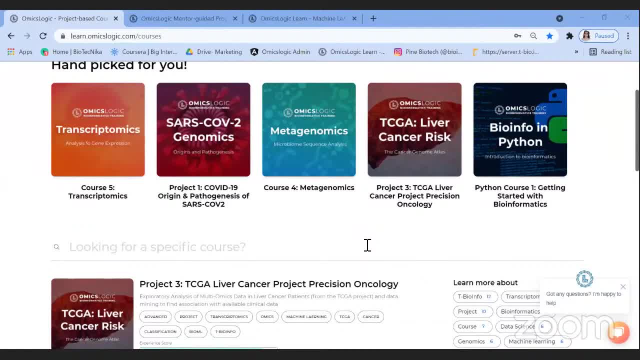 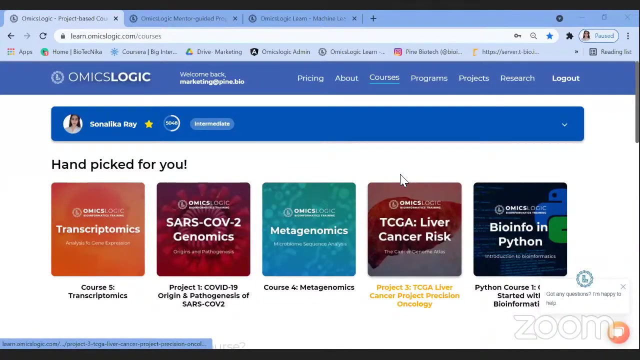 learning about the application of supervised machine learning for classification in this session. we will be learning about the application of supervised machine learning for classification in this session. we will be Okay. thank you everyone for casting your vote. I'm just ending the poll now. So once you are here on the omics logic portal, you would be able to find few bars here, as 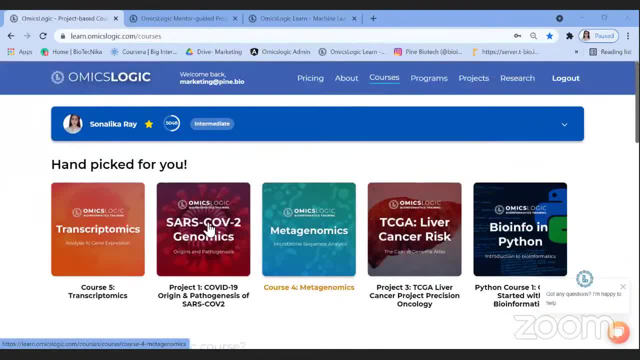 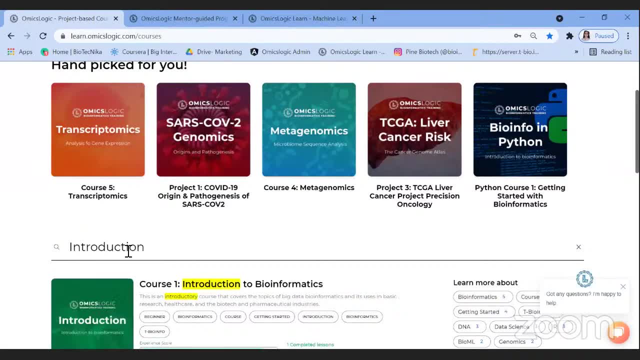 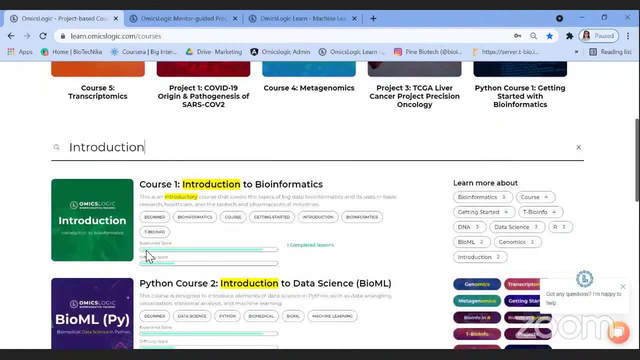 courses, programs, projects and research. Go to the courses tab and just type introduction and you would be able to find a lot of introductory courses. So if you are new to bioinformatics, let's say you are from a biotechnology background or microbiology or biomedical, and you have 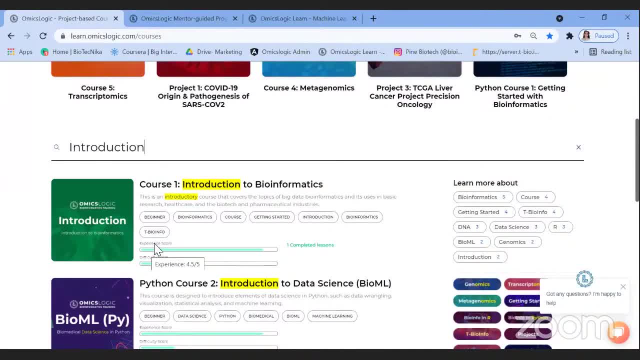 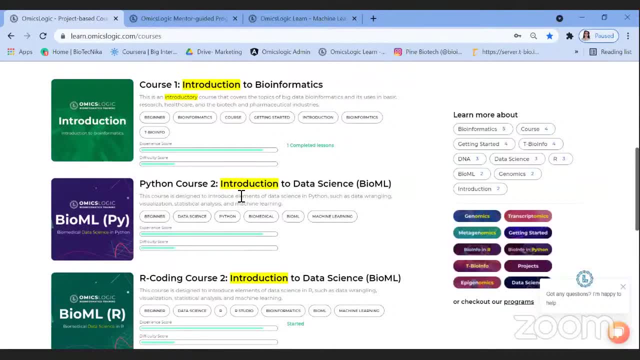 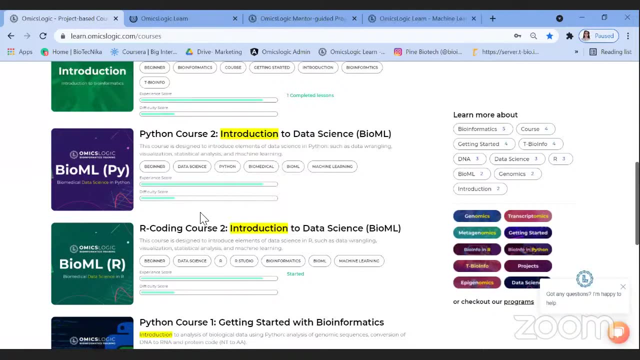 no clue of what bioinformatics is, but you want to begin with that? then make sure that you go through and explore this course: introduction to bioinformatics. We have various introductory courses on R and Python as well, So let's just go through one of the introductory courses. 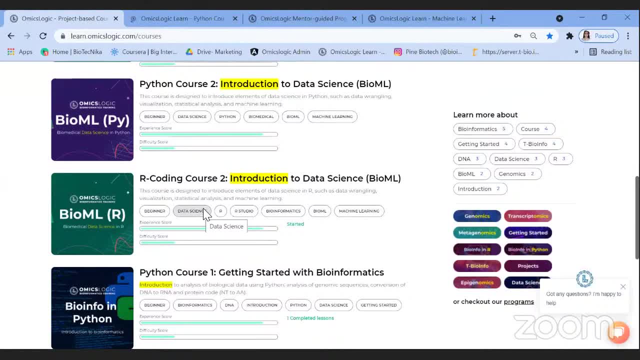 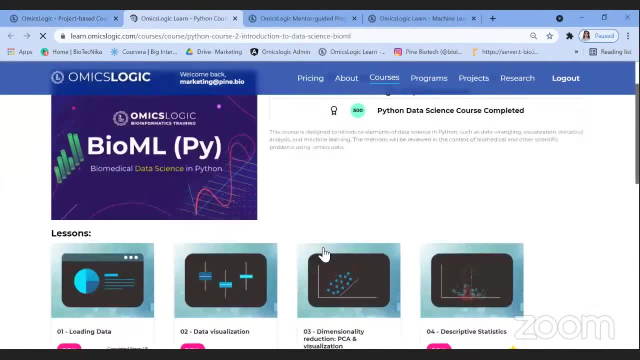 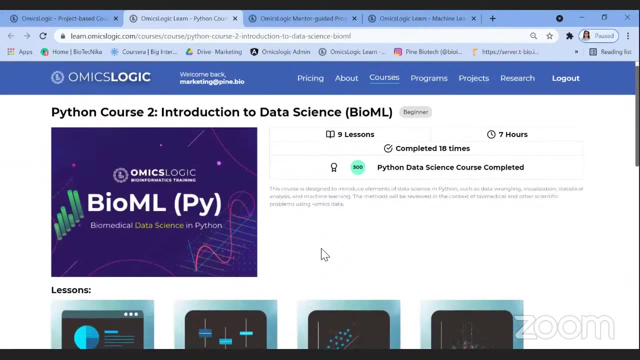 You can just begin with introductory courses and then have the basic knowledge, and you would definitely be able to go along with all the session material there. So these are a few of the lessons which are there. in the course of introduction to data science for Python, You could also practice each and every code. 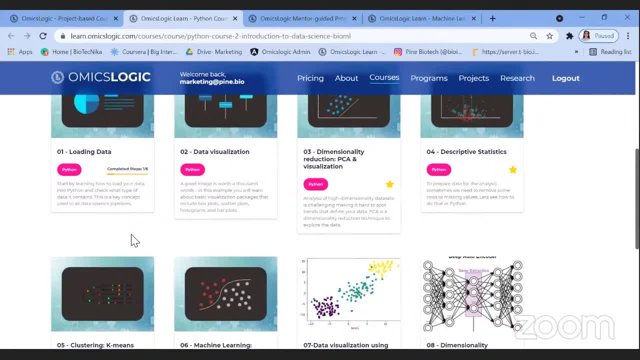 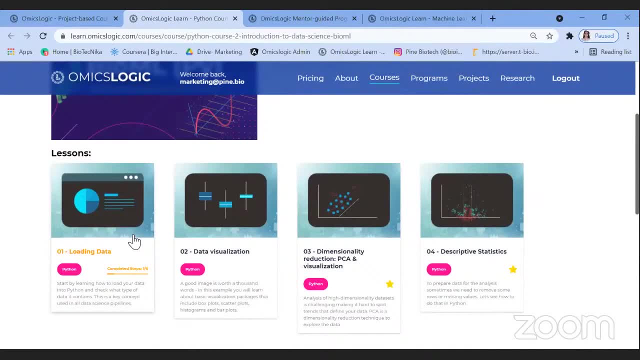 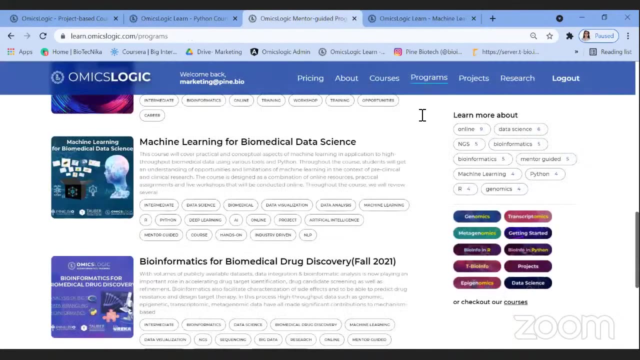 block on the console- It's like Ilya showed you- and help you practice with few of the stuff, So you need not install any Jupyter notebooks and stuff, but actually just learn the code and practice it then. and there Now coming to the program page, how you get to the program page and how you register. 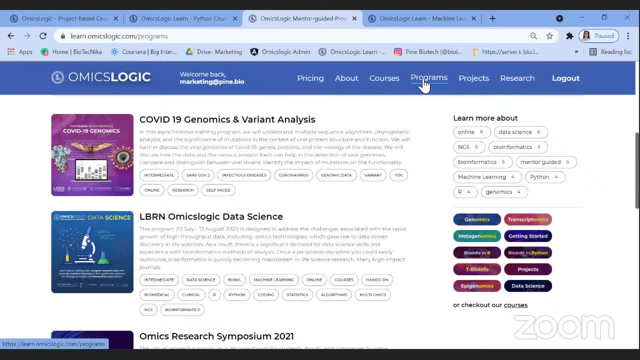 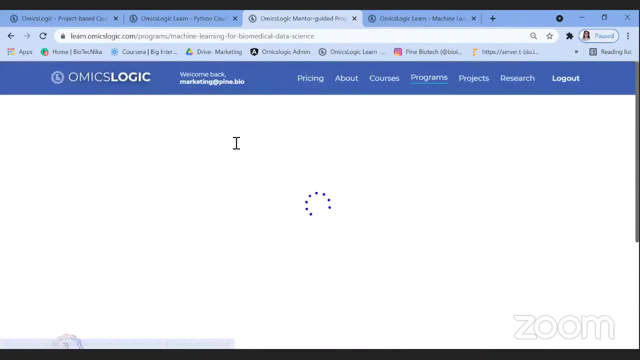 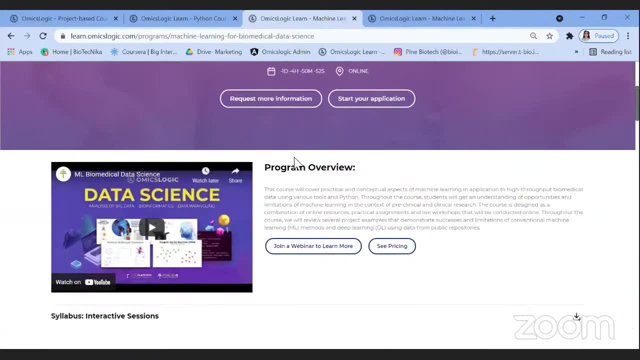 yourself for the program. So visit the programs on the omics logic learn portal and just find the program that is machine learning for biomedical data science. Now, once you are here on the program page, you would be able to find all the details that are related to the program, and also the schedule of the program and the session topics. 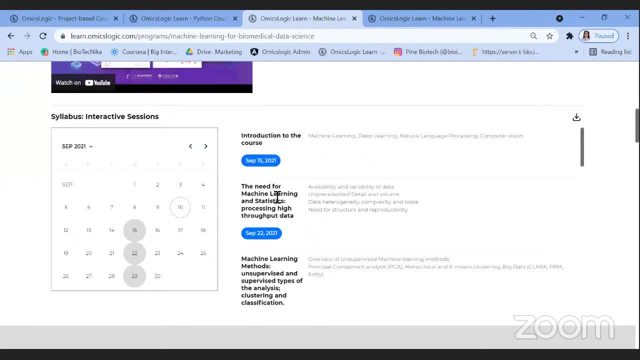 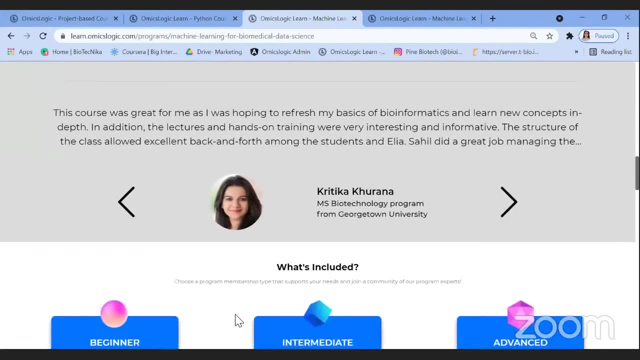 that are going to be covered on various dates for the program, the title and also the topics that would be covered. And once you scroll down, you would be able to find three levels that are beginner, intermediate and advanced. So the beginner, intermediate and advanced. 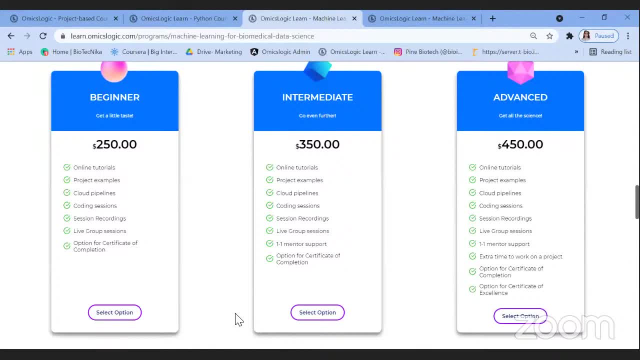 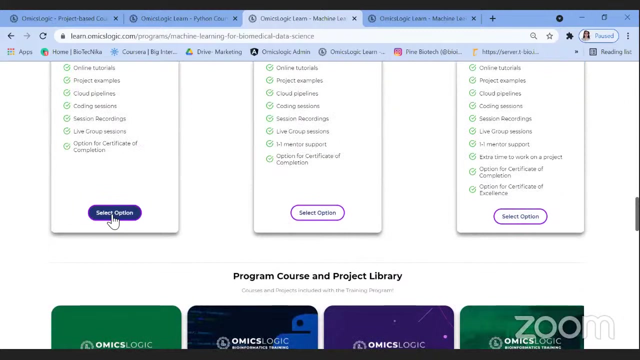 advanced levels. Now, these levels are being divided just based on the prerequisites that are being provided for these, each different levels, And you can enroll yourself for whatever level you want to be, based on the facility that you would like to gain from the program. You just have to click on the select option and proceed with your payment checkout gateway. 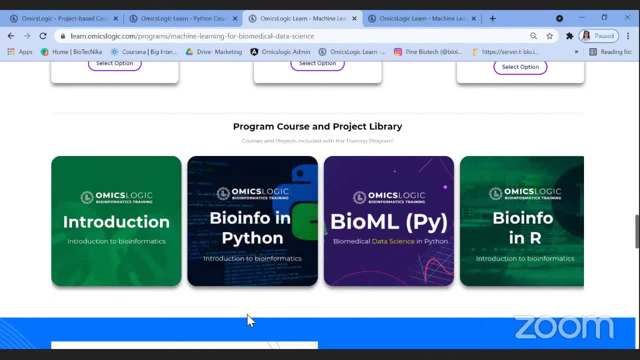 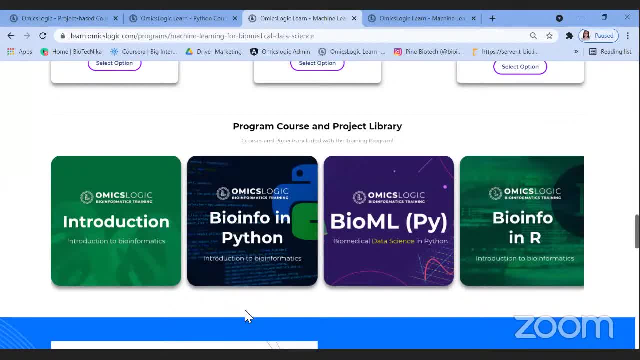 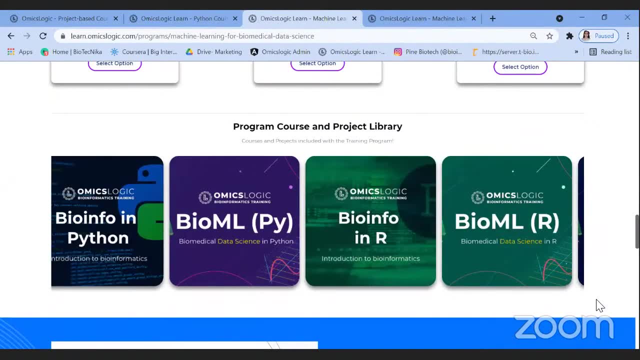 Okay, So again, all these lists are here. Don't forget to scan So you do see the arrangements here in the course tab where all the courses that are recommended to complete for the program And also you would have the access to each and every program here. 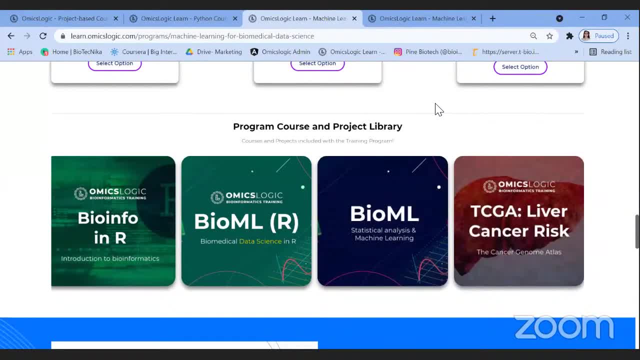 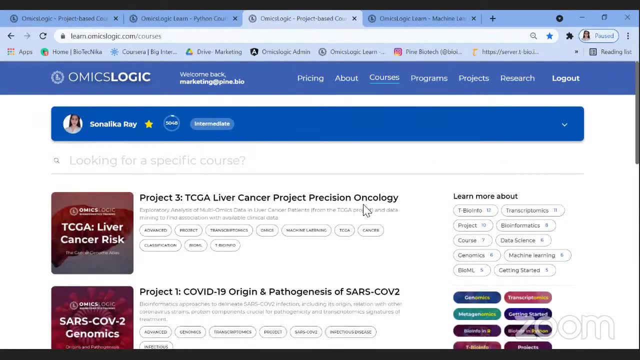 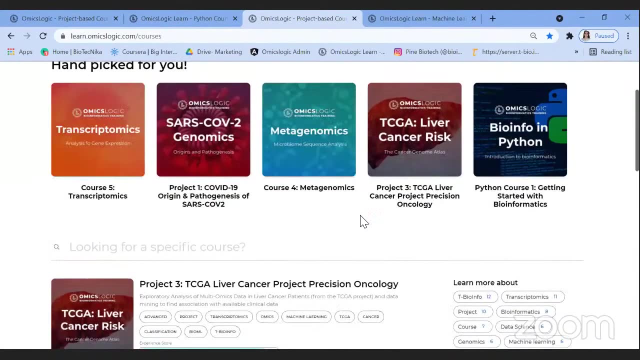 the introduction program by Enfer and python, by R and bio, ML courses- that as well- where you will learn about statistical analysis and machine learning. I also. we have various could be applied to solve a research problem and then how you analyze or interpret the results. 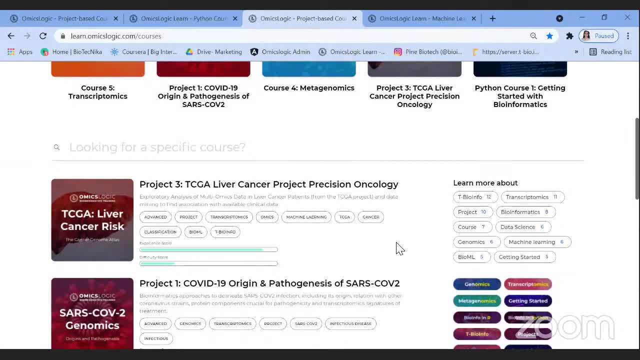 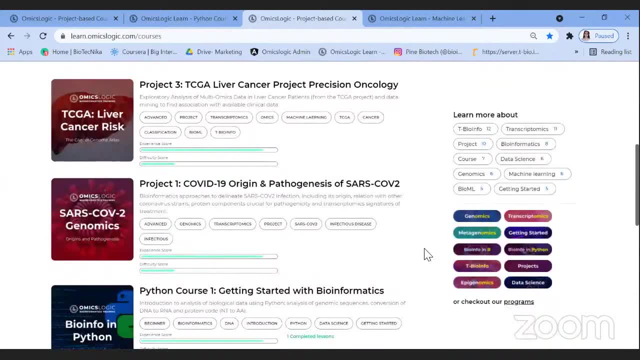 from the server. so now let me just take a minute to help you navigate how you have to reach to various projects that we have and also the courses. so if you wish to view the courses that are available under the courses tab on the learn portal, just click on the course and you would. 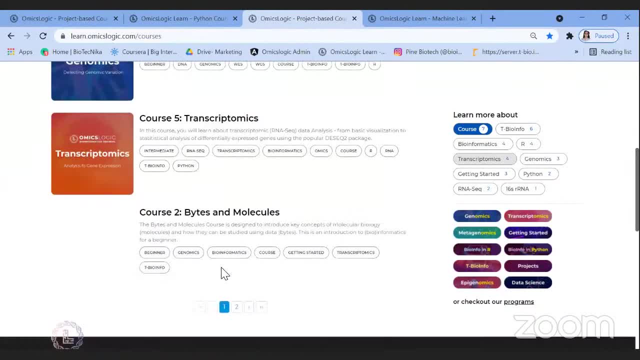 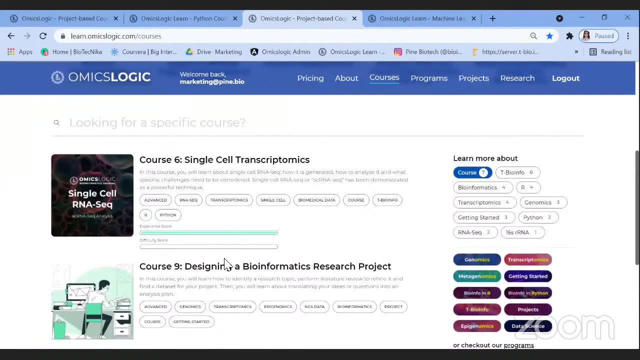 be able to find all the courses that we have. so i was just talking about the bio ml course. i would really like to take you through that as well, and those who are want to carry out a research project, a bioinformatics research project, but come from a different field, they can definitely take up this. 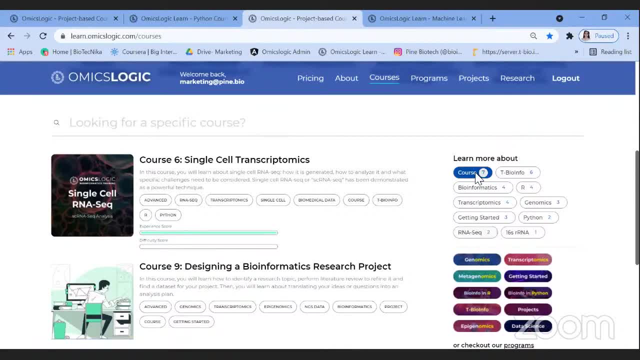 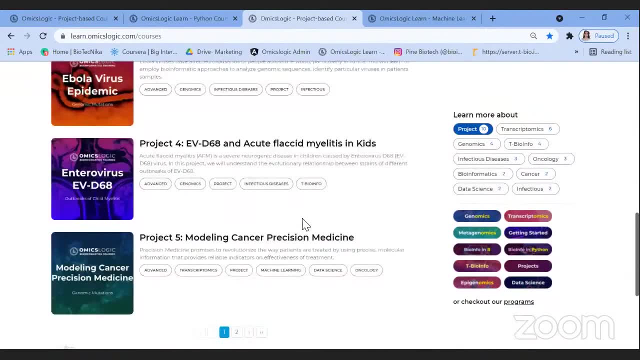 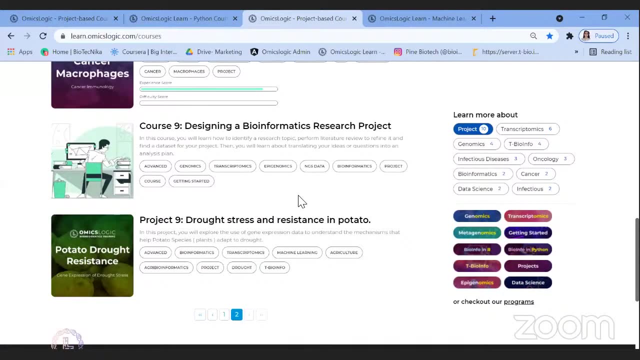 course and learn from it. and then the projects which i was talking about. you just have to click on the projects and you will get a list of sample projects that we have in which we have tried to analyze a lot of different sorts of fields, including the data sets, and then how you reach. 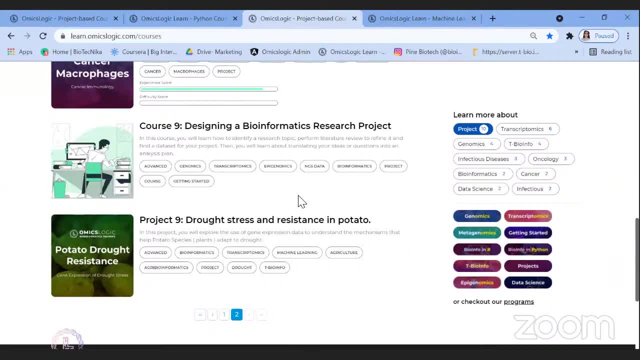 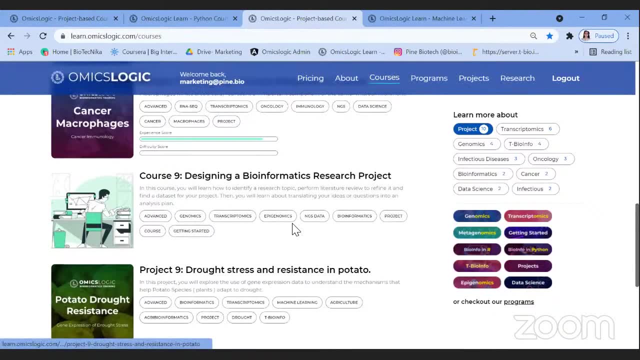 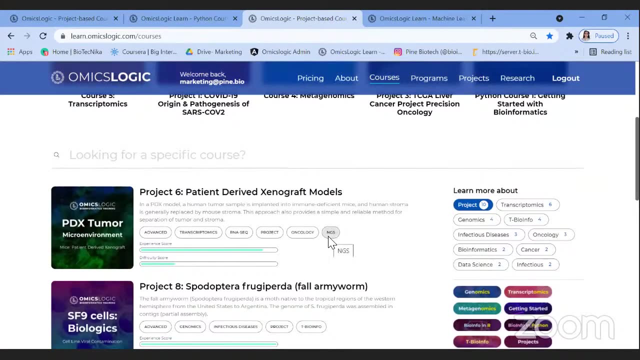 to the final analysis, how you run the python on the server, get your results, and then you, how you interpret your results to get biological, meaningful insights. and also those who feel that the program caused for them is not right, uh, right now, and or if they're very busy with their ongoing research. 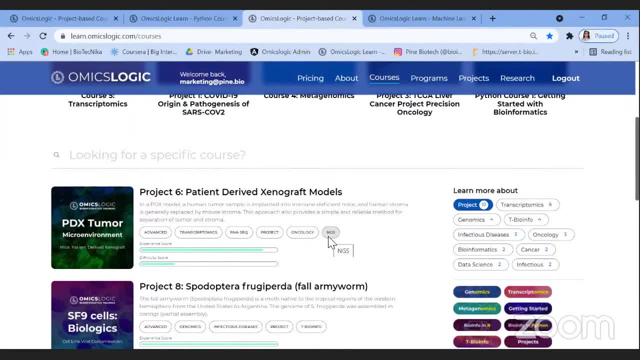 or their ongoing commitments to their institute. they can definitely go ahead with taking a basic subscription for the omics logic learn portal, where they would have the access to all the courses and all the projects that are present here under the courses tab on the learn portal. they can begin with going ahead. 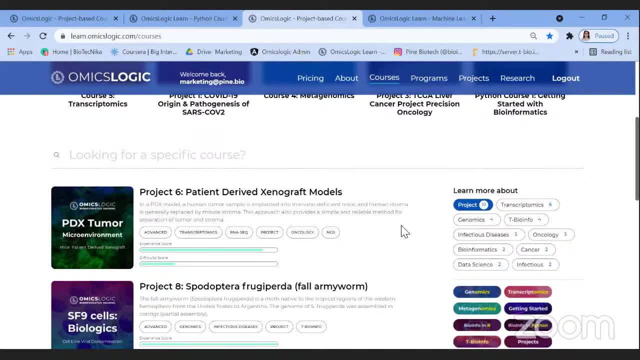 to have an understanding of these various courses and once they feel that they are now ready to go ahead with the specialization, maybe then they can definitely go ahead with taking the program enrollment and advance their knowledge of research. so we have few of the questions. uh, so no, no, mala, all these courses? uh, yes, they have one particular fee, that is a basic subscription. 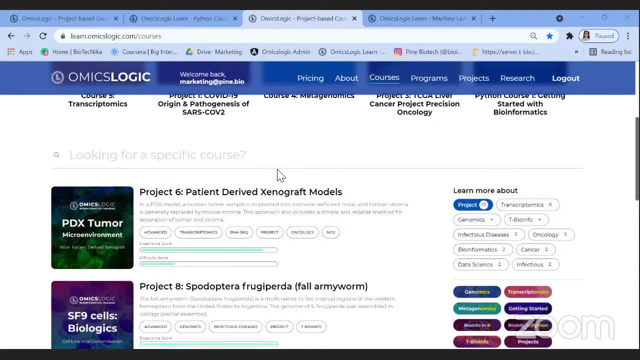 dollar 10, but you need not pay the fee individually for each and every course. the dollar 10 includes the access to all the courses that are present here under the course tab on the learn portal, to all the courses and all the projects that are here on the course under the courses tab on the. 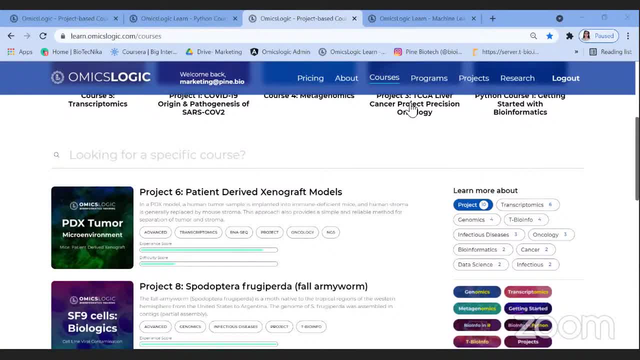 learn portal. sonam is asking: i'm exposed to python, art, omics, pipelines, machine deep learning in an intermediate expert level. how would this program help me? so i would like dr mohith to please uh help you, sonam, with this question. uh, over to you, dr mohith. 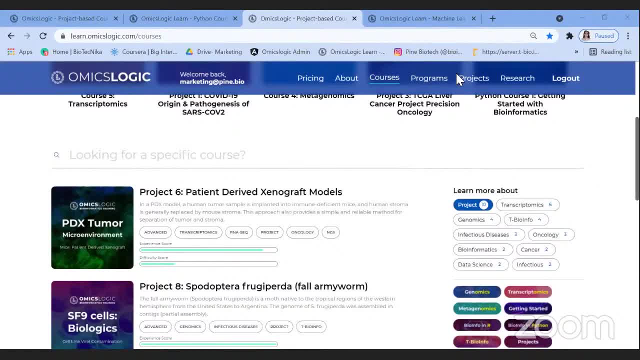 okay, so let me take the question itself. so, sonam, you are saying that you have already an intermediate or an expert level for uh, the various fields- python, art omics, and also uh omics, pipelines and machine and deep learning. i would like to ask you: have you implemented these different? 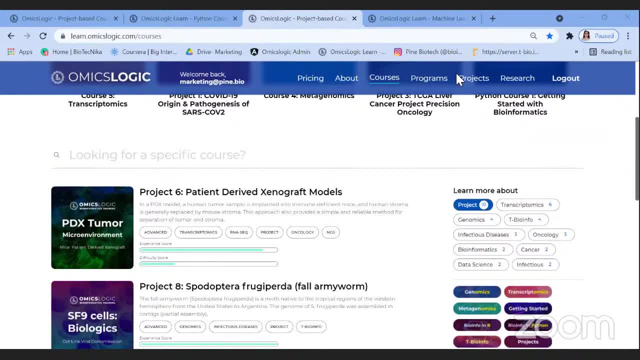 sorts of concepts to carry out your own individual research project or not? you can unmute yourself, maybe, and let me know that. and also, when you say that you have an intermediate or expert level for these different fields, is it specific to bioinformatics or to carry out the biomedical 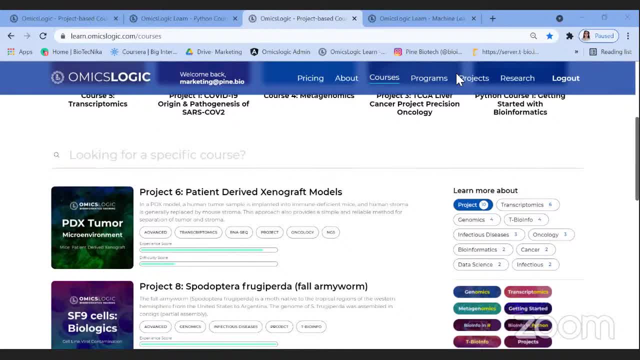 analysis or just in general. uh, you know about the basics and stuff. yes, olaq, you are uh, perfectly right. the 10 allows you to explore all the courses without the mentor support. so i'll tell you what exactly dollar 10 does. so let's say, if you go to 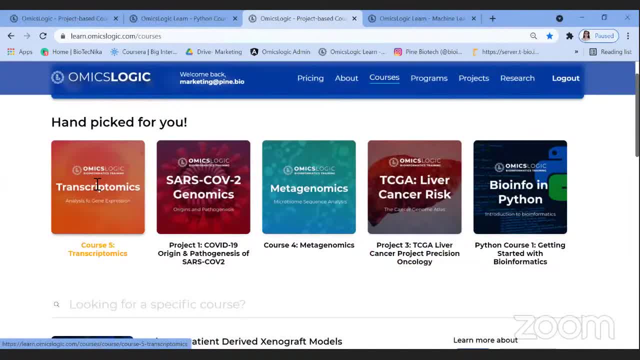 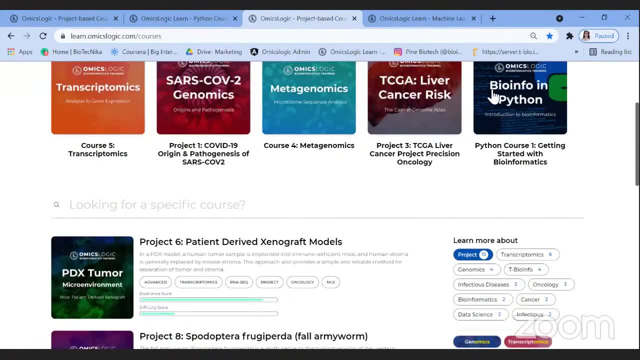 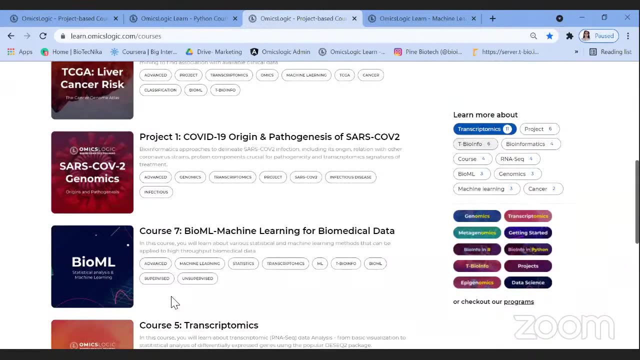 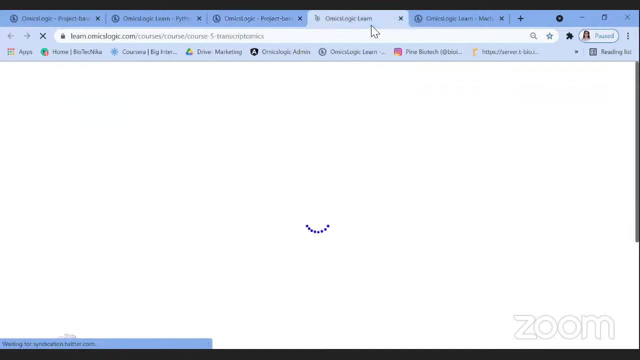 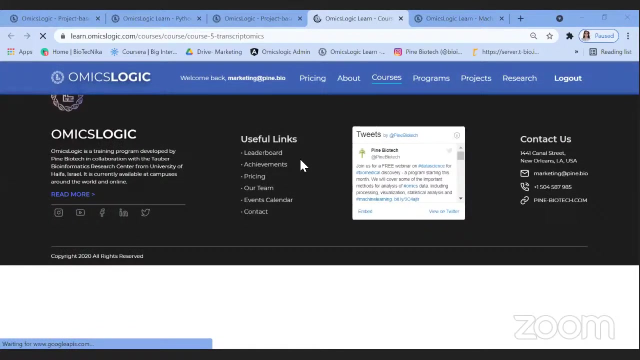 the transcriptomics course. uh, like whichever course you go to, you will find some start content on the course. just a second, i think i have a so net, yes, so when you go to the courses, uh tab, to whatever course you want to explore, you will find few of the lessons that unstart and many of them are start. so the ten. 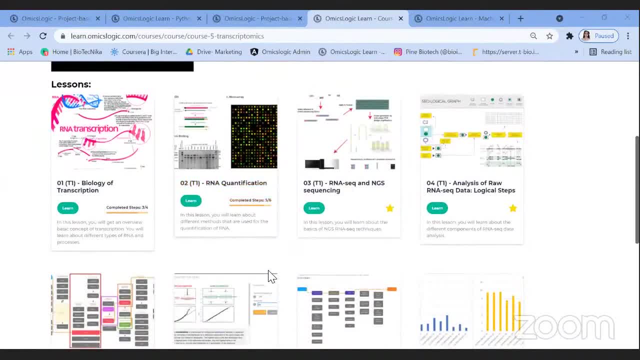 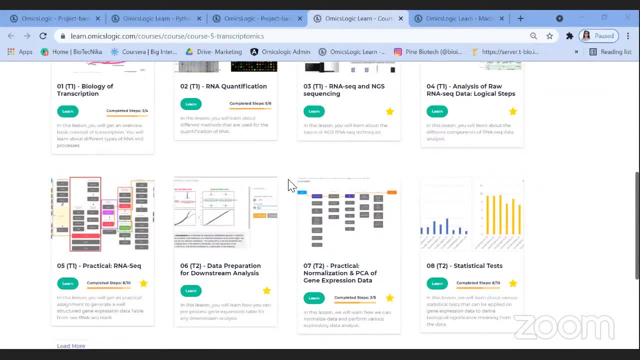 dollar basic subscription is basically to oriented the course and you will need some help creating them. and while the individual course pl asا looks as we saw the course think web page as well, so see all the course. let's know how they share with you about your information. um, do you want to do a lot of that and check out the links by ahammah? whom? of what learnings and things? staff. 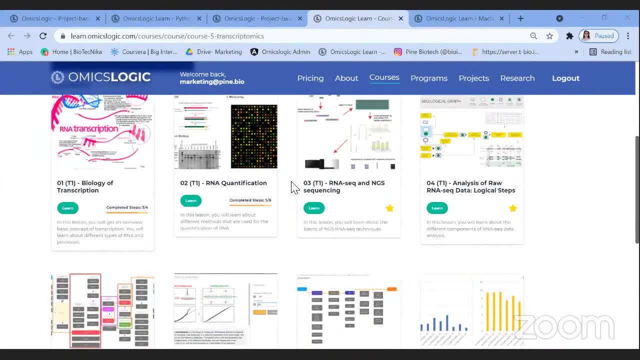 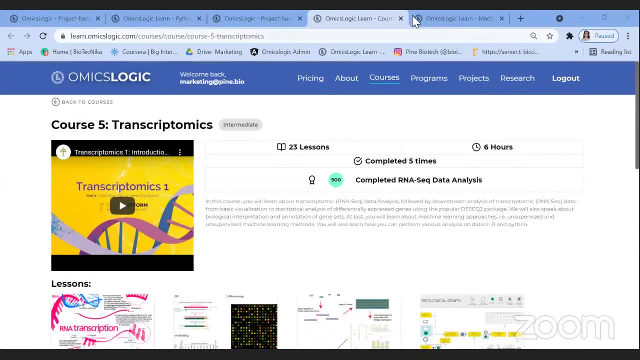 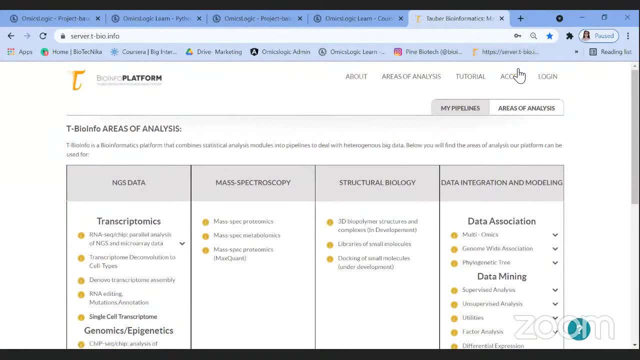 to get you the access to all the start content that is there- uh, in the courses on the uh, on the logic learn portal, and to talk about the server where you are going to uh carry out the pipelines and run the analysis and then get your results and try learn to interpret them for the server. 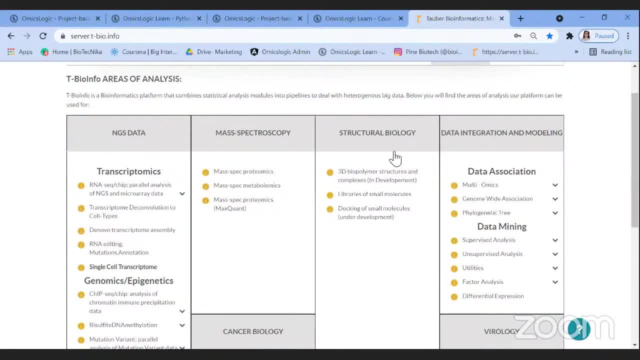 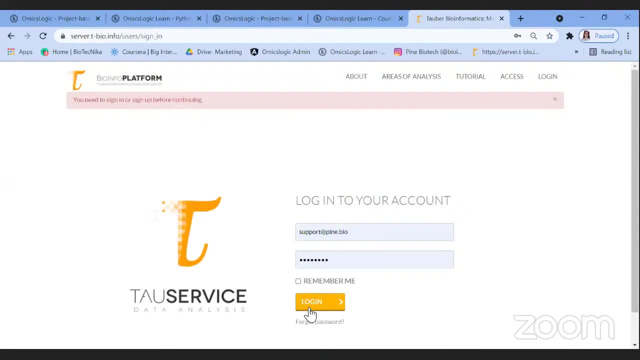 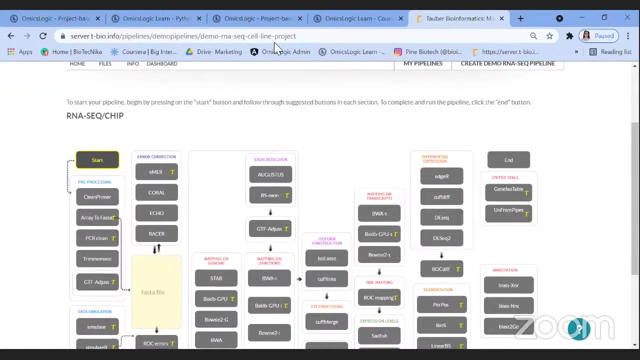 for the 10 basic subscription, you would just get the access to few of the demo pipelines here. so you already have the demo pipelines where the data set has already been uh uploaded and you just have to run the pipeline just to learn uh how the pipeline could be run using the different. 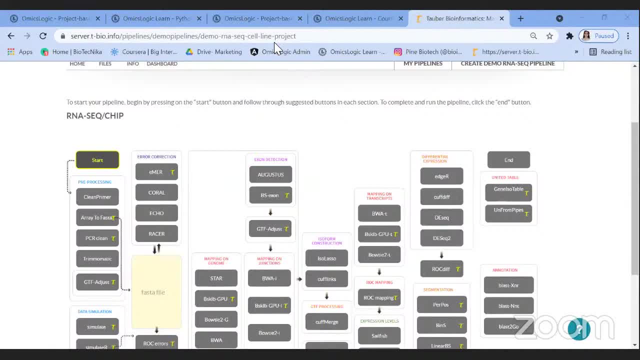 algorithms and what these algorithms are actually doing. uh, at the back end, the knowledge to that would be given in the courses, and then you will get the result from this one. uh, this is the pipeline that is being created. so you can get the pipeline and you can then analyze. 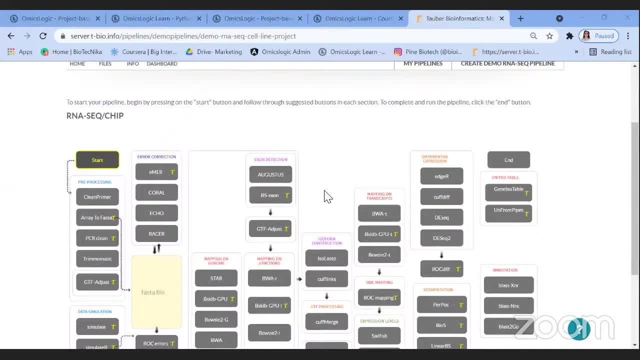 the result and interpret your results accordingly. and how to interpret your results have been very well explained in the courses as well. so that is why taking the courses to run the pipeline and actually learn how the pipeline has to be run and how you interpret the results is important. so let's 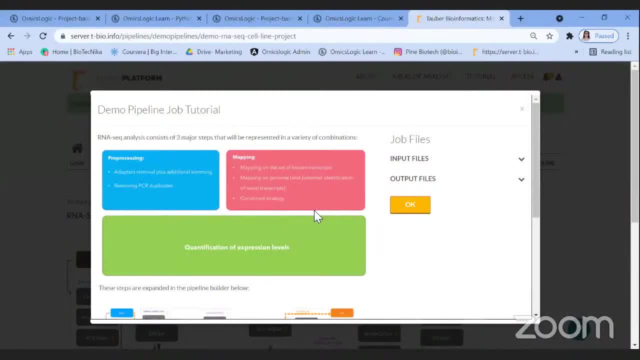 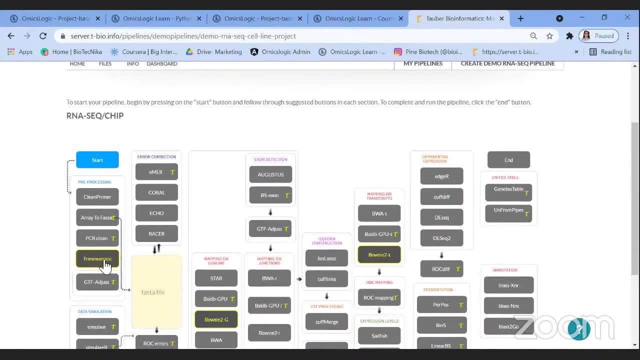 do just one pipeline real quick. so if you click on start, the data has already been uploaded you'll are trying to do at the back end. so once you click on start, the next step is trimomatic, which gets highlighted right. so you have to click on trimomatic and after that the next, the next. 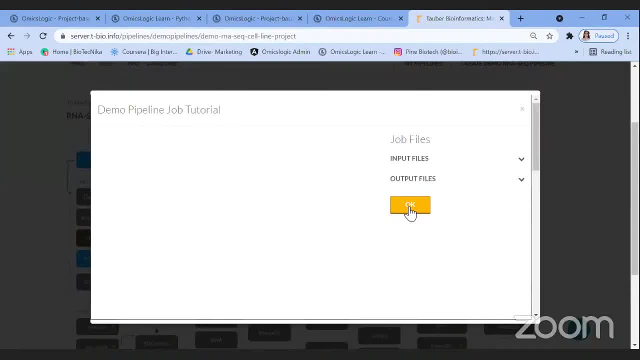 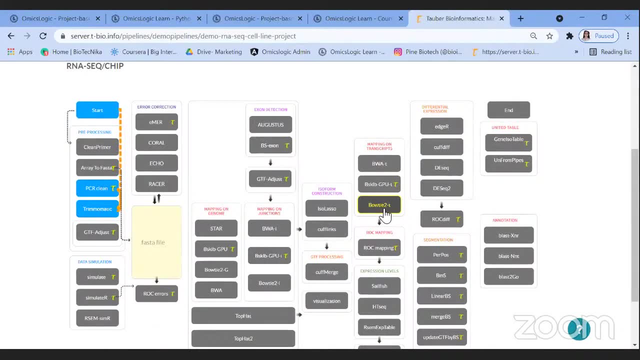 session that gets highlighted is pcr clean. now, once you click on pcr clean, then the next step would be highlighted. that is bounty 2d, the next algorithm. now to understand what is trimomatic, why is it required? what is pcr clean? again, everything is mentioned in the courses itself. 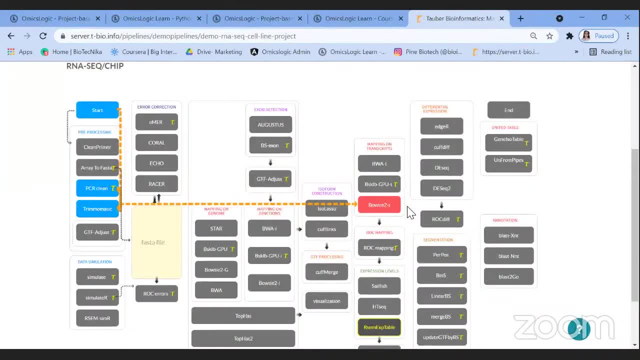 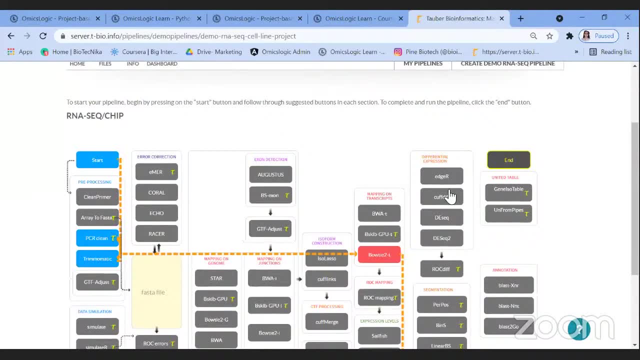 so this is the way how you can run your pipelines and get the result, and then you have to click on the rsm expression table just to get your expression table and simply end the pipeline. so you see how easy it is, that you could quickly run a pipeline and then you would get your results. 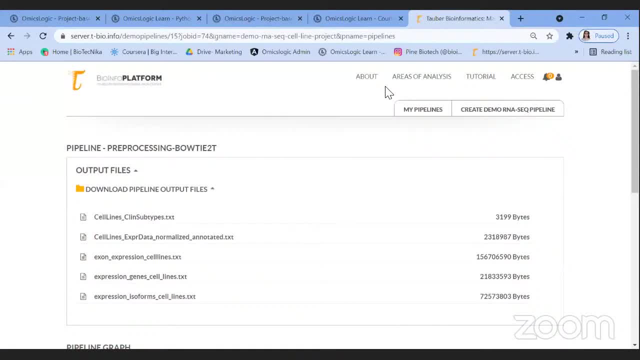 and analyze them accordingly. any further questions? okay, so now i'm dropping in my mail id in the chat box. it's marketing at the refinedbio and you can reach out dr mohit at mohut at the refinedbio with any queries or issues uh you face and you would like to proceed with, and uh also let me.